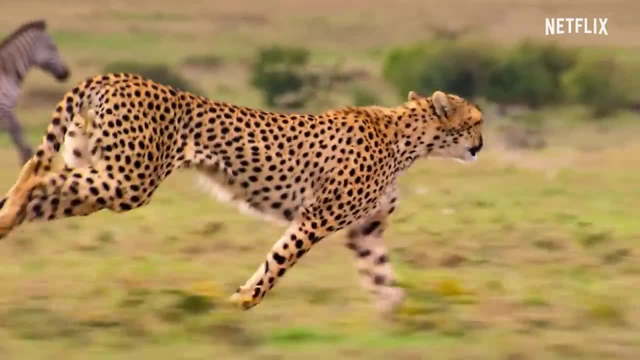 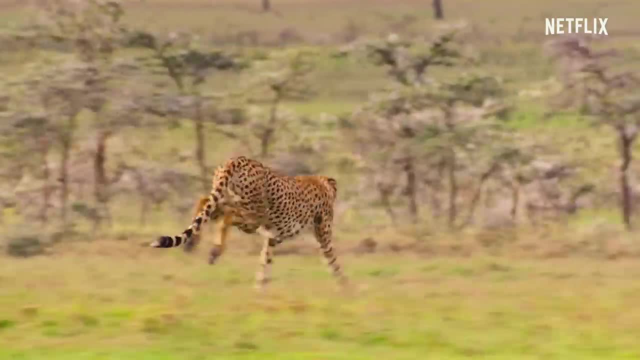 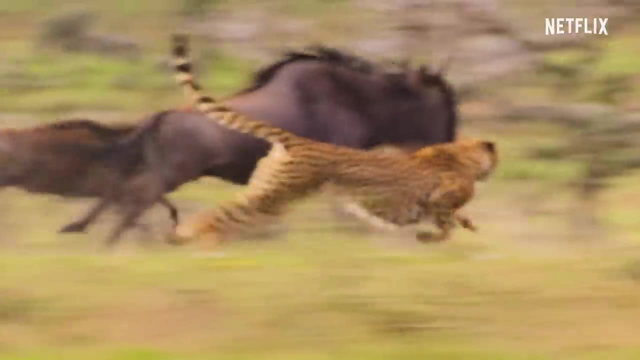 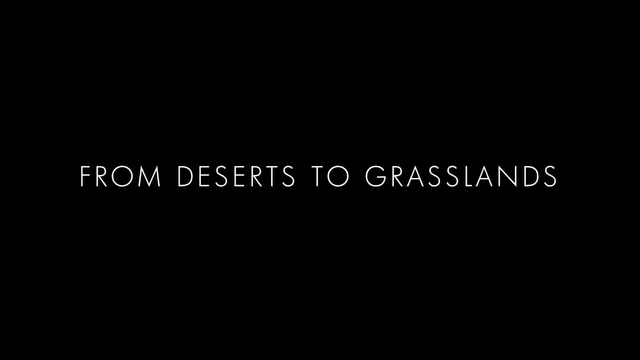 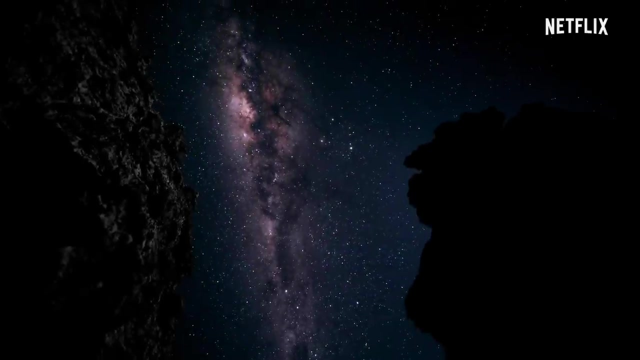 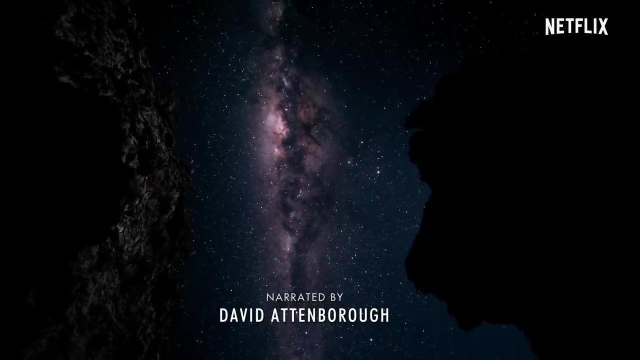 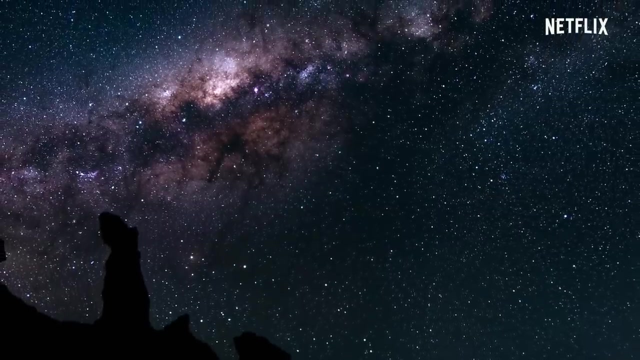 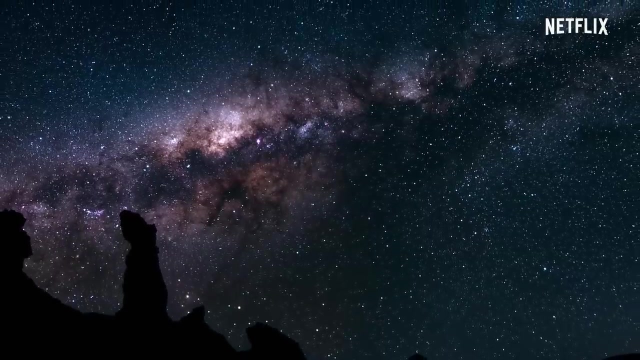 Our planet will very quickly see and feel all of its own magic一个 birth. Our planet will start built by nature. Hey, hey, hey, hey, hey, hey, hey. A fifth of the land on our planet is covered by desert. 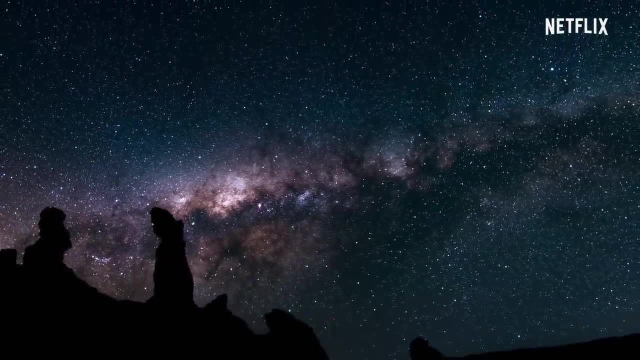 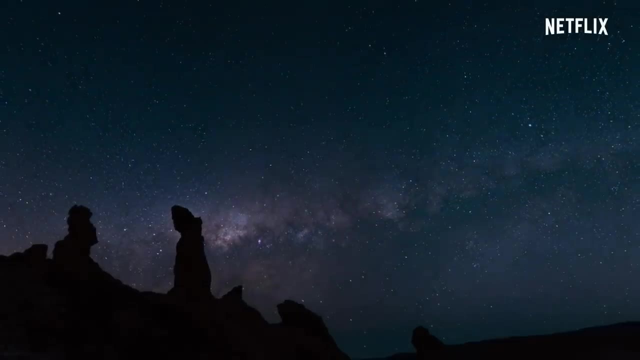 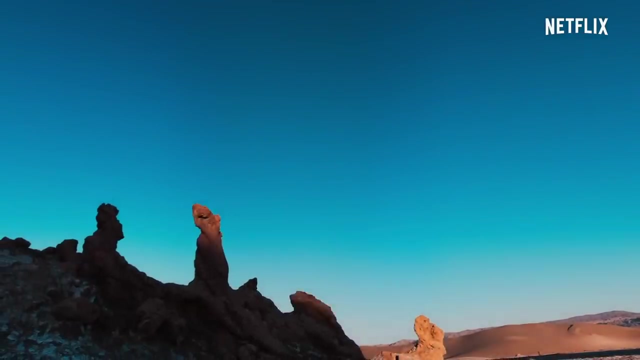 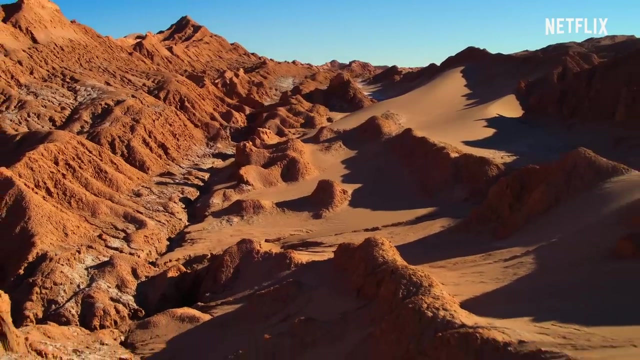 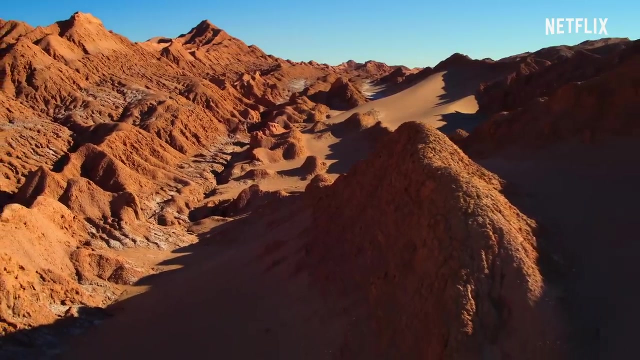 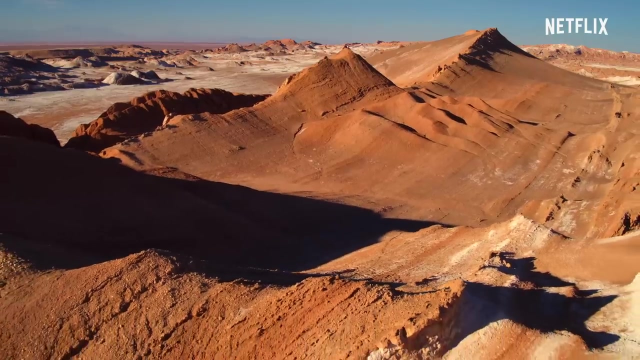 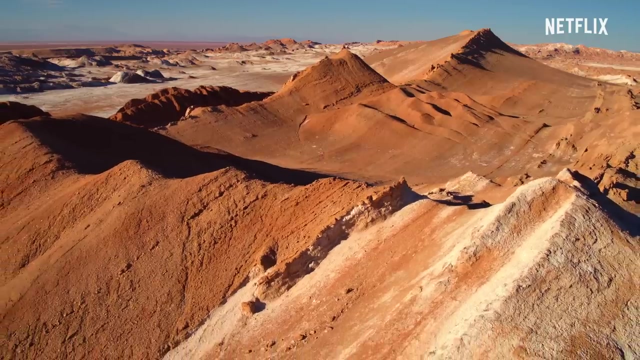 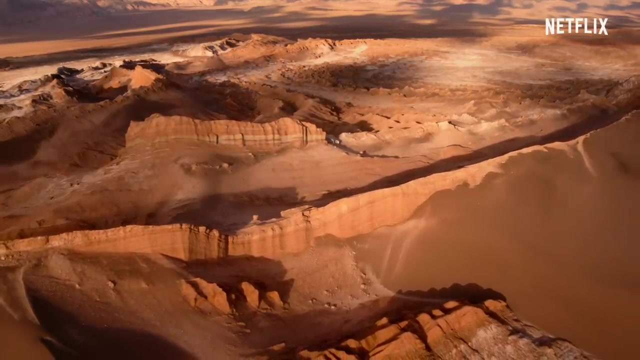 The driest of all is the Atacama in South America. There are places here where rain, but rain has never been recorded. Deserts may appear to be barren and empty, but they are of crucial importance to life For those that can overcome their challenges. 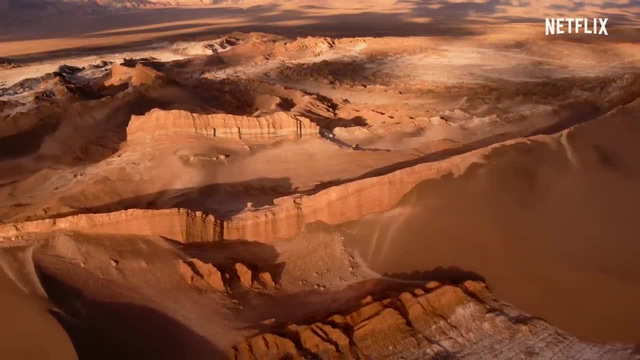 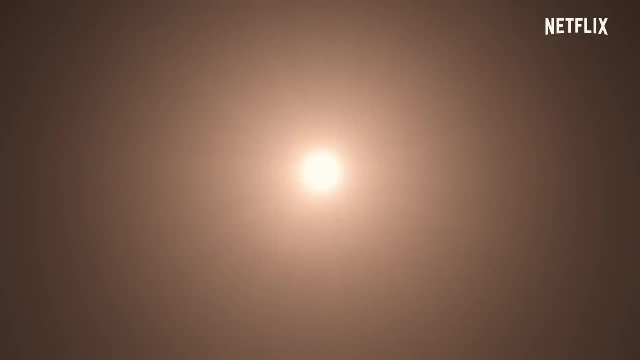 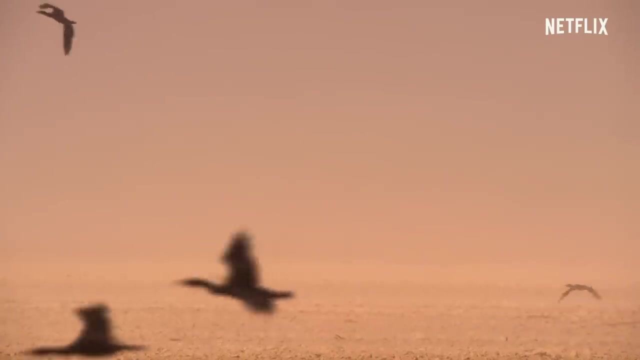 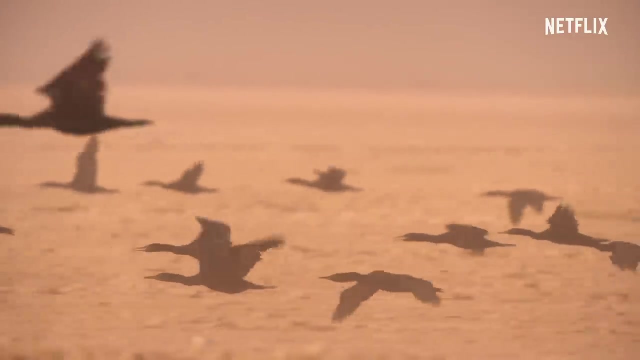 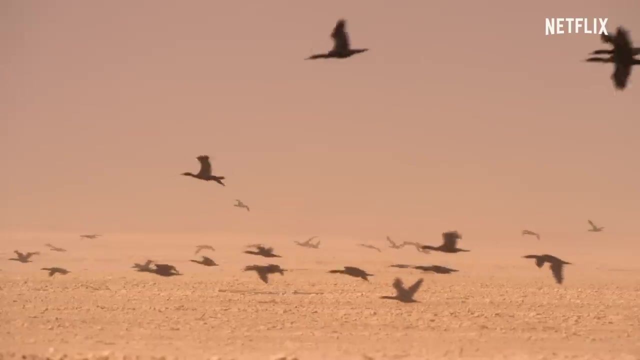 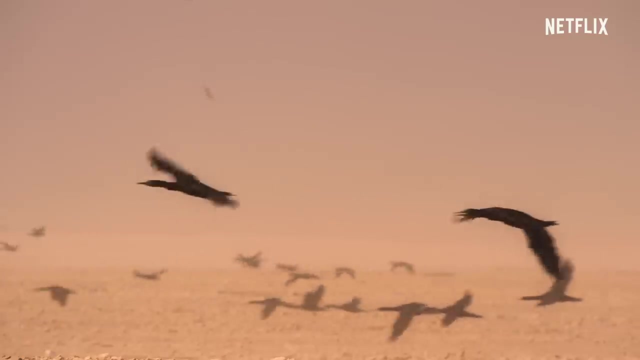 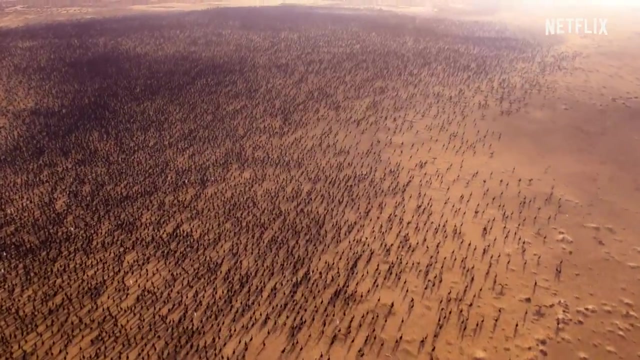 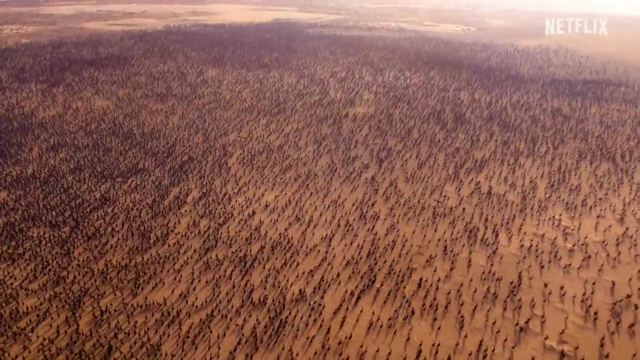 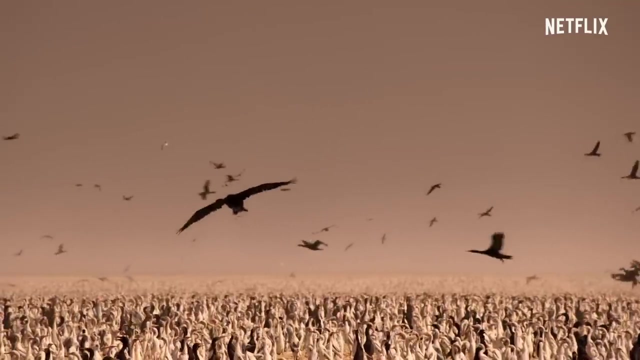 they provide a vital refuge: A Socotran cormorant emerging from a dust storm in the Arabian Desert. It is the very emptiness of this landscape that has brought them here, And they have come in immense numbers, 50,000 of them, a quarter of the total population. 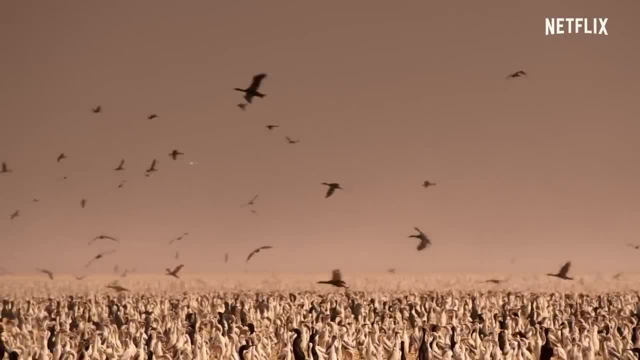 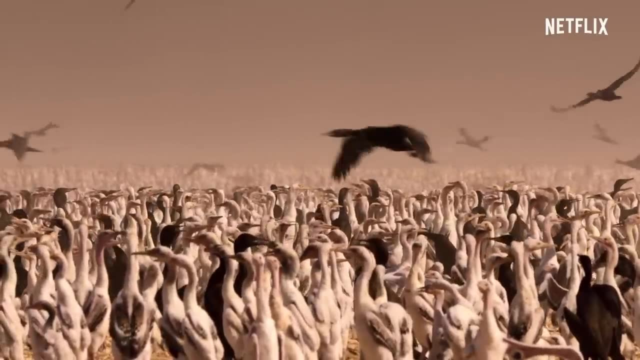 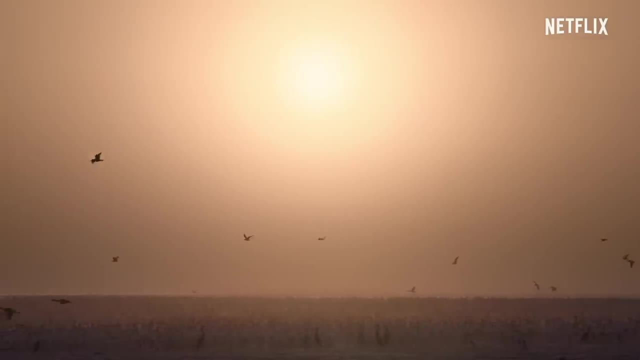 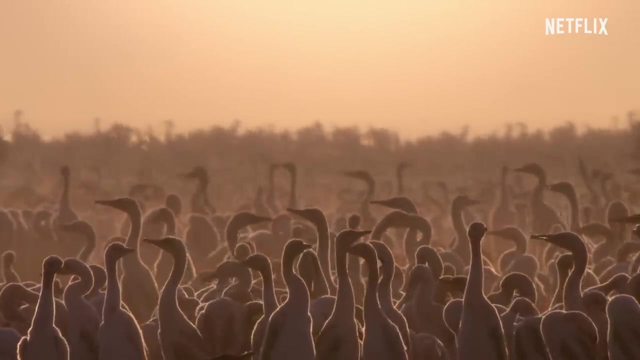 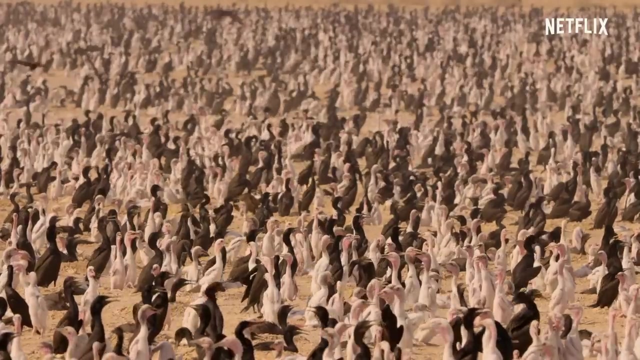 They have come because here they are. They have come because here they are And here they can breed undisturbed. But nesting in a desert is difficult. Temperatures can reach 40 degrees Celsius. Yet both the adults and their white chicks are ready for this challenge. 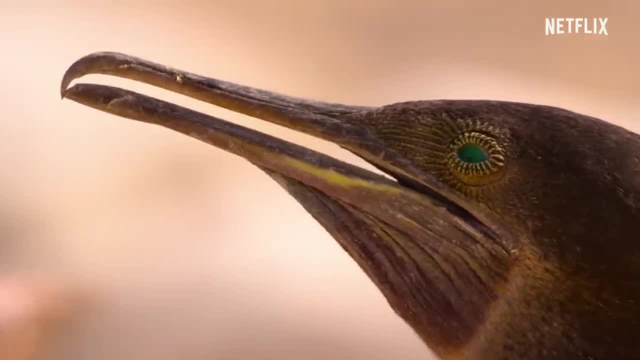 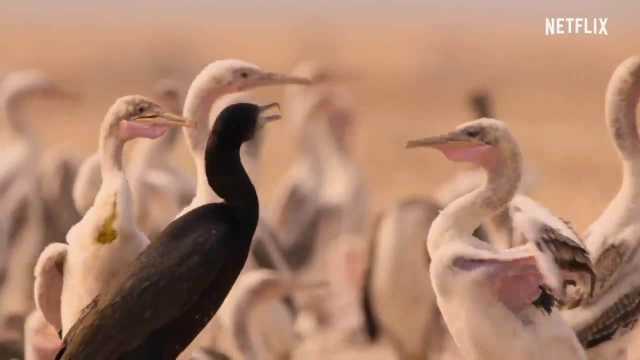 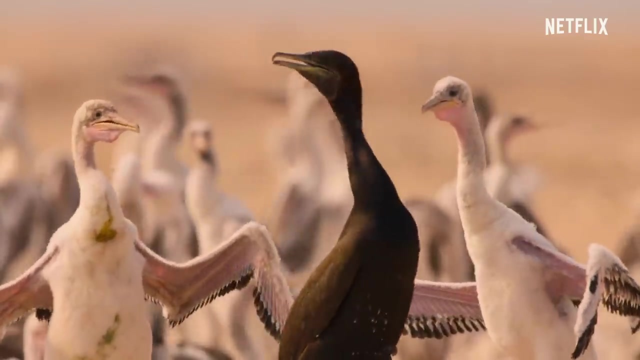 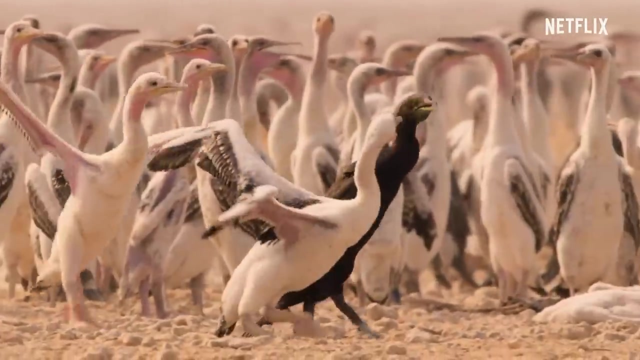 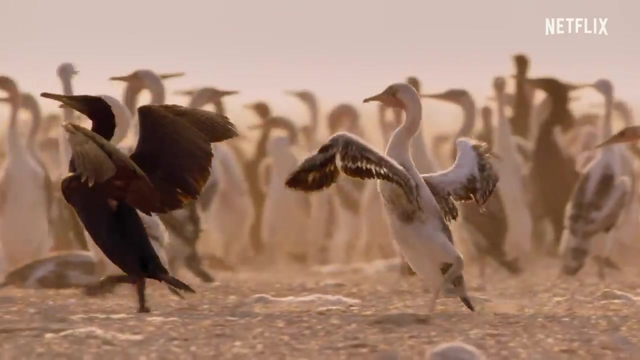 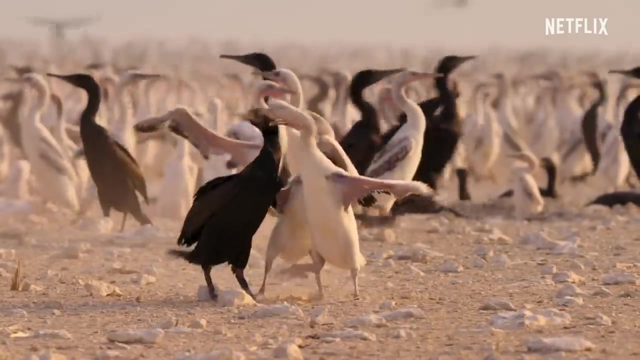 They cool themselves by panting. Any adult that appears to have food in its crop is mobbed, And they are not alone. An adult will only give food to its own chick, Which must be here somewhere. The chicks chase an adult out into the desert. 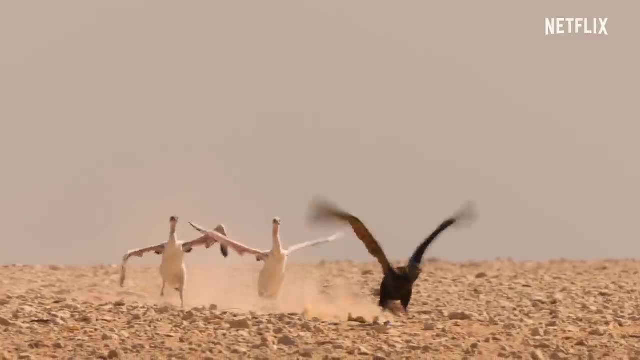 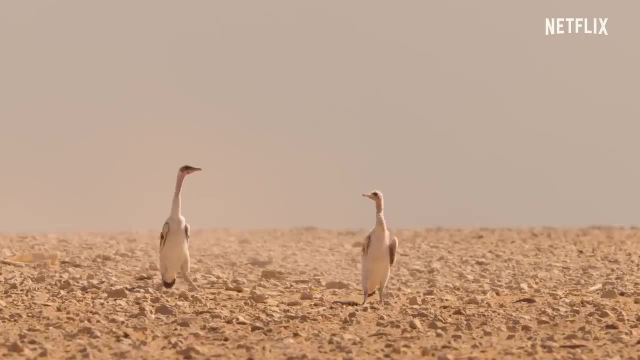 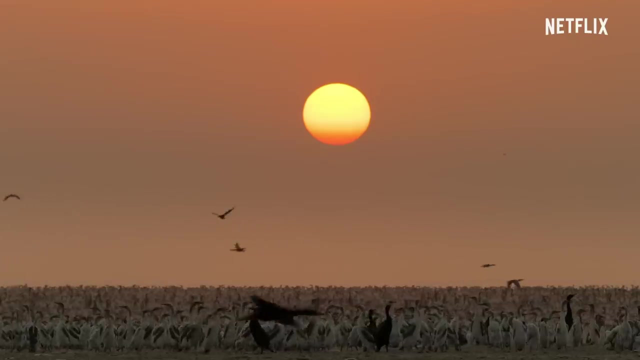 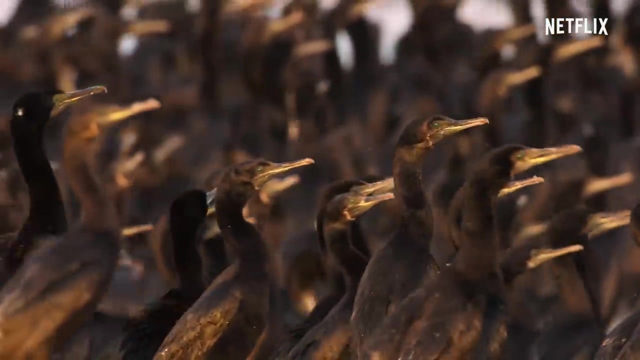 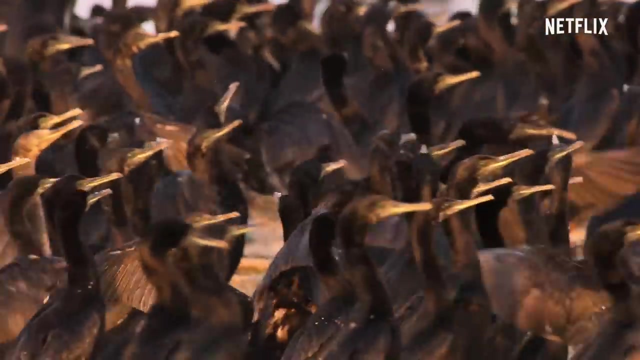 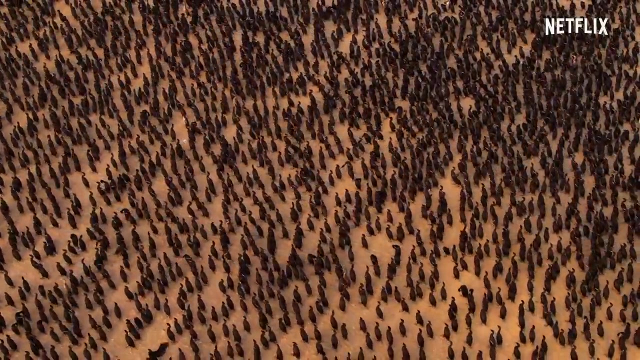 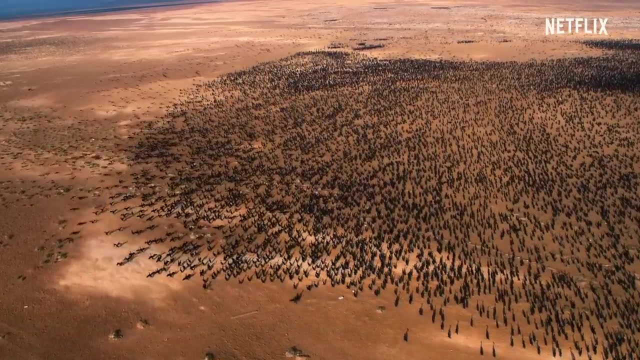 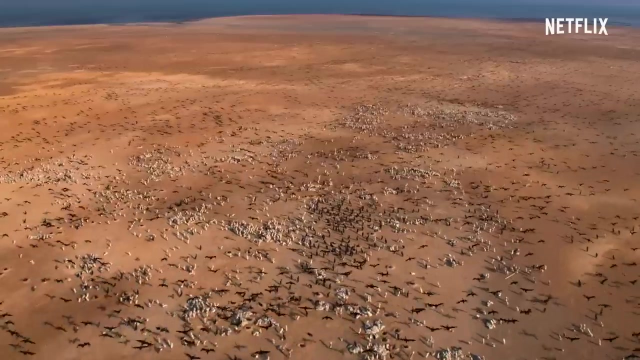 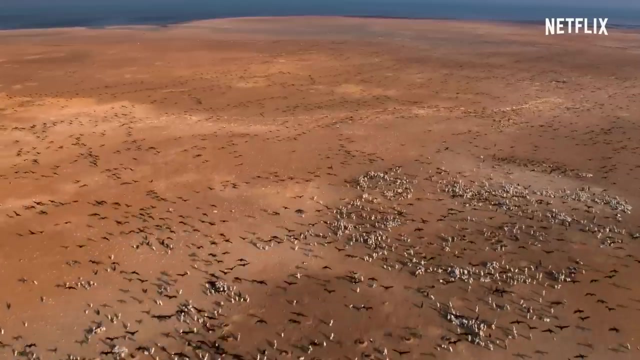 No luck, No luck. Now they must get back quickly to the safety of the colony. This desert provides the cormorants with more than just a secure refuge. Every morning, a mass movement begins. It's the rush hour. It's the rush hour. 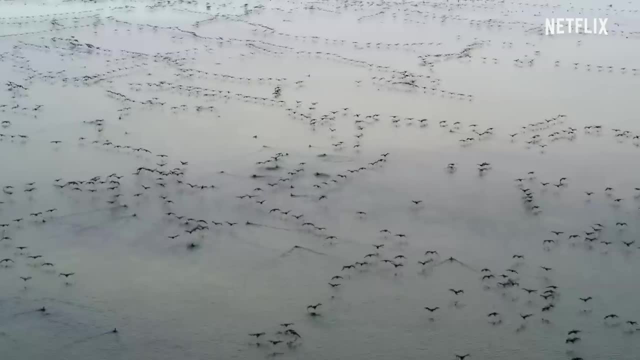 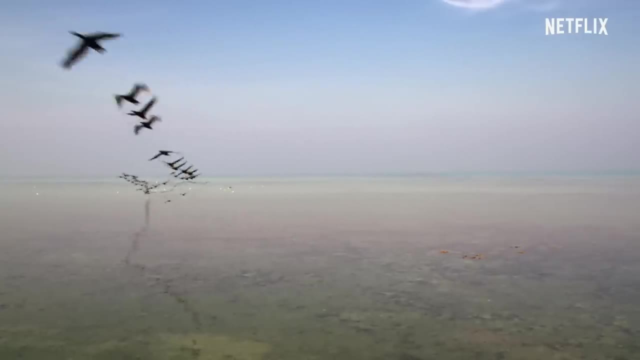 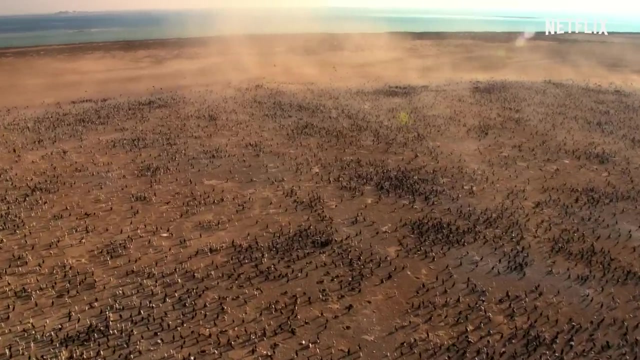 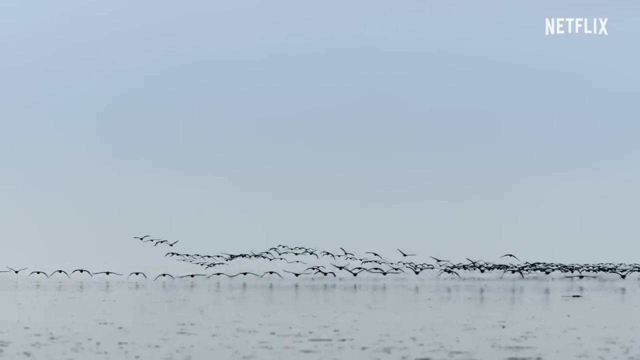 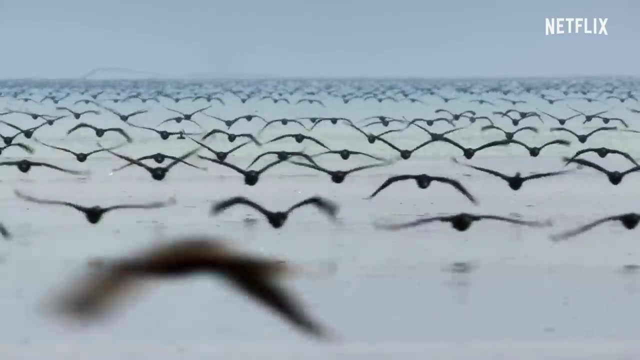 A shallow arm of the sea right beside the colony is full of food. This richness comes from the desert itself. Dust blown from the land contains nutrients that fertilise the surrounding waters, So it is the desert itself that enriches the sea. 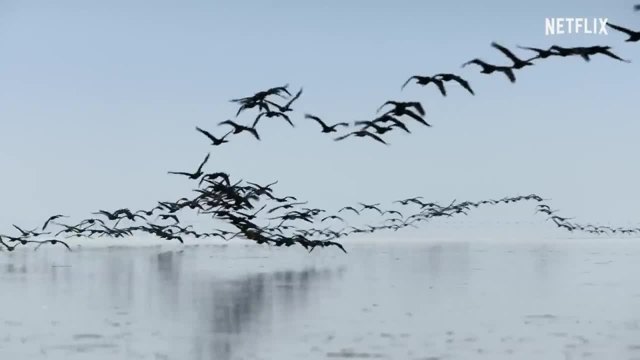 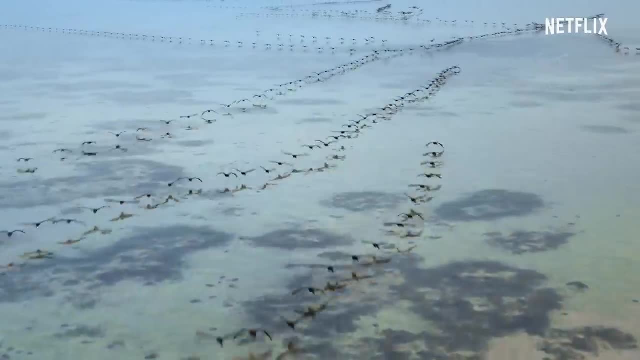 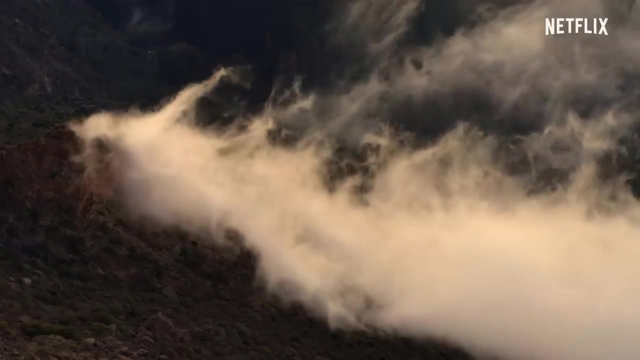 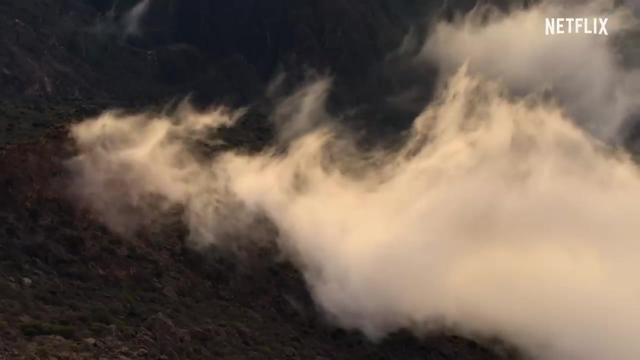 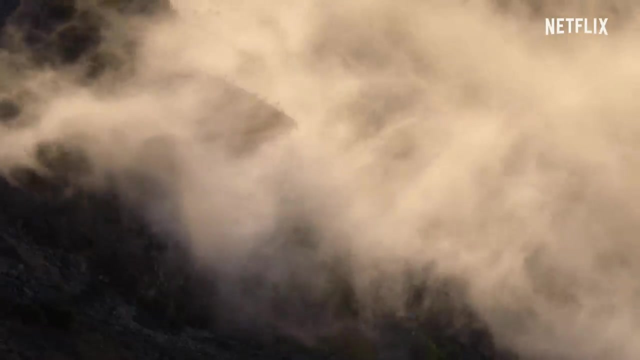 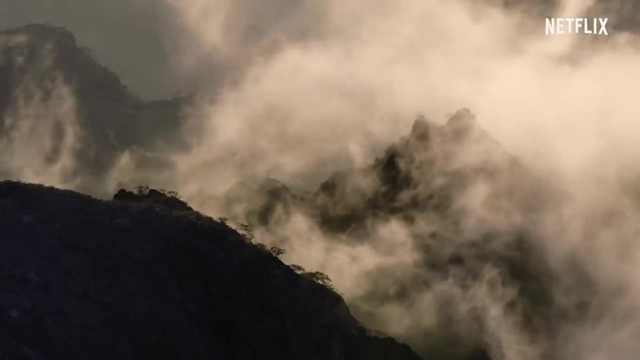 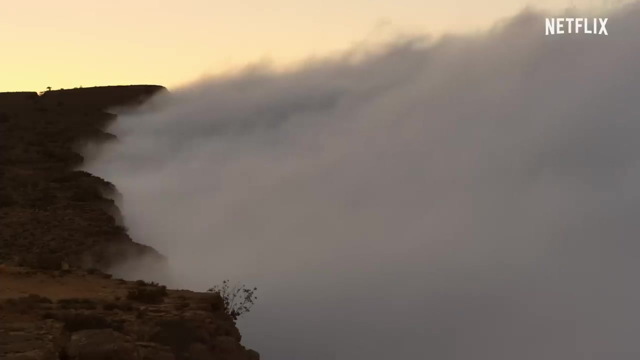 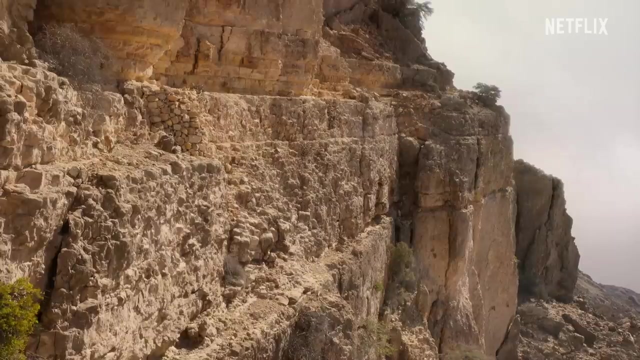 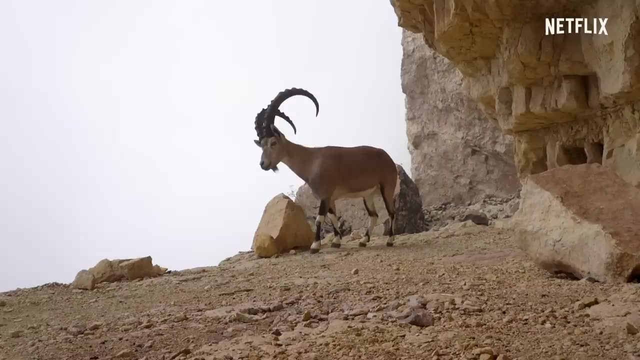 ρι In hammaman. during the summer monsoon, thogs roll in from the sea over the Dhofar Mountains. The mists bring just enough moisture to sustain a little vegetation, And this sparse greenery becomes a focus for life. It's a place where you can find a lot of beautiful nature. 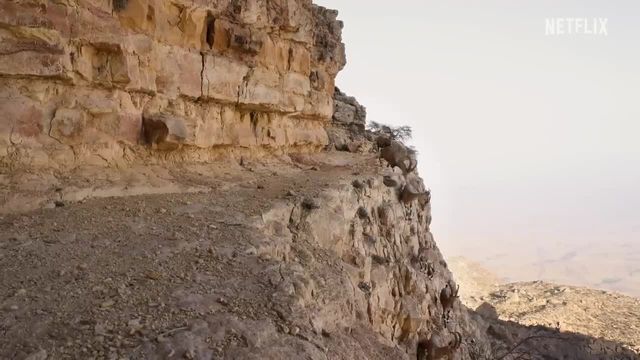 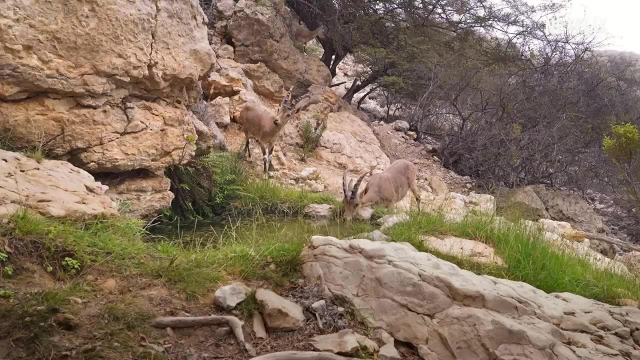 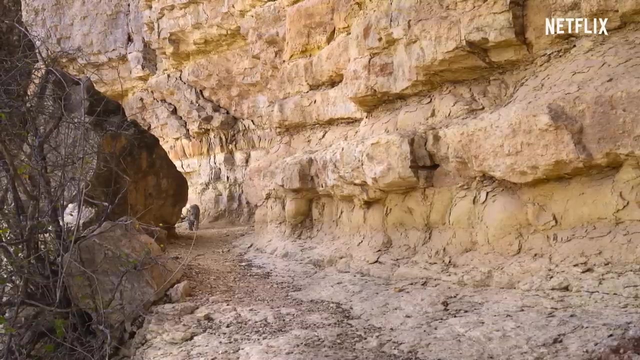 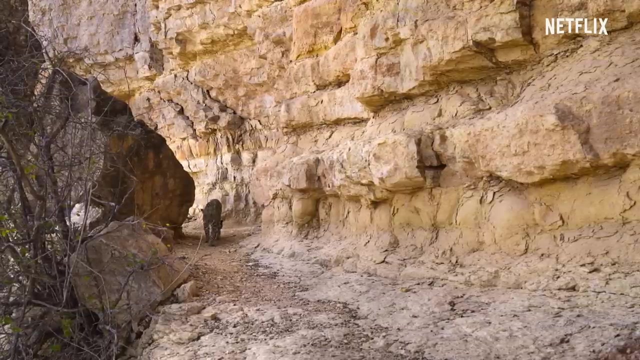 It's a place where you can find a lot of beautiful nature. Ibex must cross the near-vertical cliffs to reach one of the few springs, But they're nervous, And with good reason. An Arabian leopard- One of less than 200 that survive in the wild. 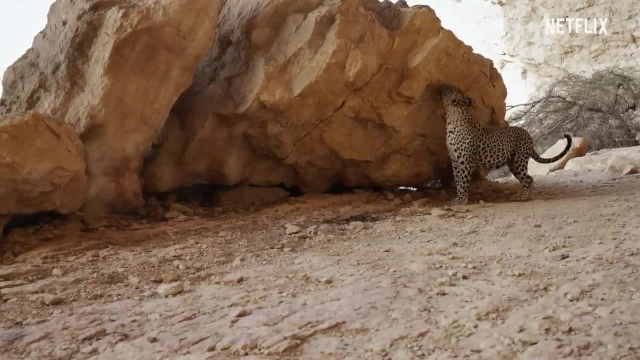 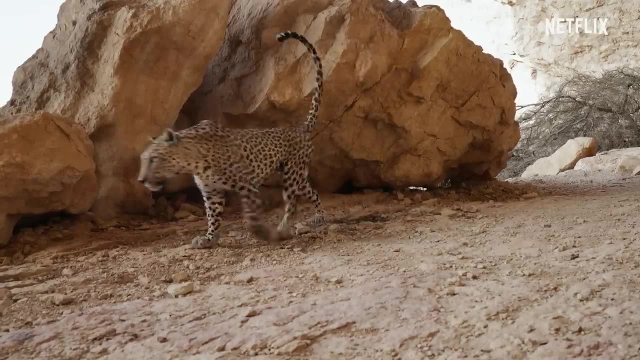 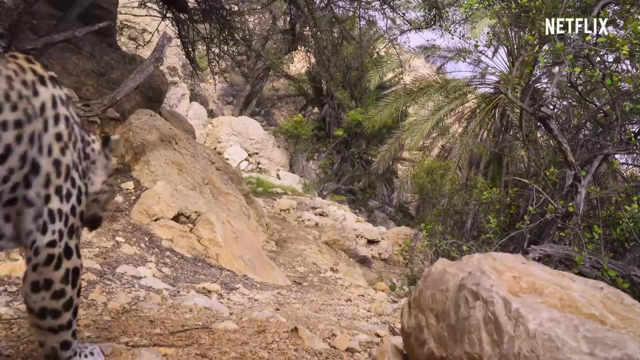 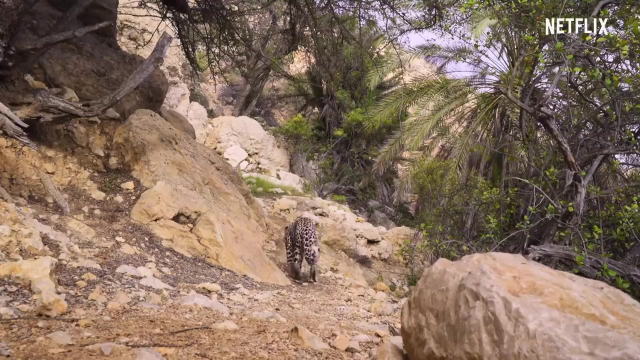 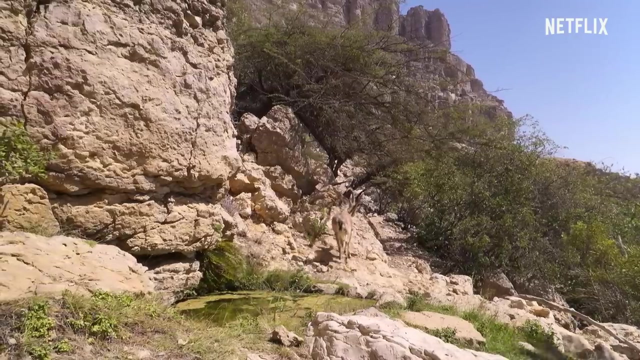 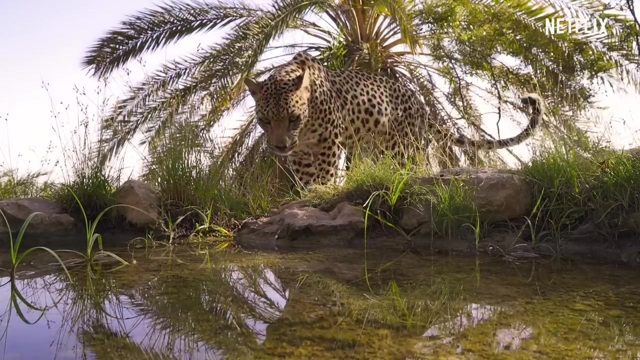 This male's territory extends over 350 square kilometers of high mountains and deep wadis. The southern edge of the Arabian Peninsula is one of the few places left where there is enough prey to sustain a population of these leopards, But even so there are probably less than 60 individuals. 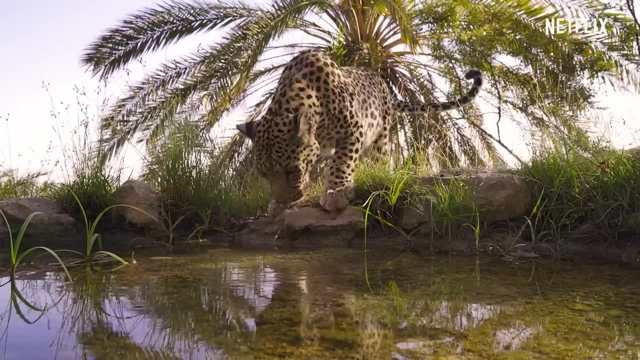 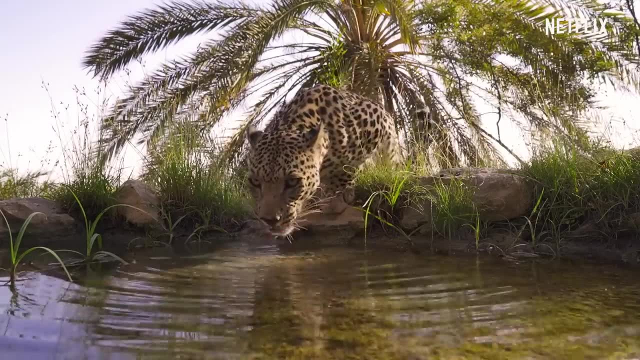 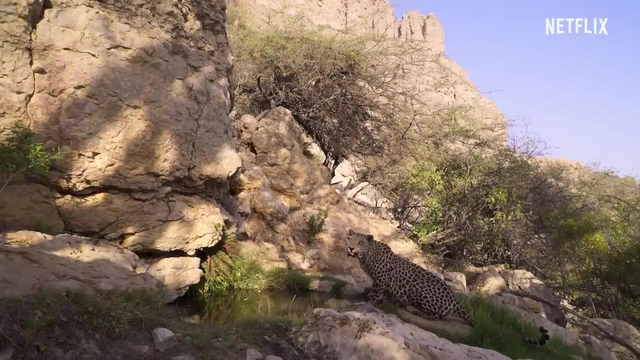 in over 15,000 square kilometers. The Arabian Peninsula is a beautiful place where you can find a lot of beautiful nature, But these leopards have always been rare, But now conflict with people is causing their numbers to decline still further. 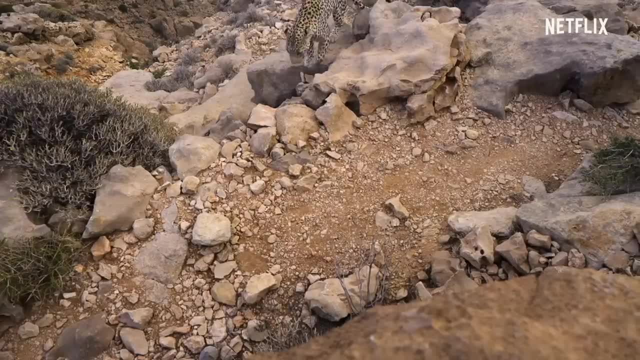 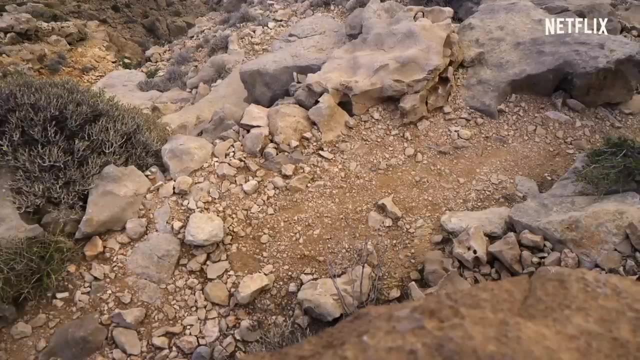 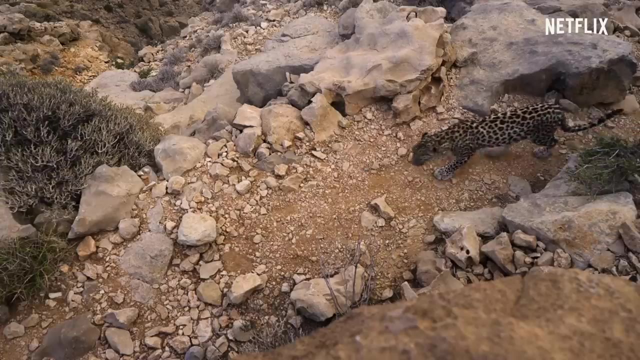 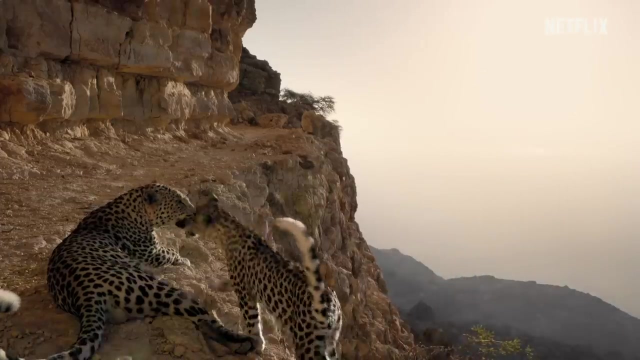 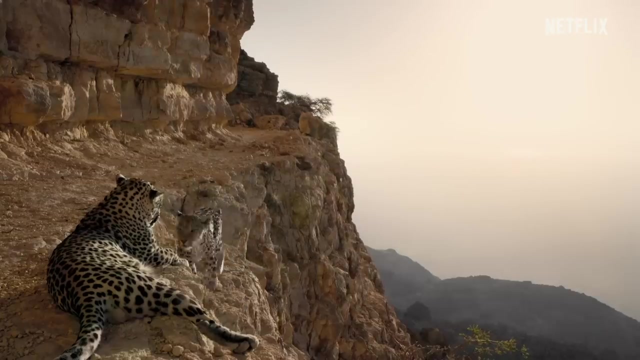 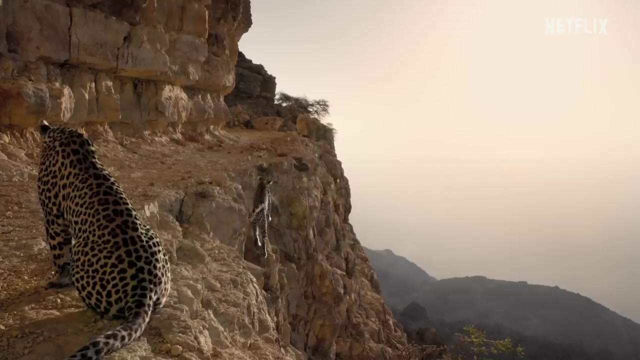 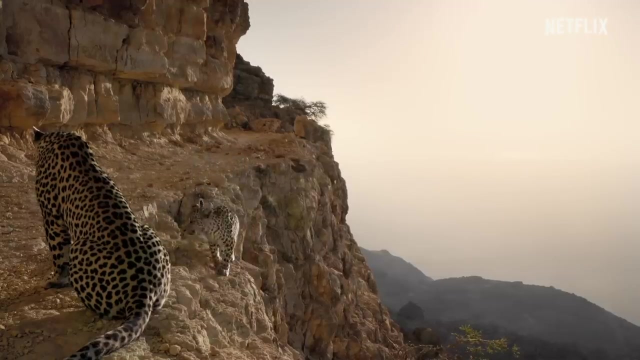 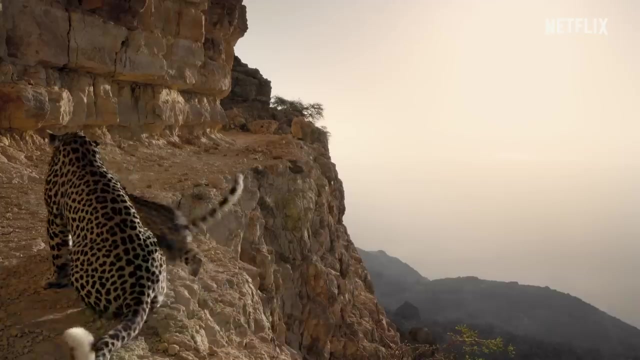 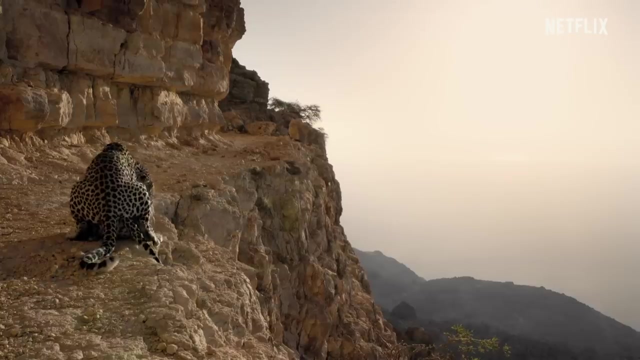 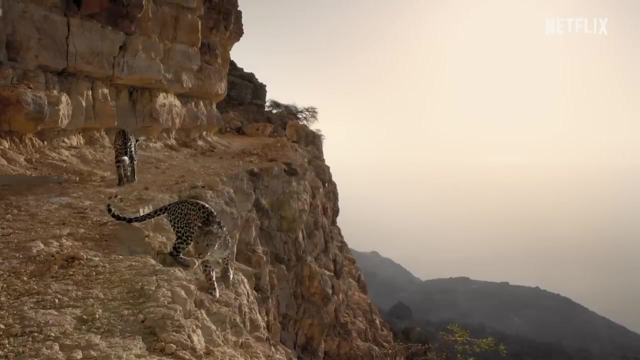 Few leopards are left. So what our hidden cameras now capture verges on the miraculous. A female leopard, And she is tracking a male. I hold it by my finger. Such meetings are becoming increasingly rare. This briefest of unions may ensure the short-term future for these leopards. 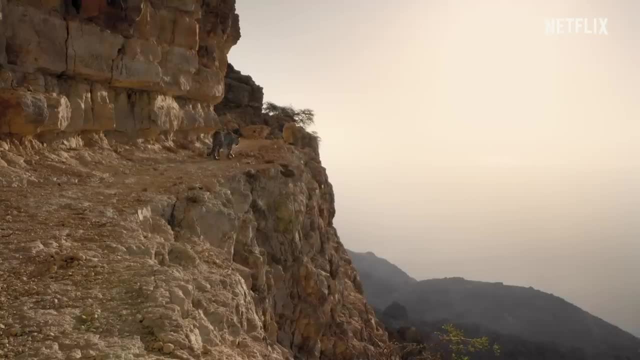 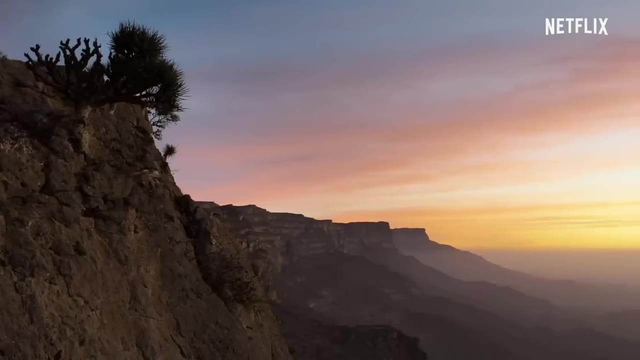 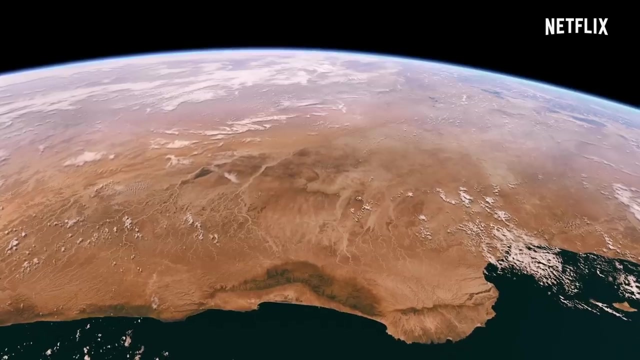 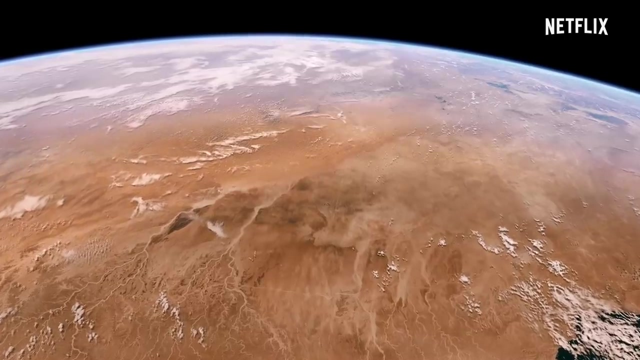 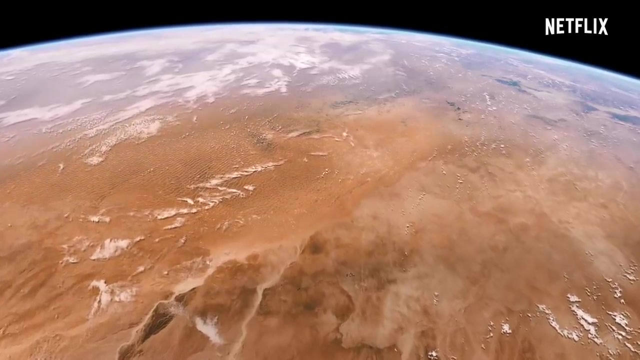 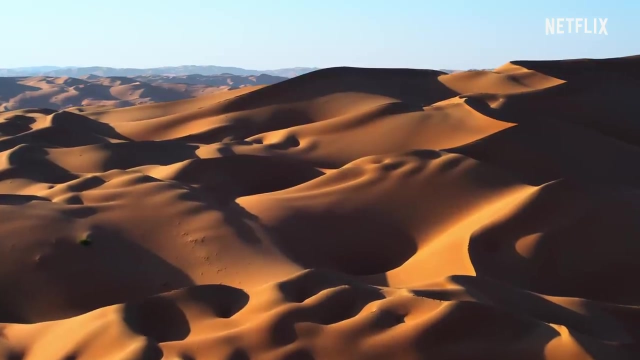 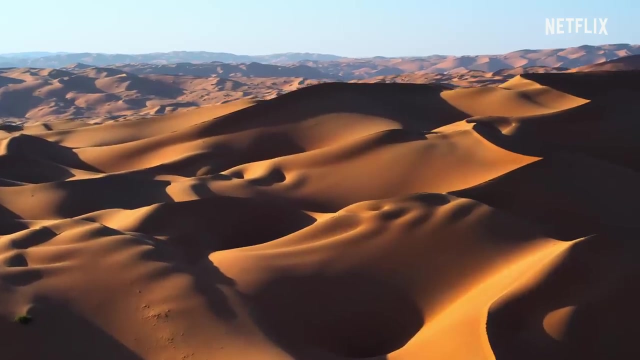 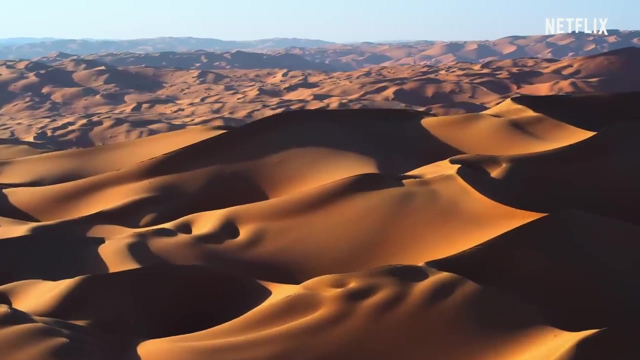 But in the longer term, their fate will depend on their territory being protected. To the north of the Dhofar Mountains lies a place of almost unimaginable emptiness: The Rub al-Khali, The empty quarter. The very name of the place resonates with the romance of these desert lands. 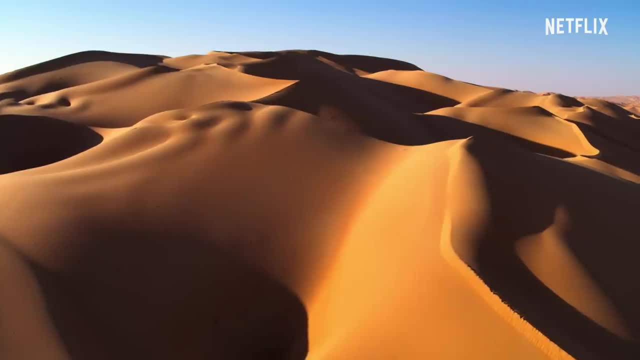 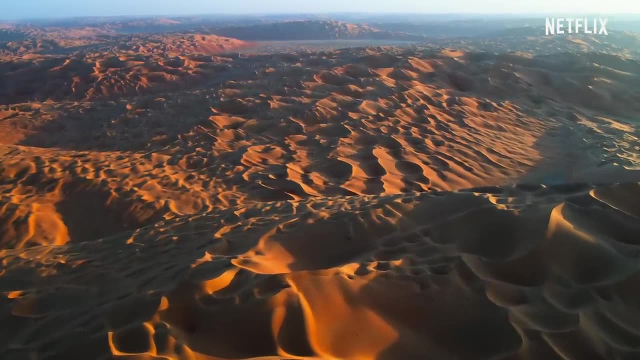 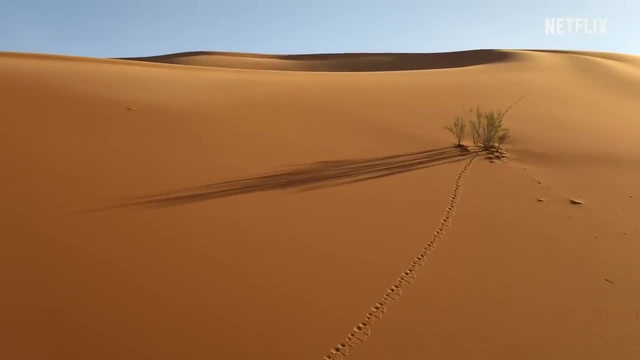 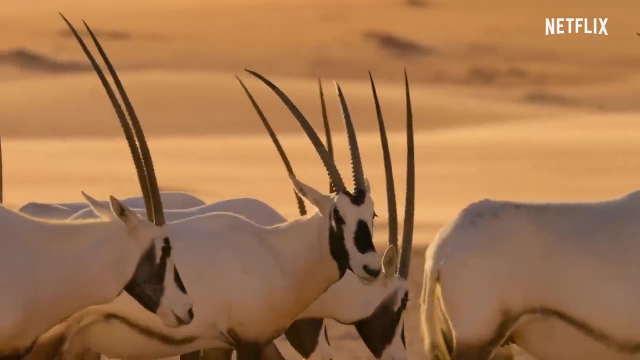 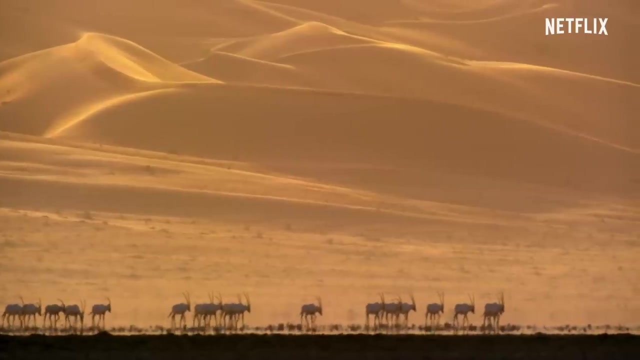 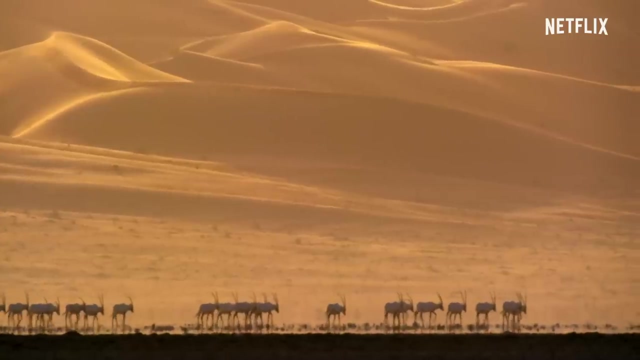 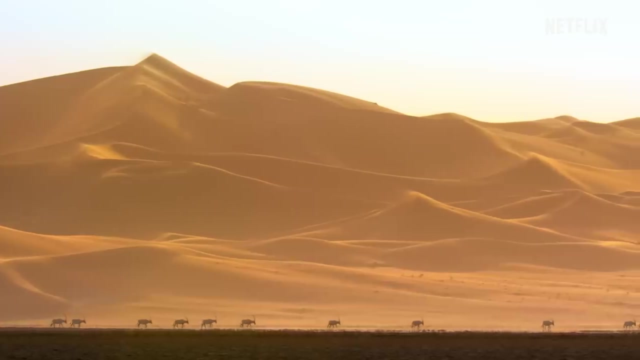 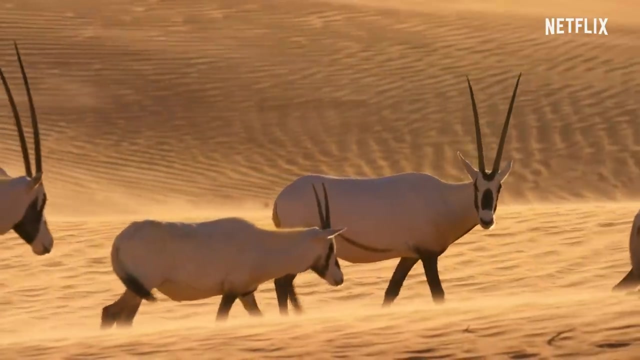 Only the greatest desert specialists can survive here. Arabian Oryx. Their ranges are vast, extending for over 3,000 square kilometers. This is one of their last refuges. Once hunted close to extinction, they have now reclaimed their ancestral territory. 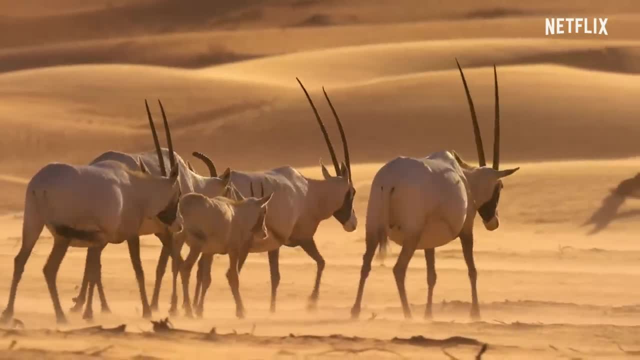 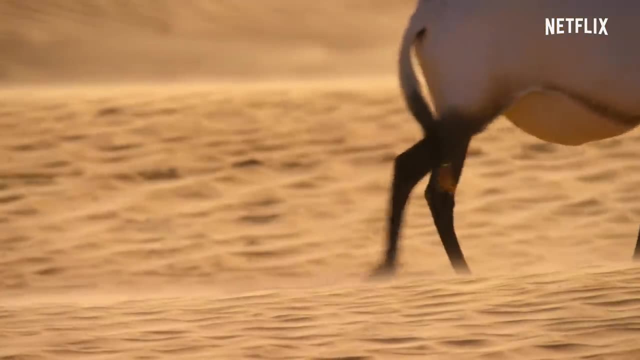 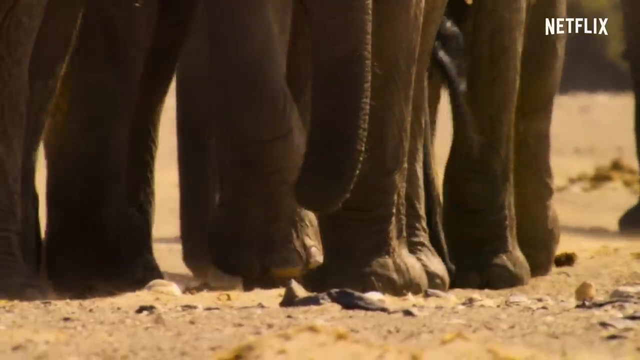 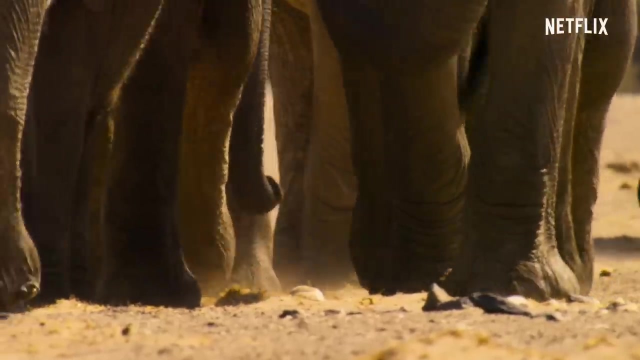 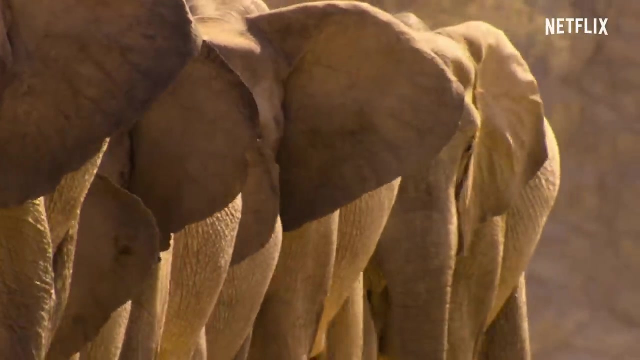 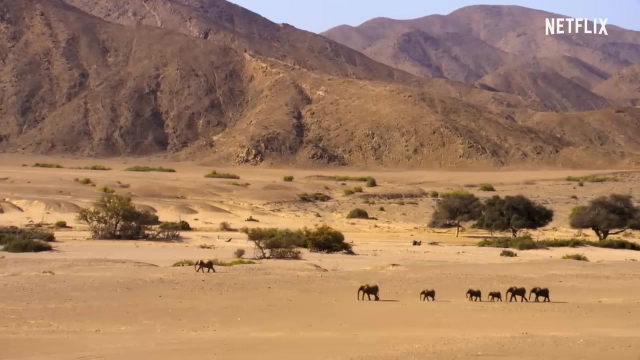 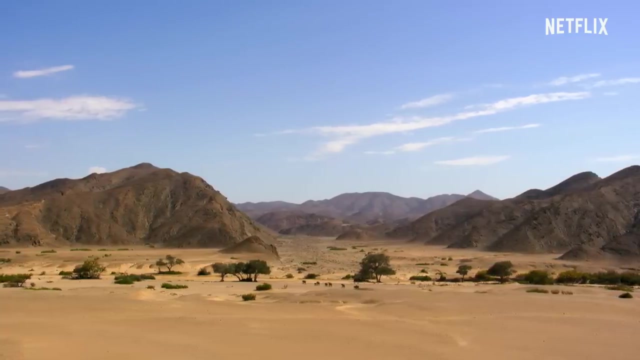 With the help of conservationists, they have returned home, But reintroduction cannot save all desert animals. Desert elephants- Less than 150 survive here in Namibia. This oldest of deserts is scarred by dry riverbeds carved by water that flows for only one or two days in a year. 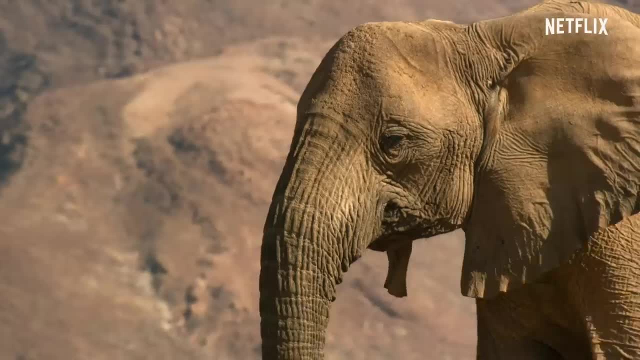 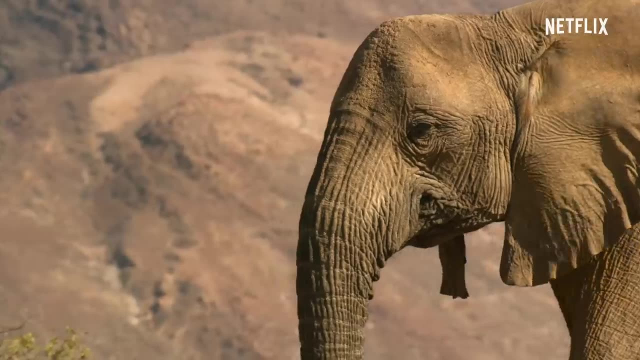 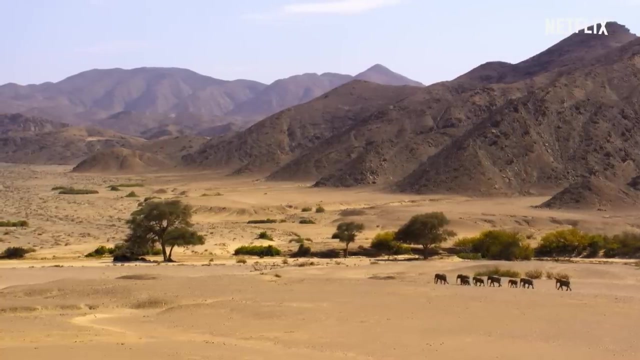 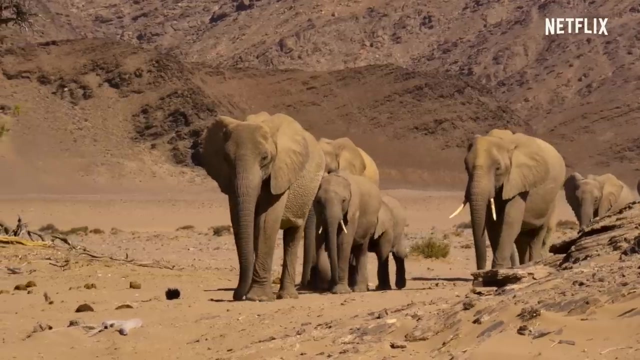 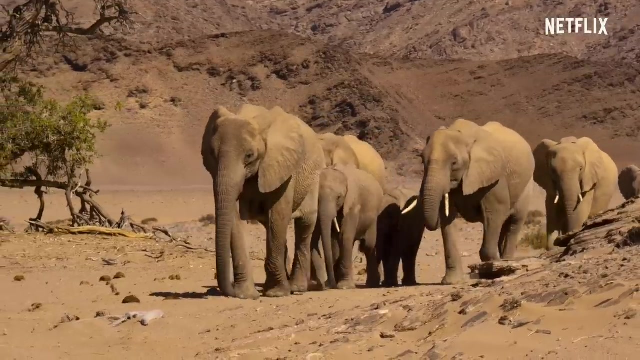 An adult elephant must find up to 200 of them, 100 kilos of food each and every day if it's not to starve. So for these last survivors, life is an endless trek. The herd is guided by a single old female, the matriarch. 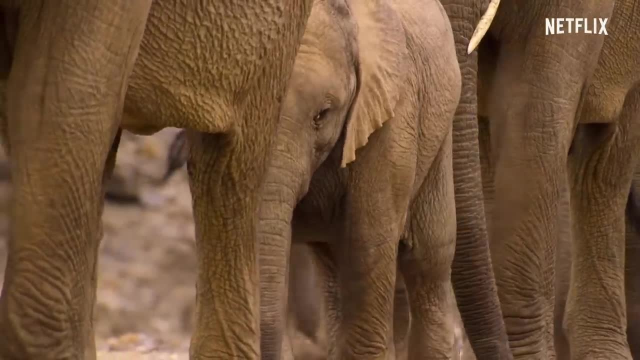 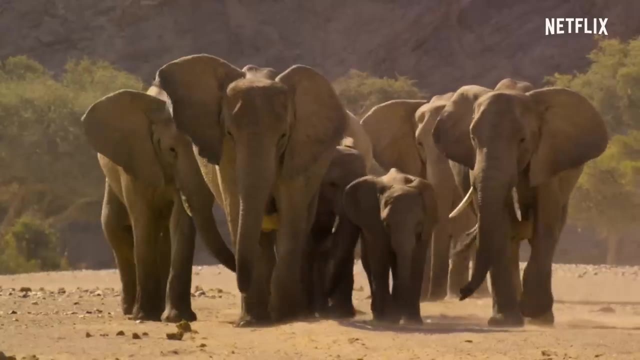 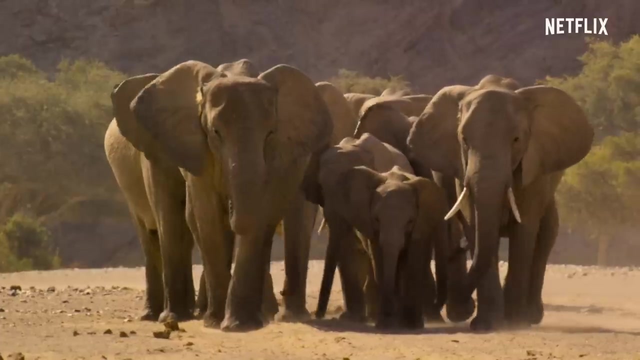 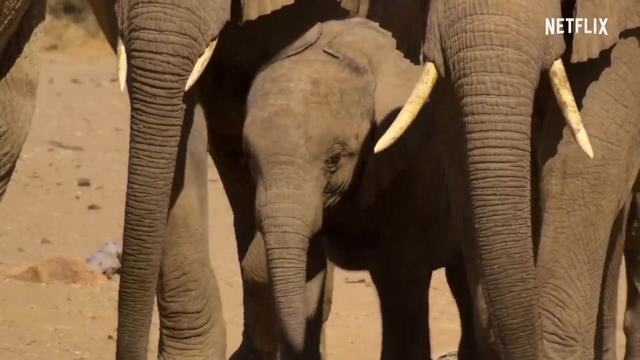 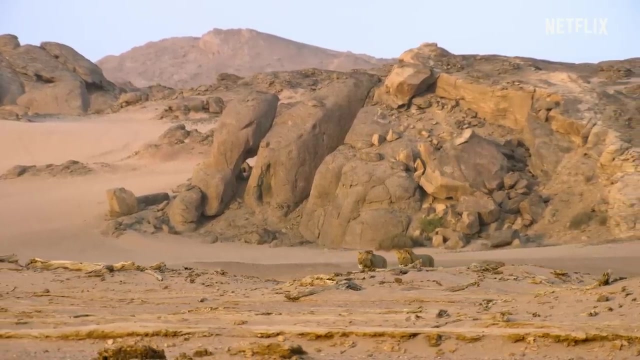 She is leading her family to a special place where food should be available even in the drought. She learned of its existence from her mother many years ago. Now she's teaching her own calf how to get there. The elephants are not alone in their search for food. 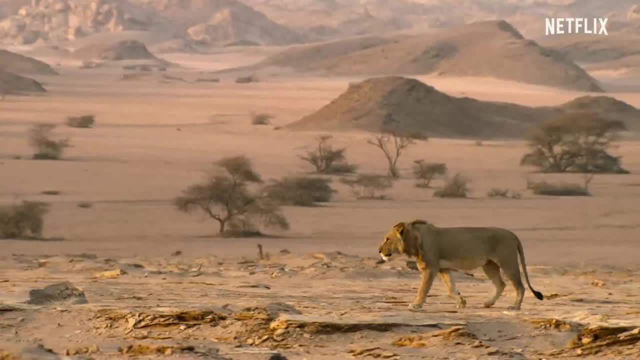 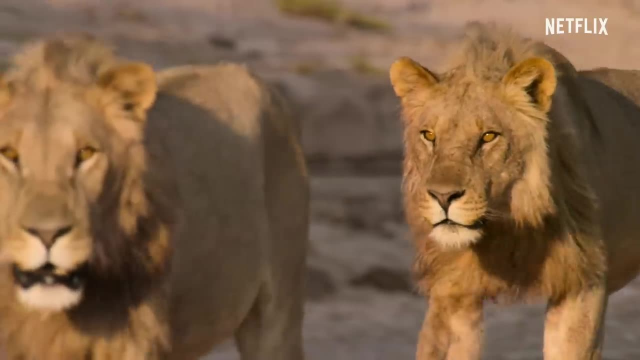 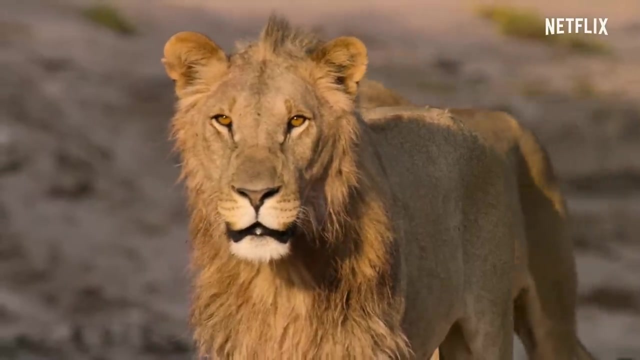 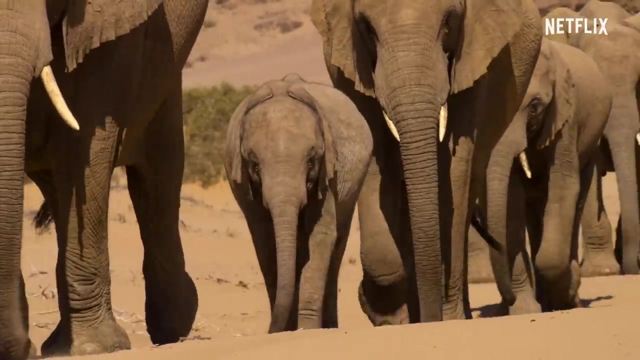 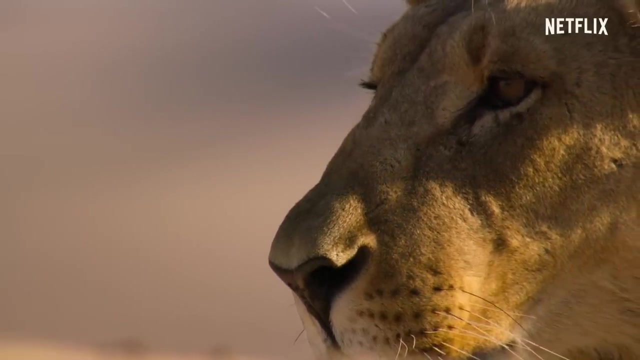 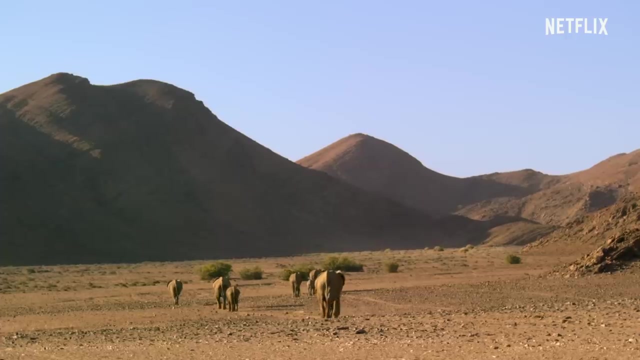 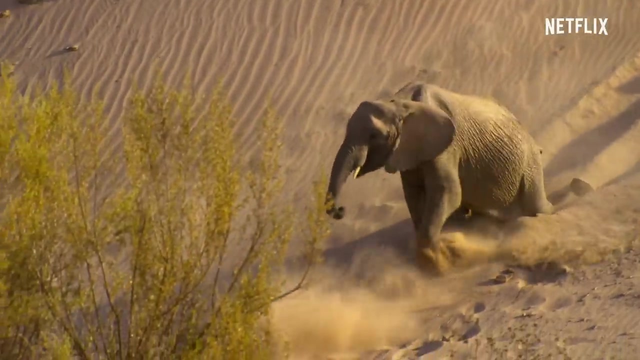 Desert lions. They are just as rare as the elephants. The calf is brought to the desert. The calf is protected by its mother, So the lions let them pass. Distant trees are a sign of water. Desert lions: They are the best bait to feed their families. 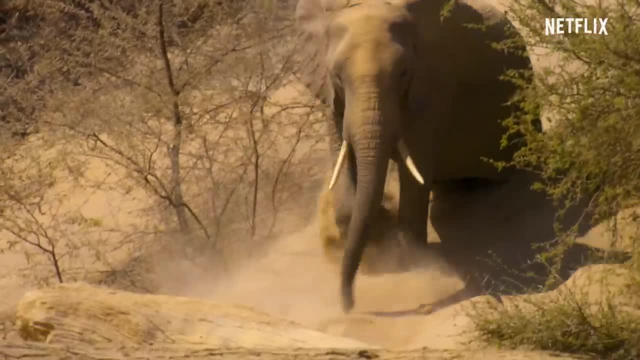 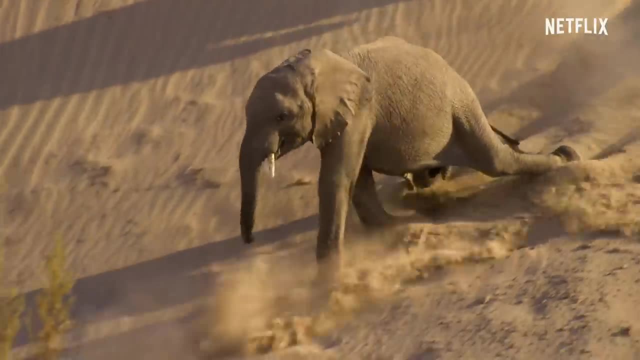 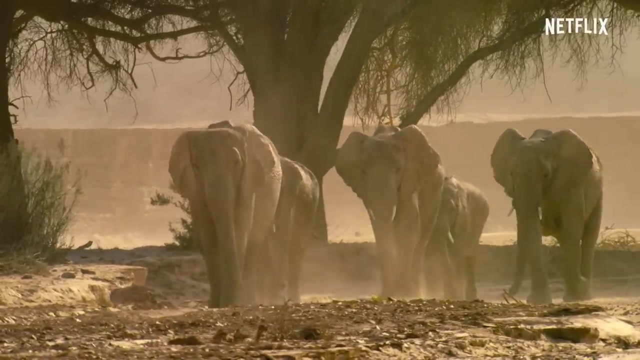 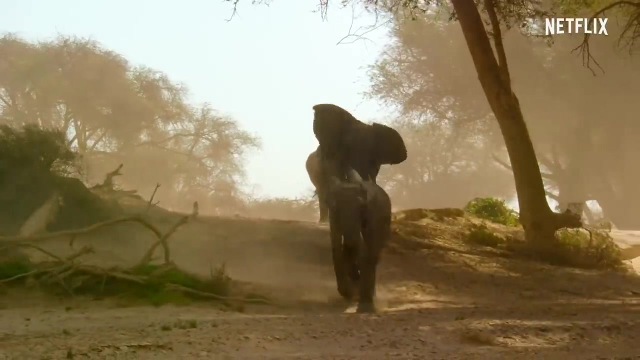 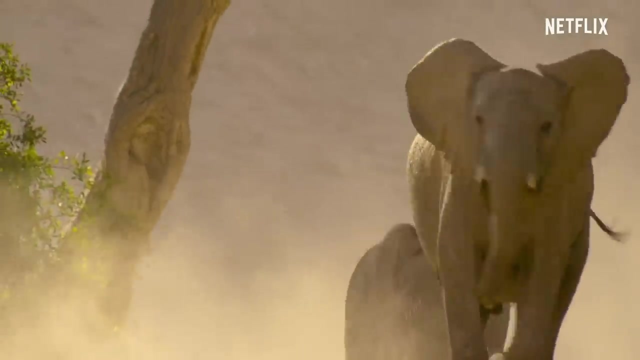 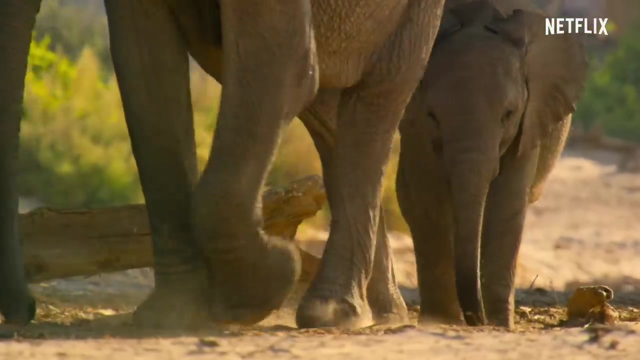 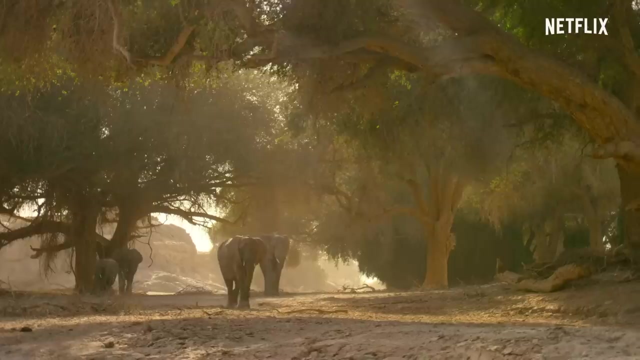 The The riverbed is dry Desert lions. They are as strong as their mother. Desert lions, Desert lions, Desert lions. The anna trees, however, are still green. But there is a problem: At this time of year, seed pods from the anna trees usually litter the ground. 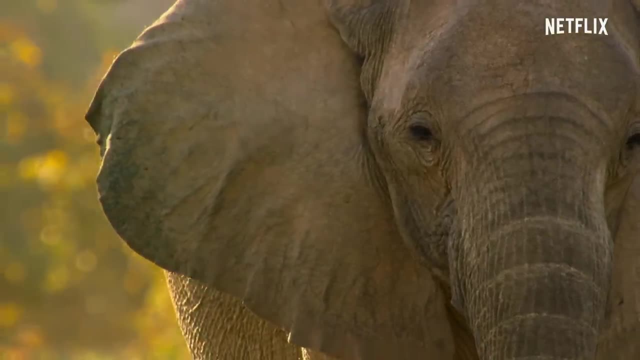 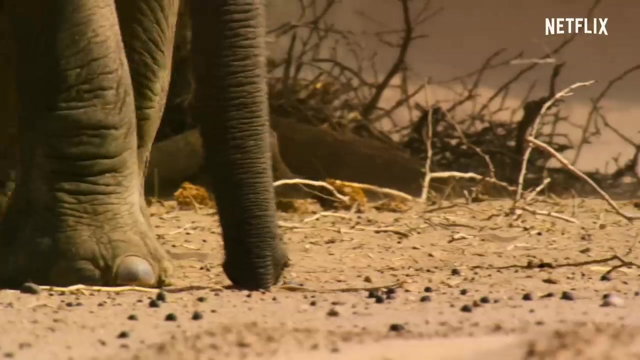 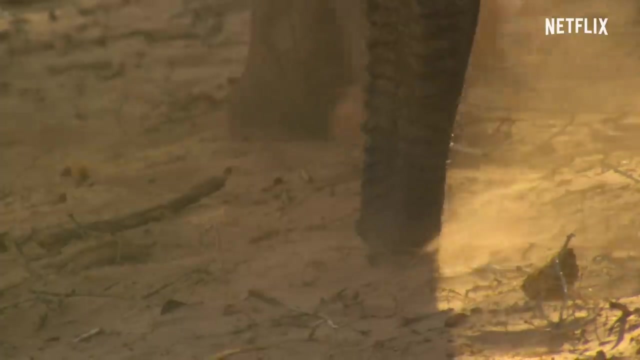 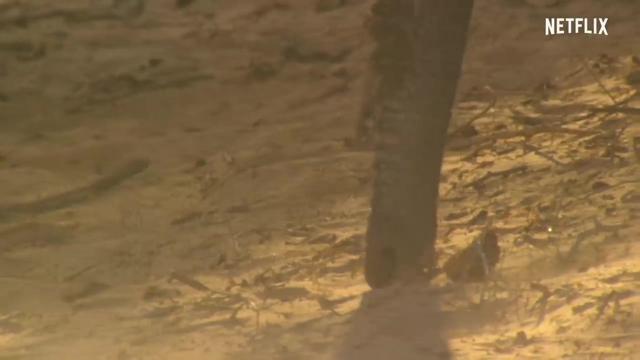 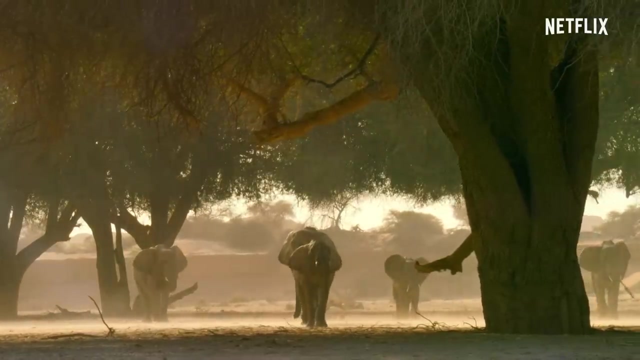 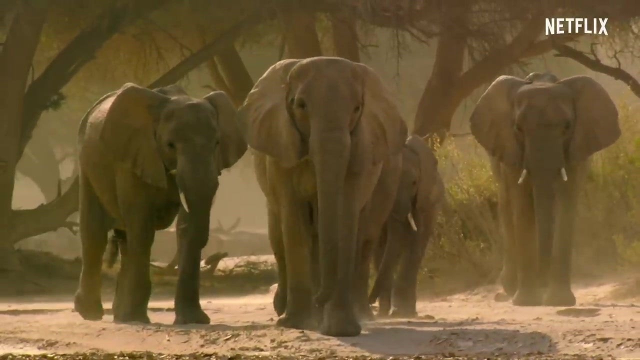 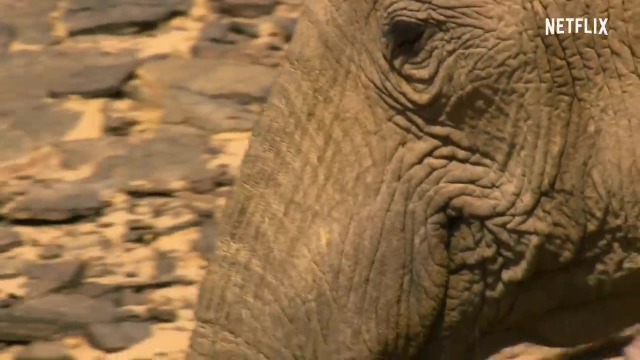 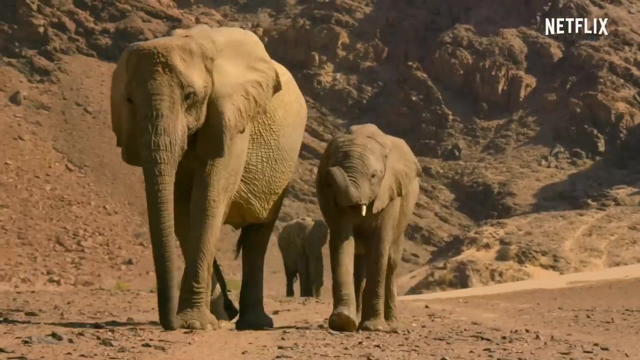 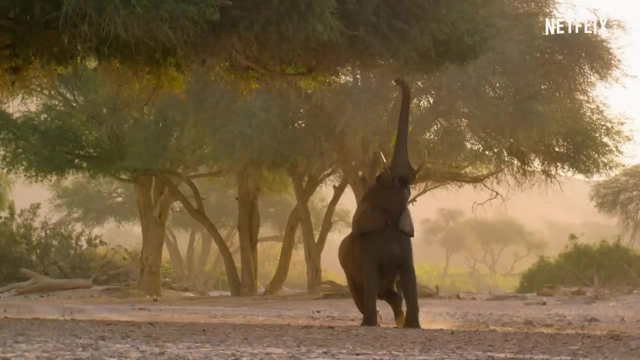 Rich food for elephants, But this year the crop has failed. The matriarch has led her herd here for nothing. Even the tree's leafy branches are out of their reach. The family has no option But to move on. A bull standing nearly four metres tall. 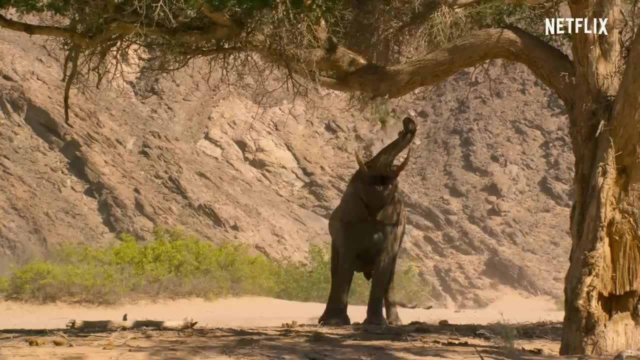 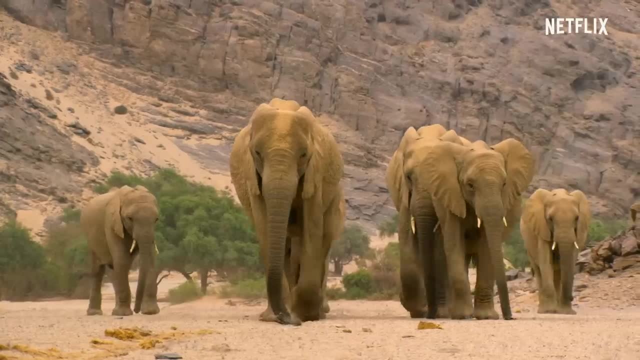 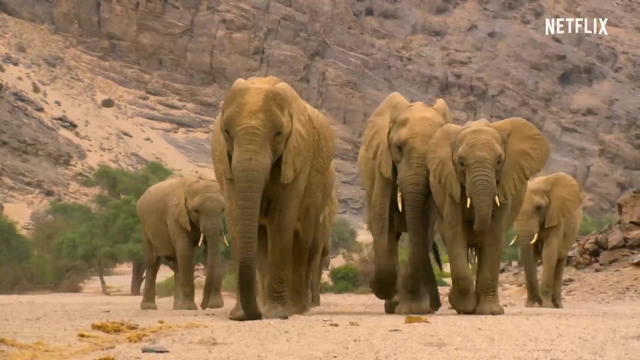 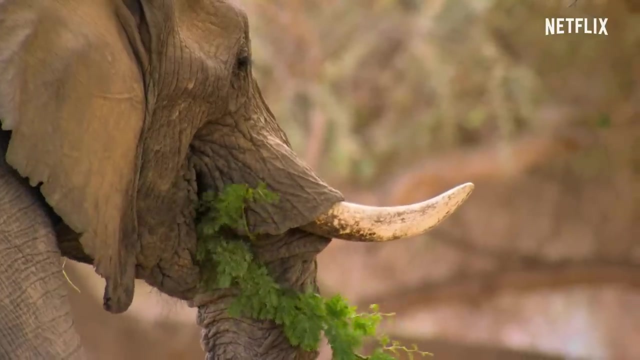 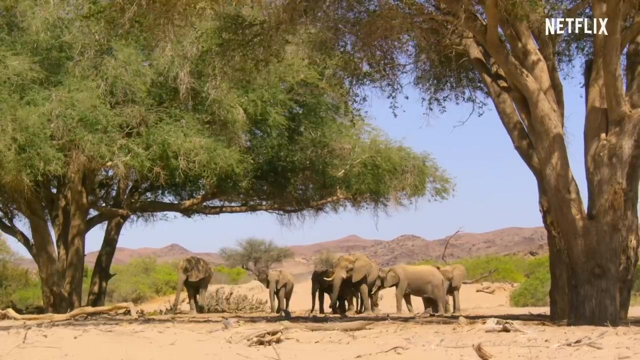 He can reach into the canopy And he could be the solution to their problem. The old female has known him all her life and turned to him for help before. Elephants can only survive here because of knowledge passed down over generations, But less than twenty matriarchs still survive. 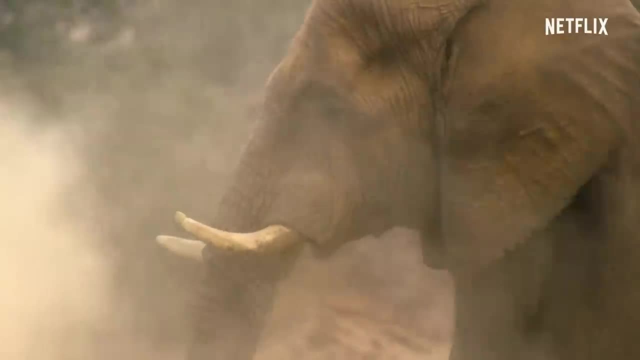 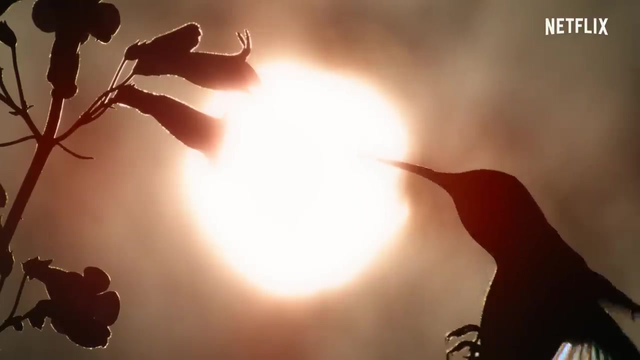 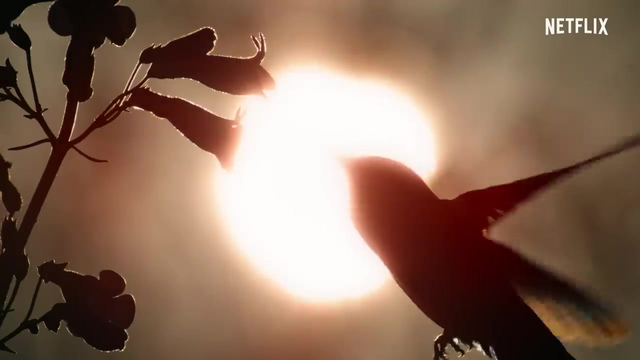 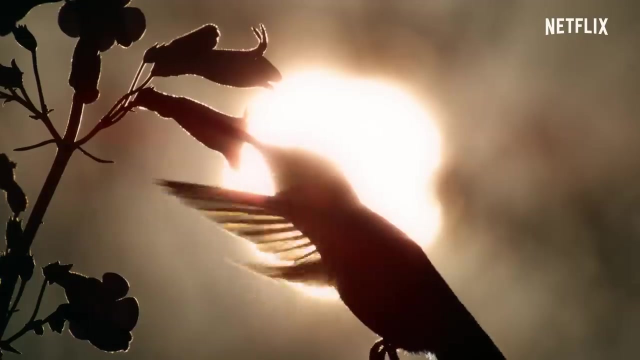 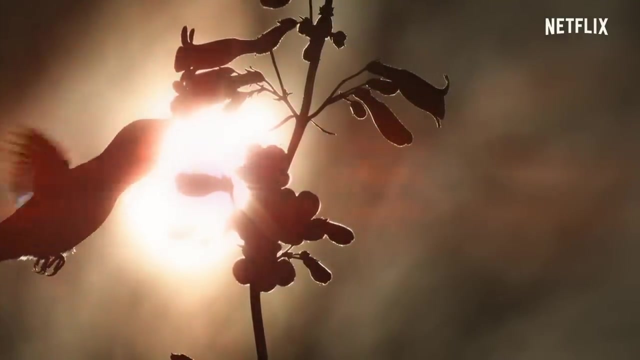 And if their knowledge is lost, elephants may no longer be able to live here. Deserts cannot support large numbers of animals the year round, And even those specially adapted to these conditions can only survive in small numbers. But on very special occasions deserts are transformed. Once in a decade there may be a cloudburst. A single one can turn the desert green. In Southern California the change is visible from space. Hundreds of square kilometers suddenly bloom. If such transformations become regular, a new habitat may develop. 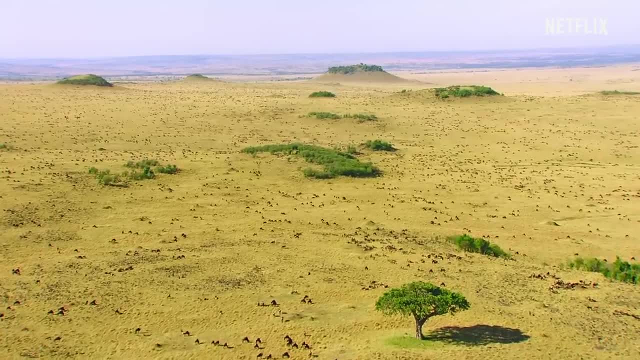 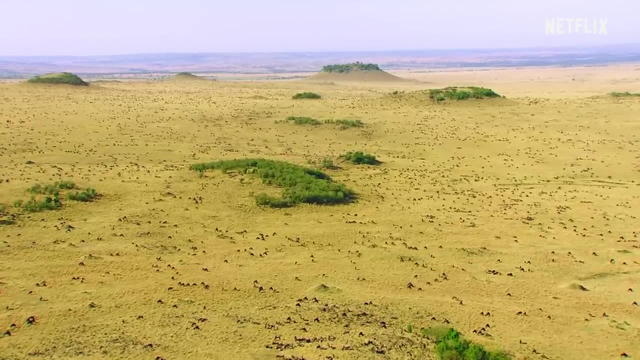 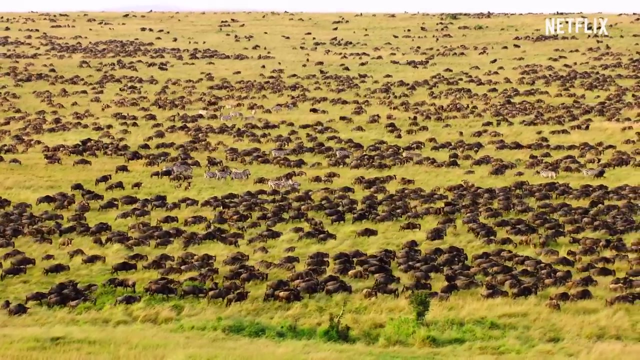 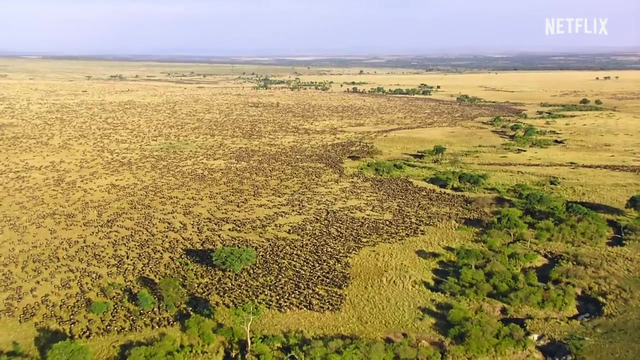 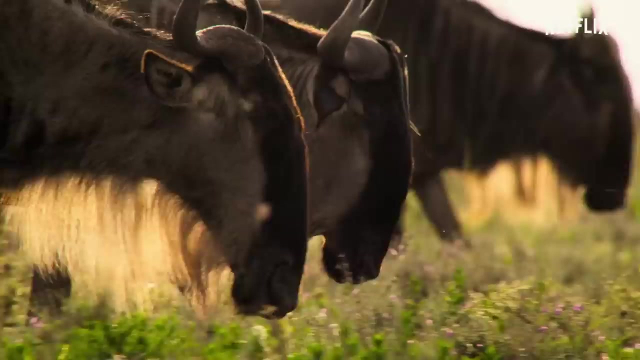 Grasslands, One of our planet's most productive landscapes. They support the greatest aggregations of large animals on Earth. The Serengeti sustains herds of over a million wildebeest. They follow the rains to crop the newly sprung grass. 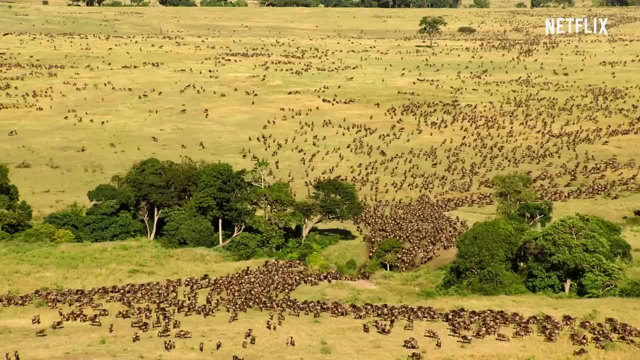 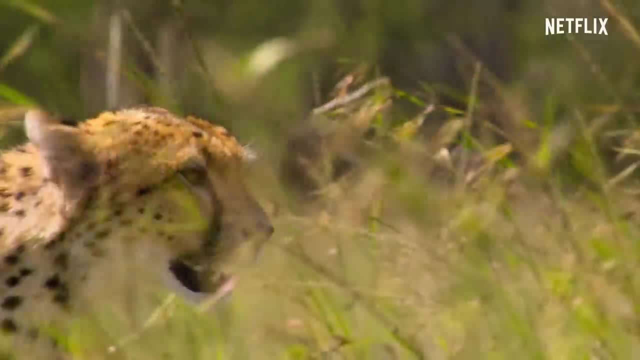 These forest herds attract predators. One of the largest weasels in the world, The Serengeti are singed by the Serengeti. Life's biggest predator is a monarch. The Serengeti's highest prey are the Serengeti. 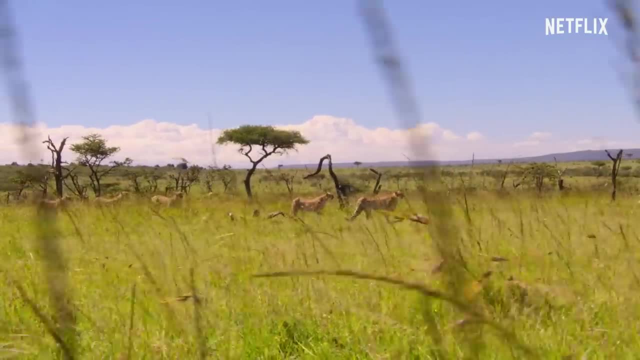 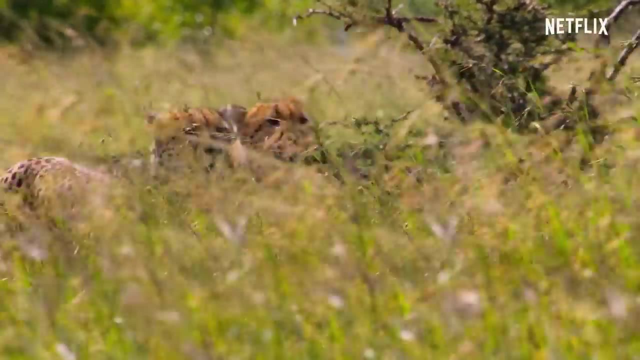 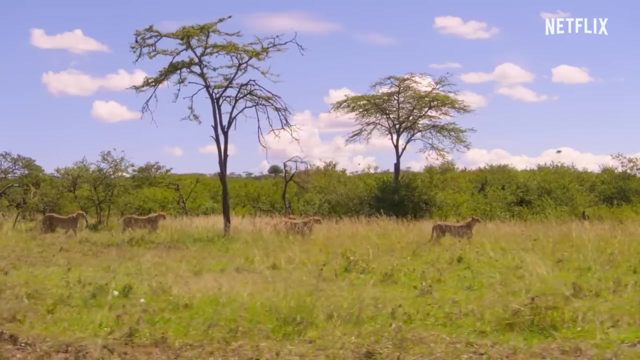 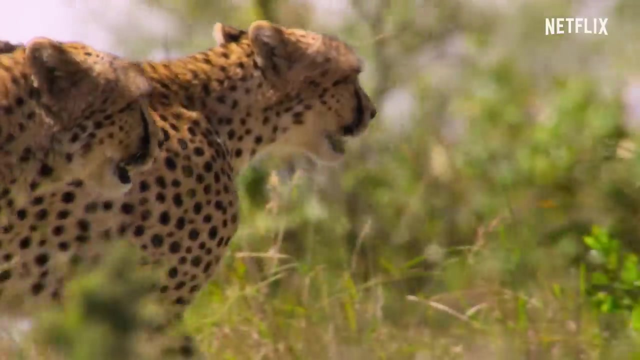 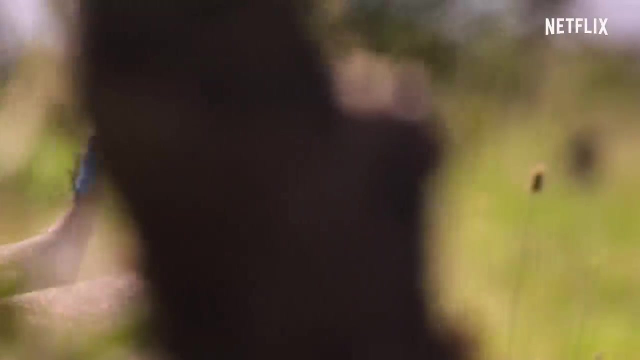 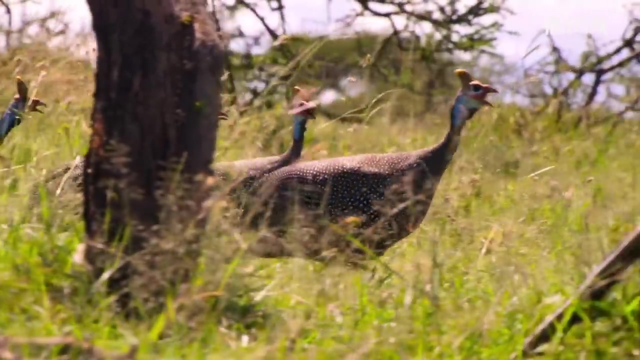 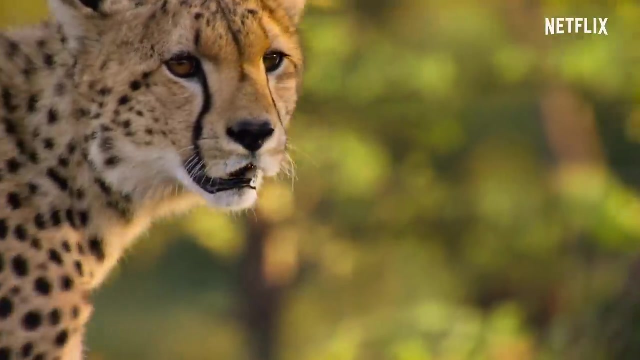 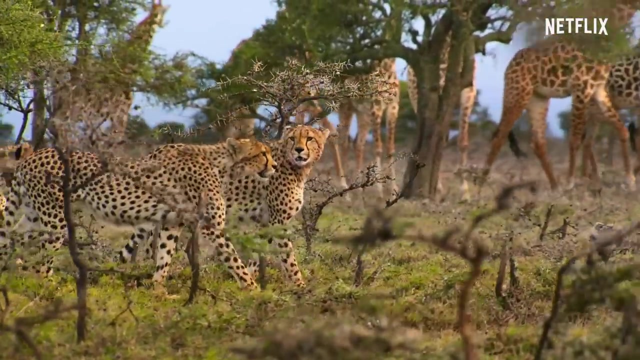 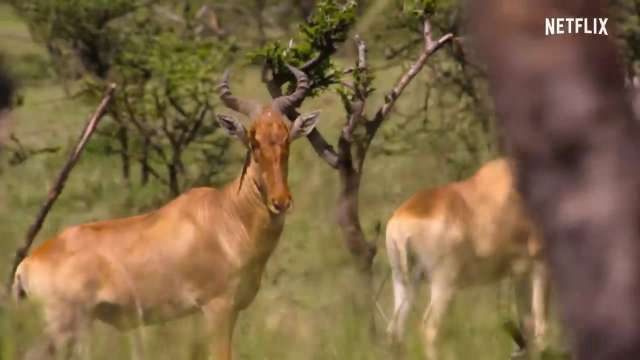 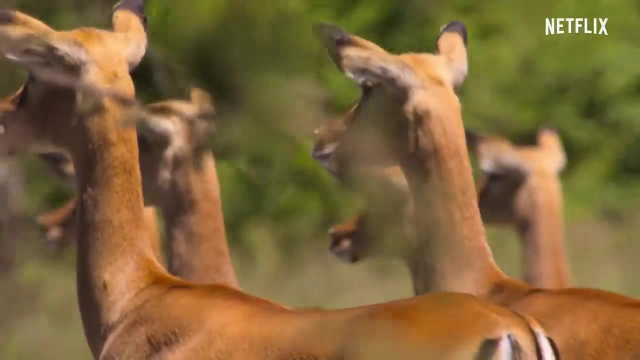 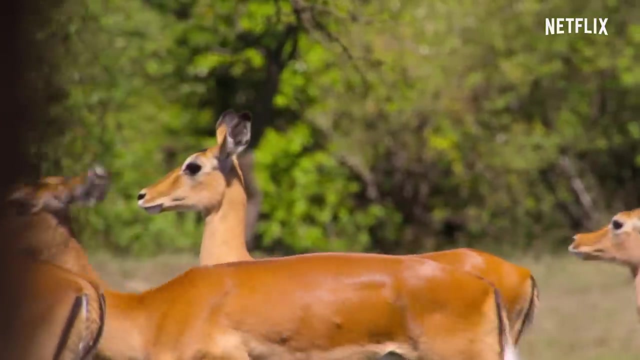 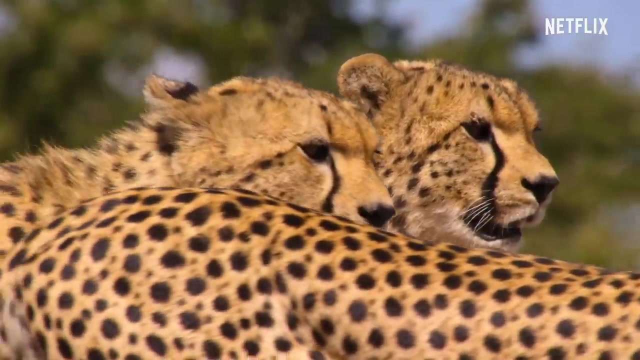 and they are one of the largest predators: Five male cheetahs, One of the largest coalitions ever observed, 150 square kilometers. They patrol it together And that attracts attention. SIREN WAILS. A change of strategy is needed if they're to hunt successfully. 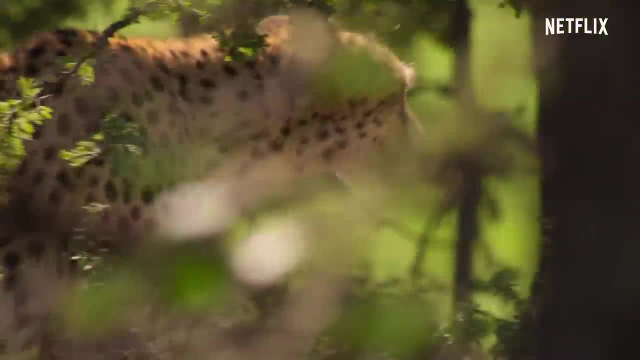 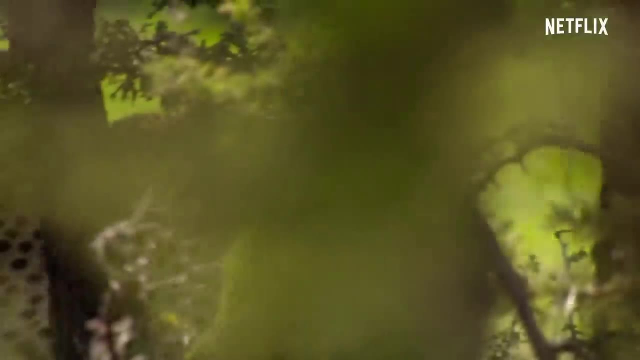 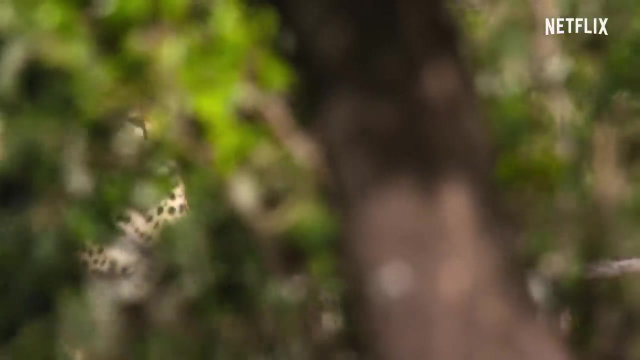 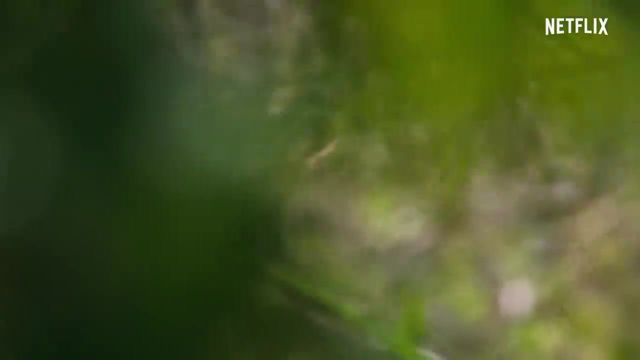 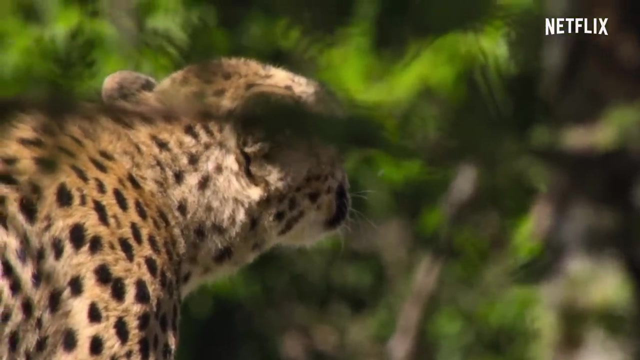 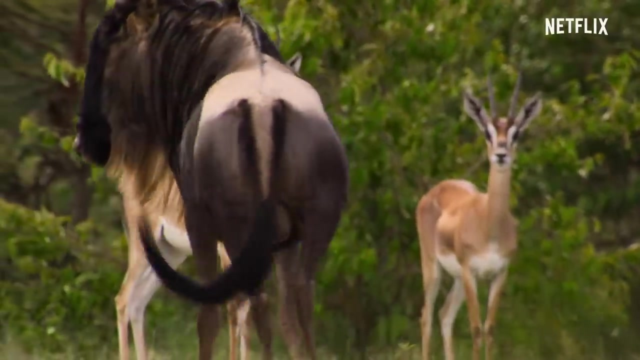 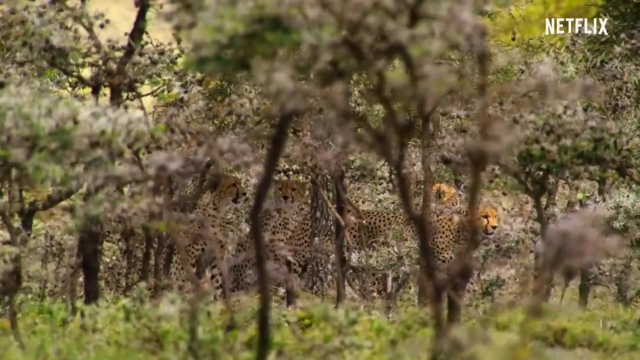 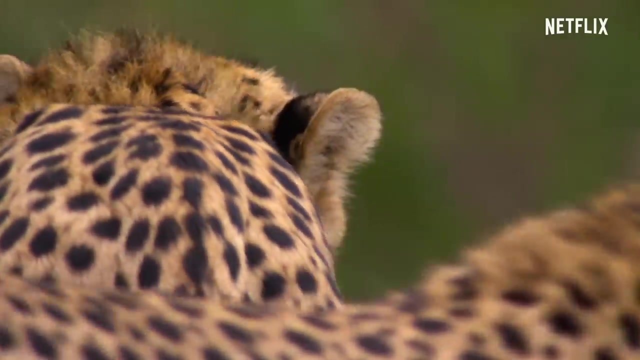 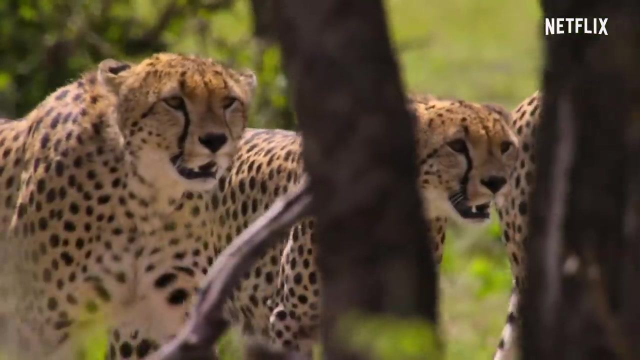 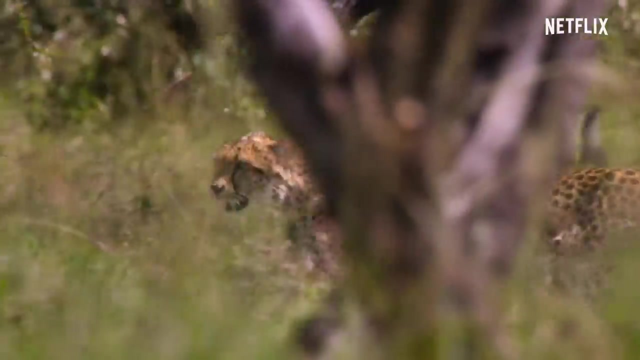 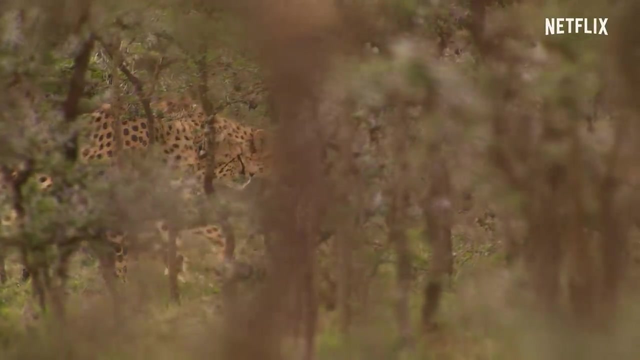 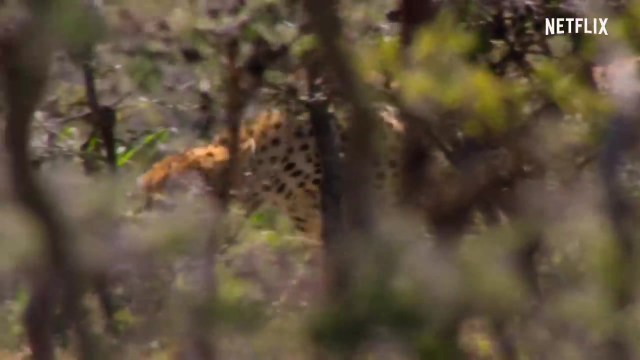 They need cover. An adult wildebeest is a formidable opponent. Four of the cheetahs start the stalk, walking directly towards the prey. The fifth creeps around the side. SIREN WAILS, SIREN WAILS, SIREN WAILS. 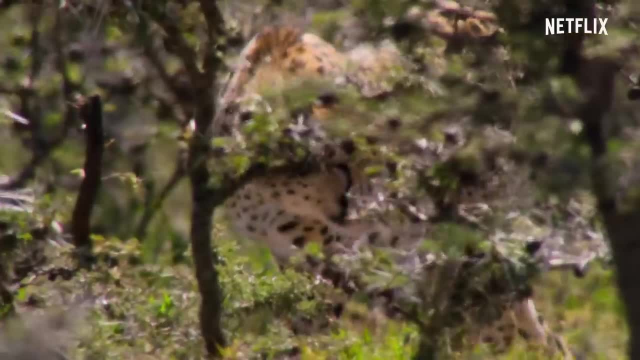 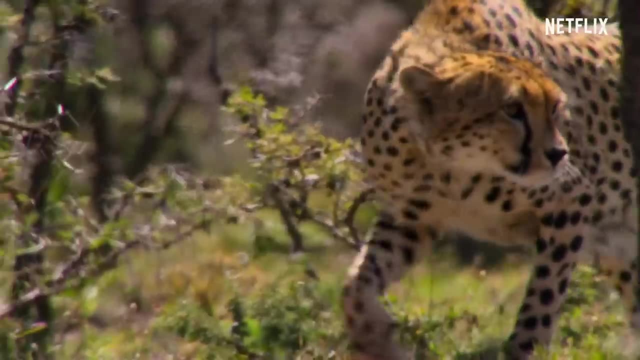 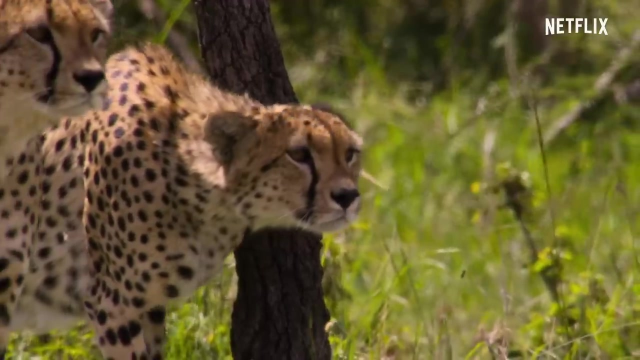 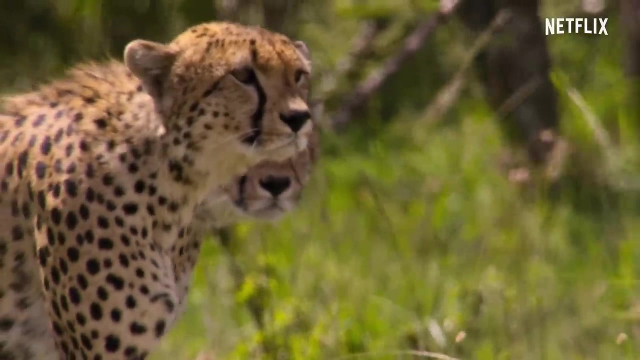 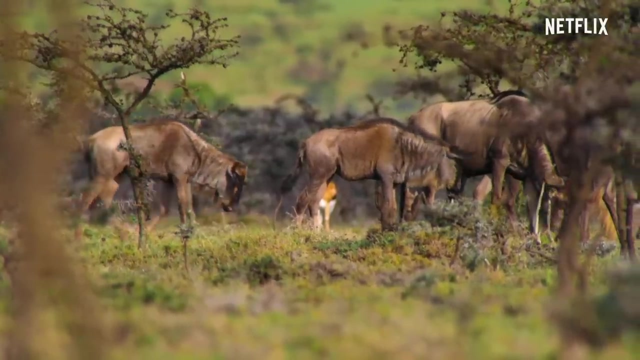 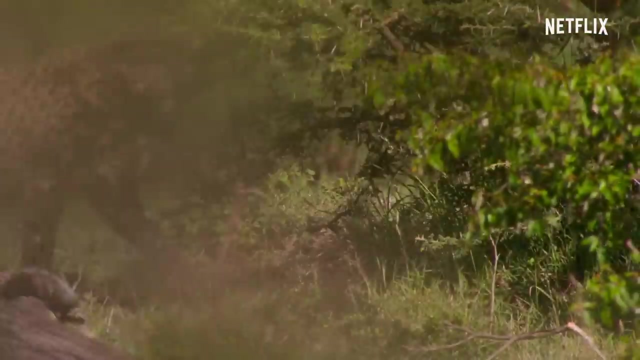 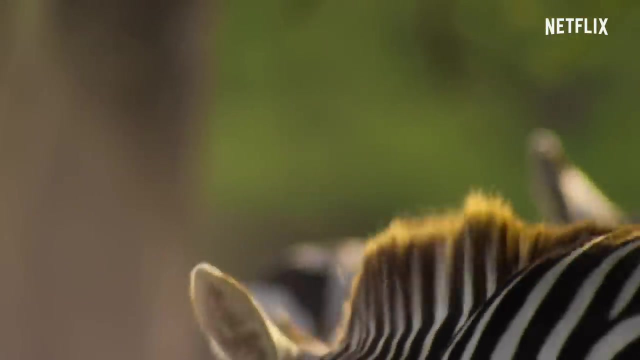 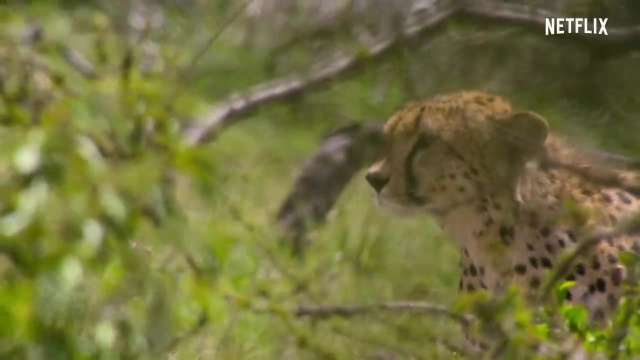 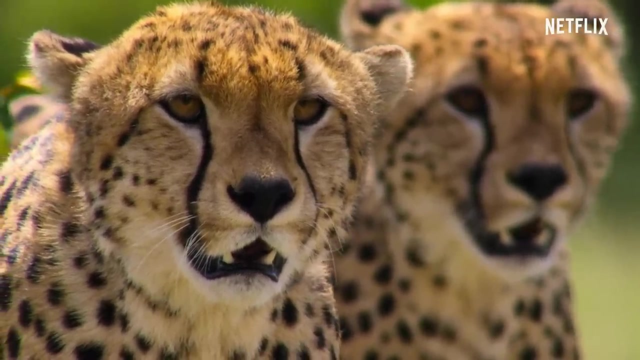 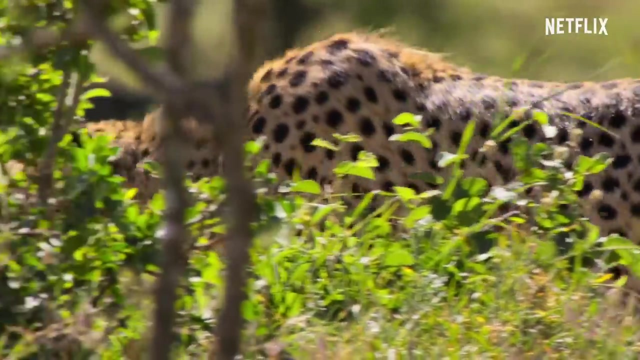 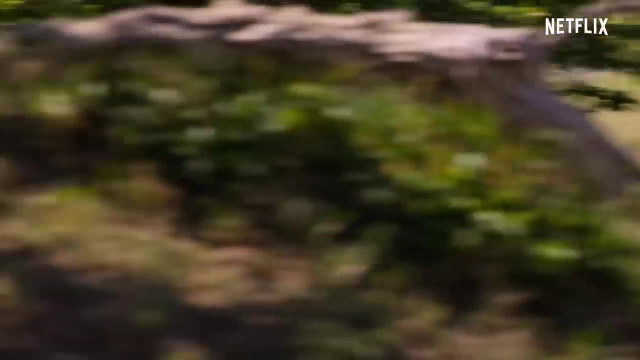 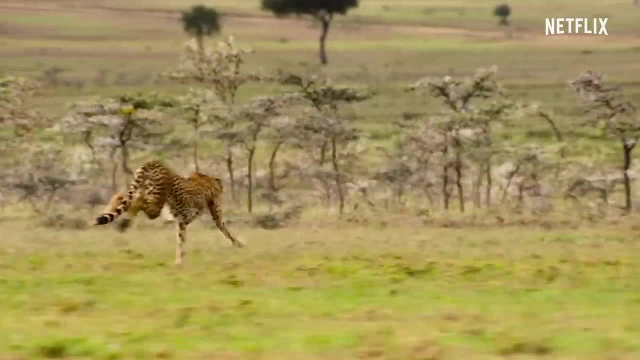 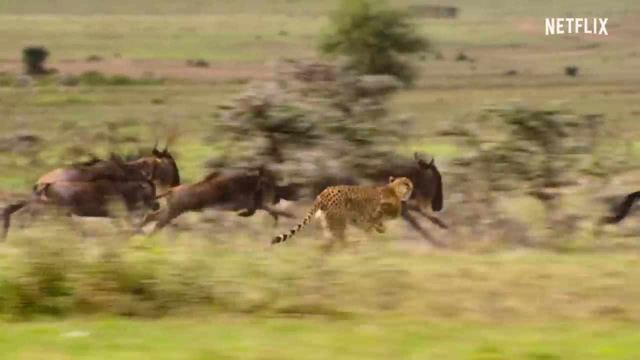 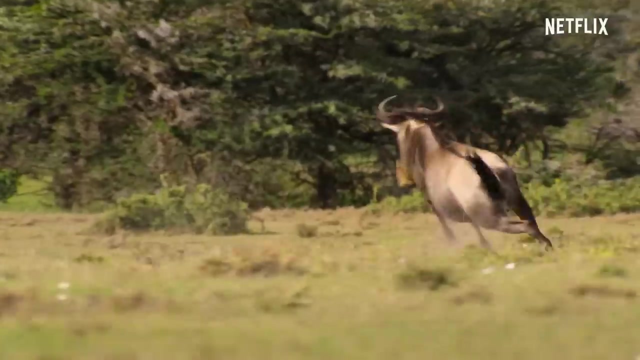 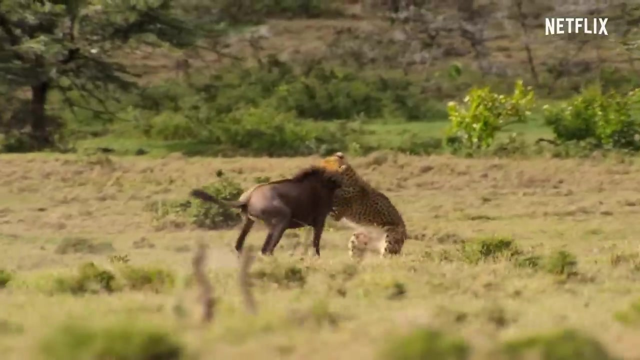 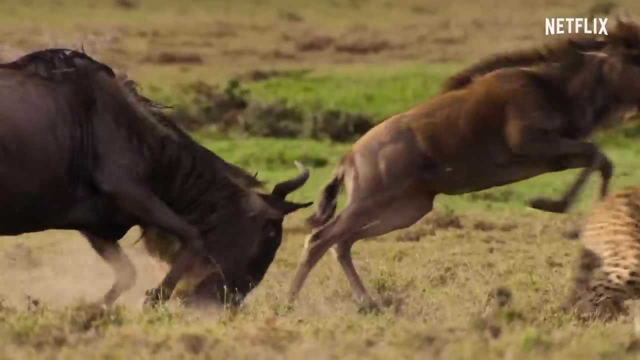 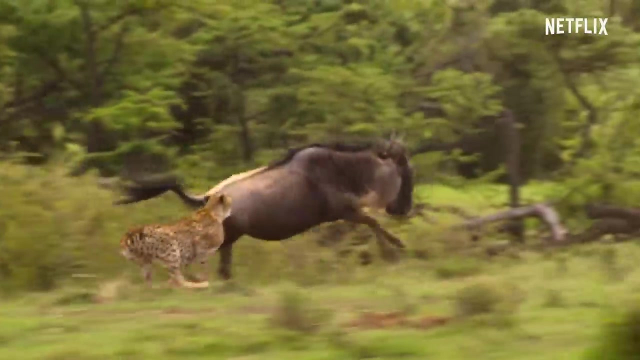 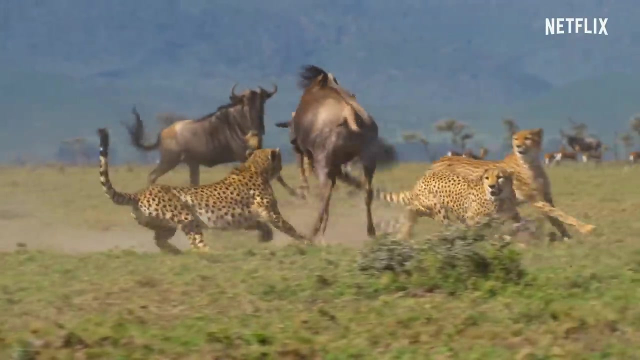 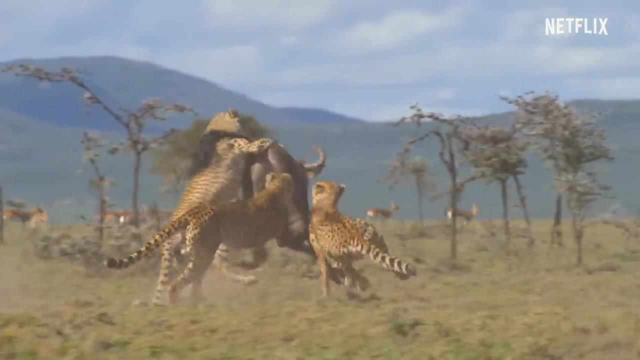 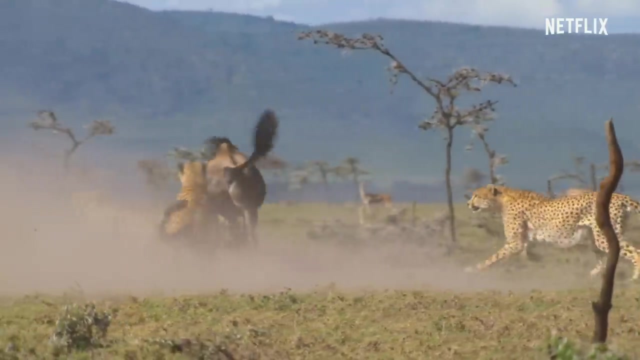 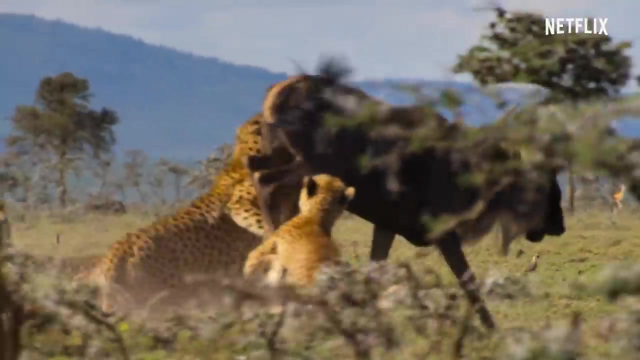 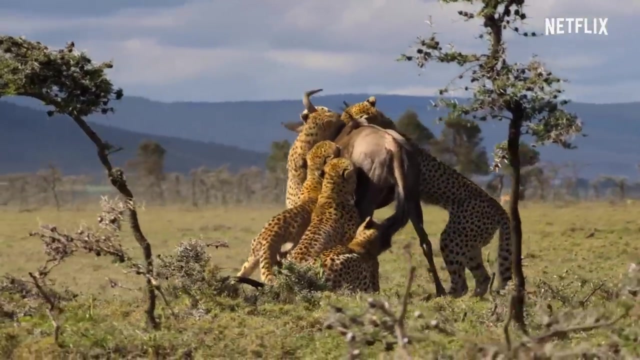 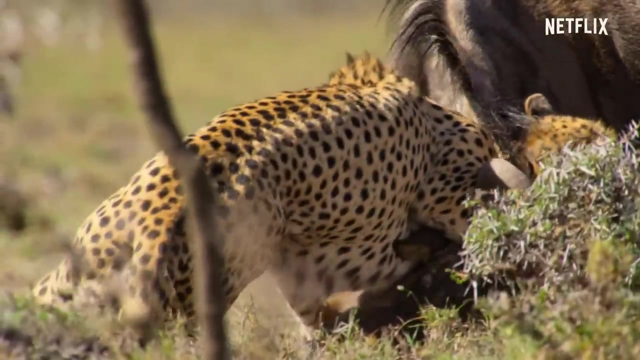 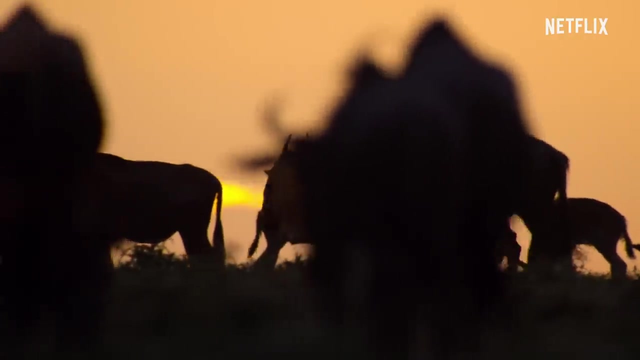 Each cat chasing a different target. It's chaos. A single cheetah is not strong enough to defend its prize. They must work together, They must work together, They must work together. These dramas only continue because the Serengeti is protected. 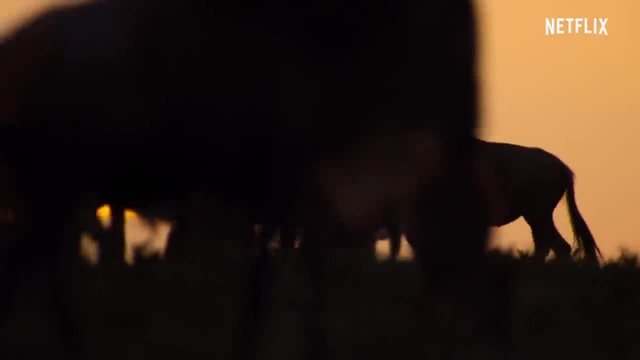 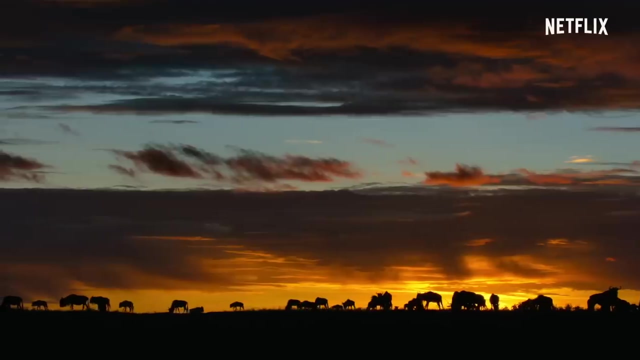 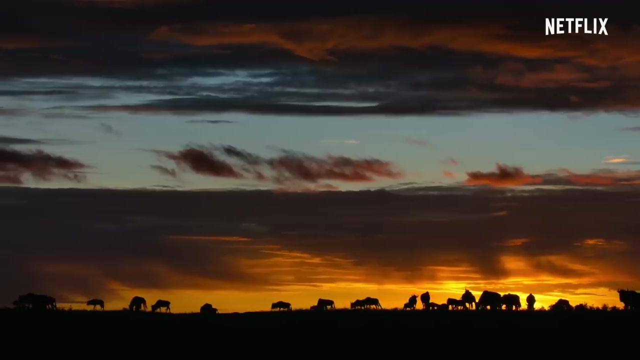 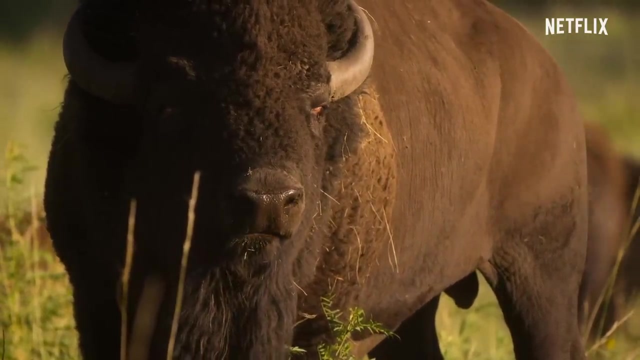 and has been for over 65 years. But the Serengeti is an exception. Across the planet, space for grasslands has been steadily disappearing. 180 years ago, herds of bison, millions strong, grazed the great plains of North America. 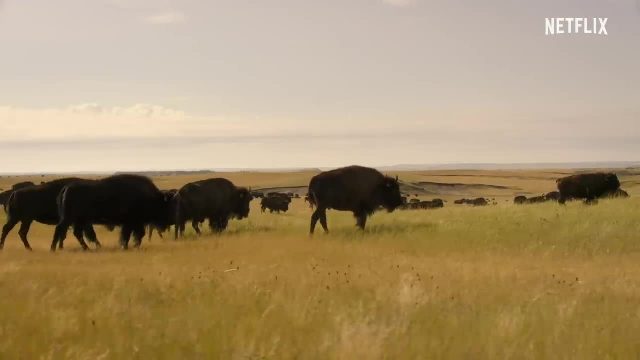 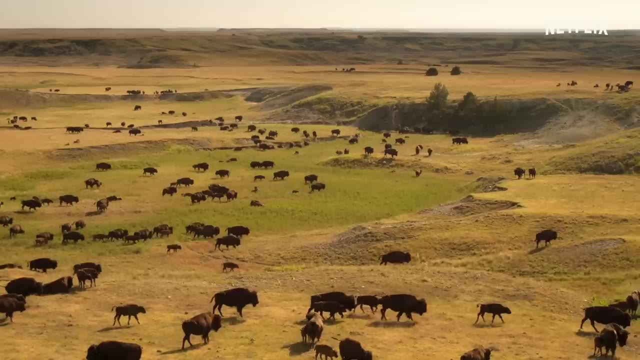 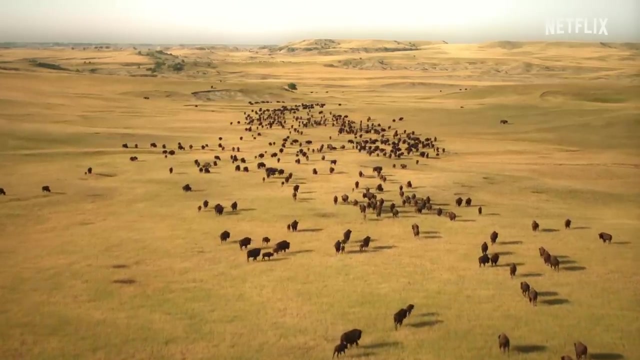 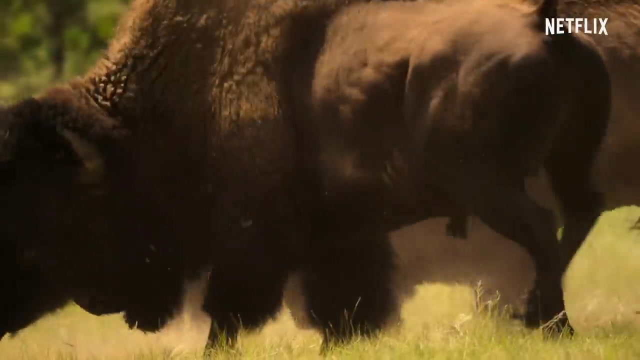 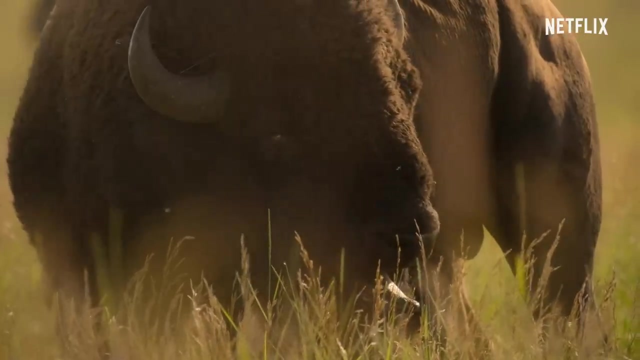 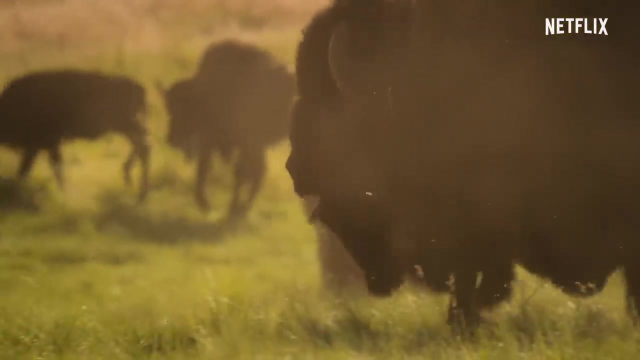 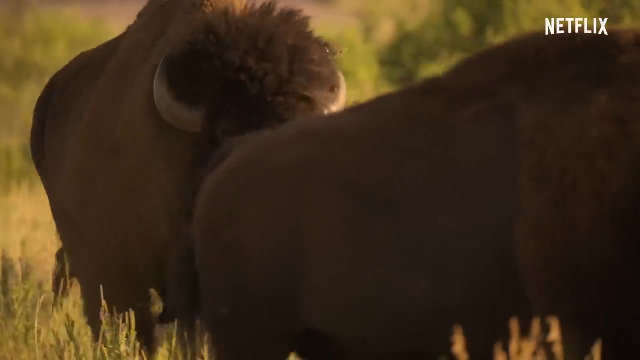 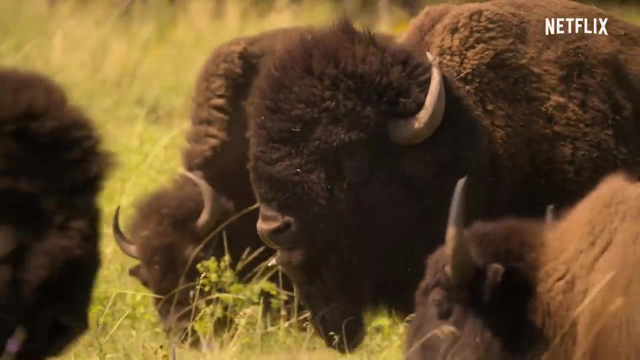 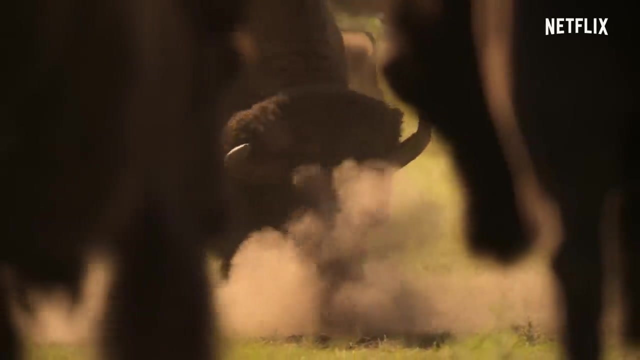 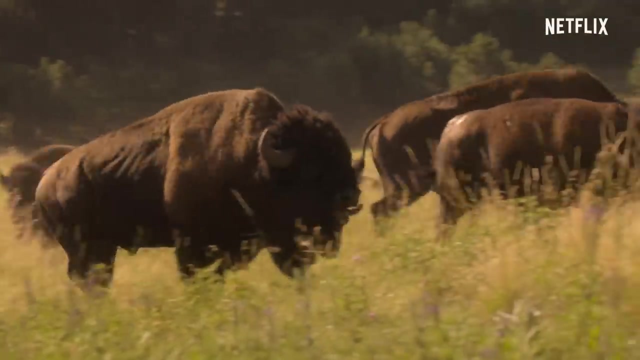 They roamed across a prairie a hundred times larger than the Serengeti. This was the true Wild West cosmopolitan's. Every summer, the males roared their challenges and fought for possession of the females. As the rut intensified, the fights became more brutal. 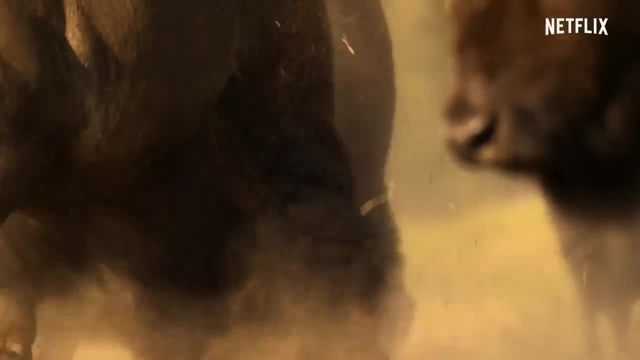 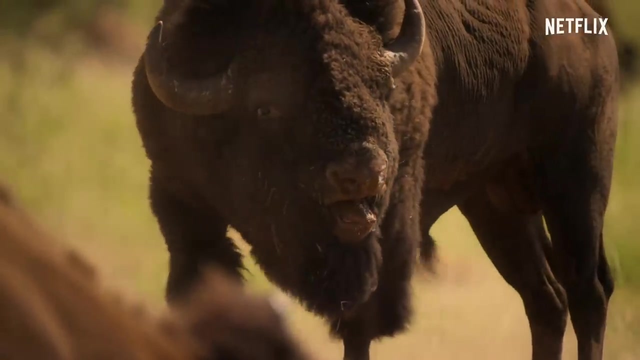 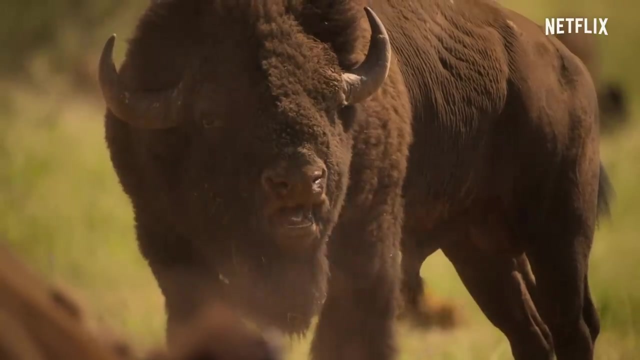 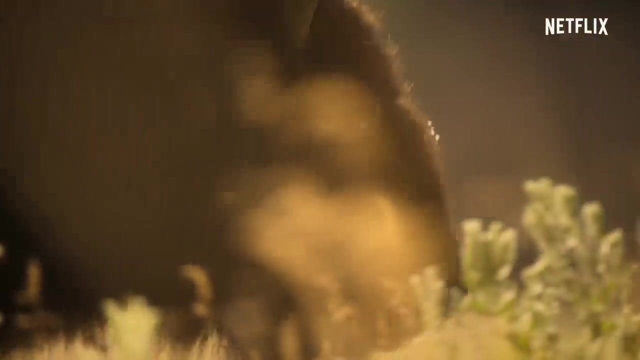 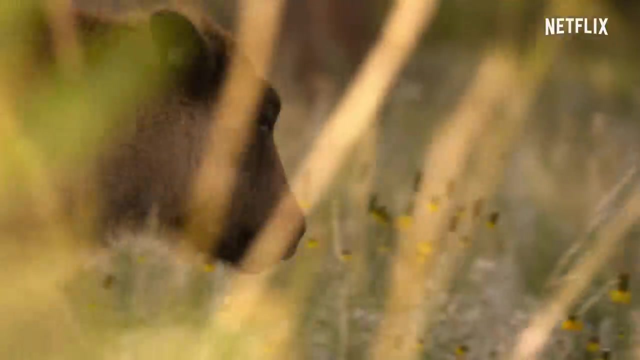 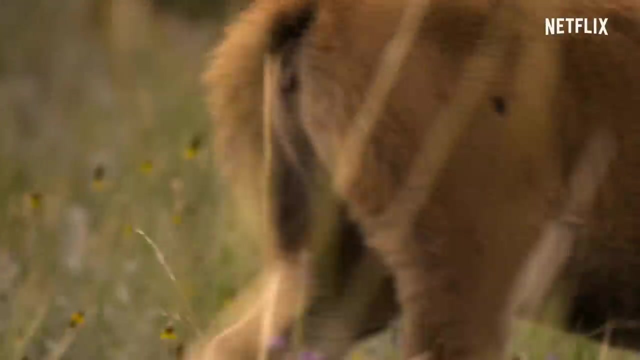 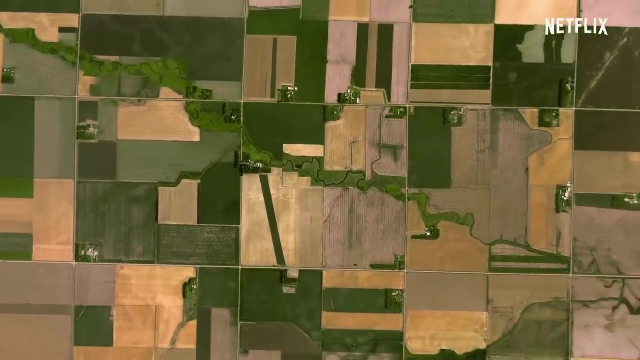 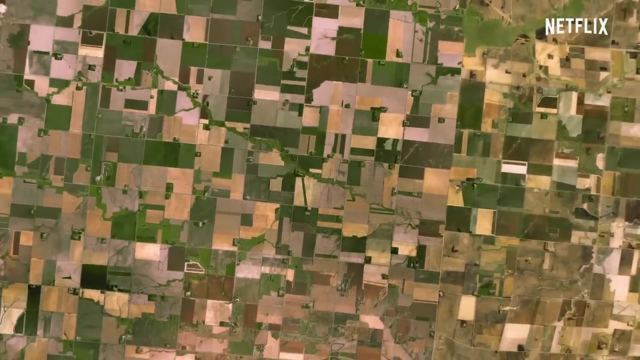 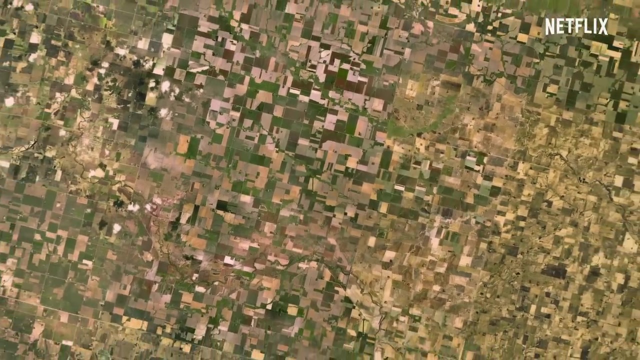 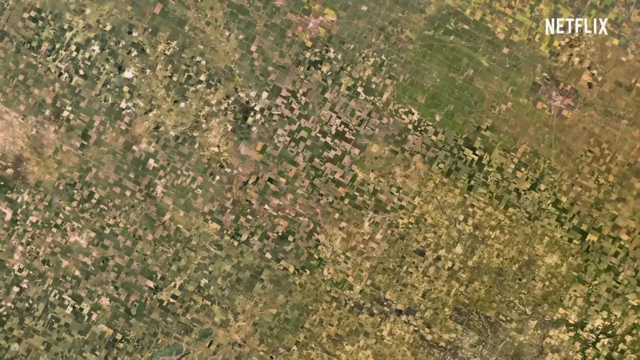 Today, however, most of the prairie is silent. Humans slaughtered the great herds, Less than 30,000 wild bison remain And 90% of the prairie has been lost. Most of it to agriculture: What we eat and how we produce it. 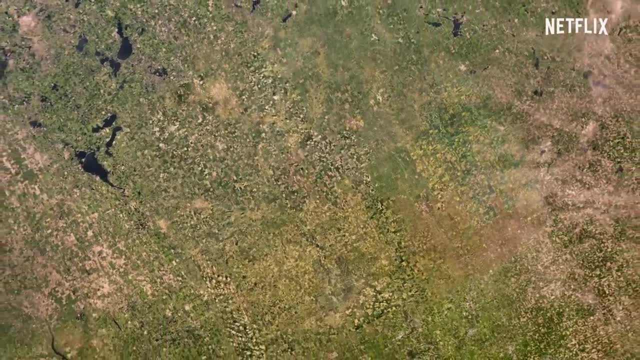 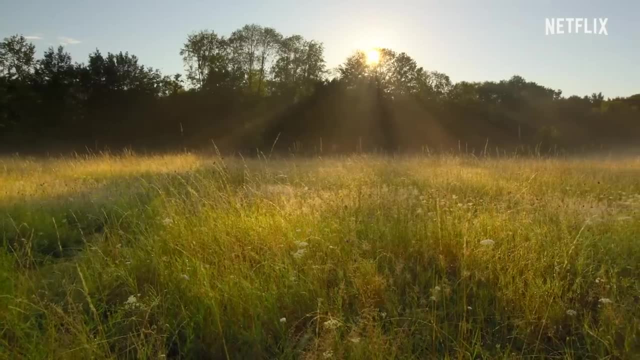 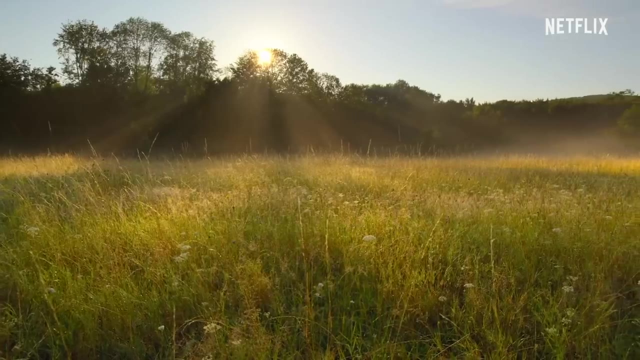 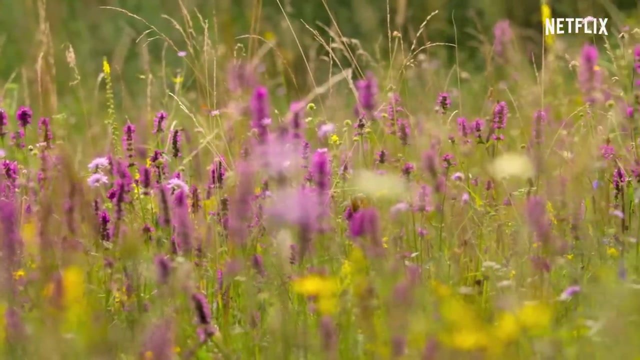 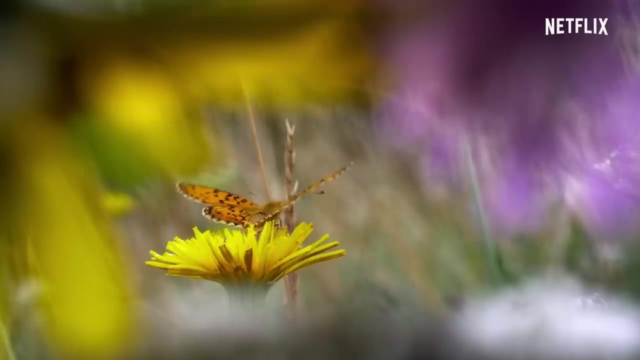 will determine the future of our planet's grasslands. Our past could show us how we can feed ourselves and survive, But still leave room for nature. The ancient hay meadows of Hungary, still farmed in the traditional way, provide habitats of extraordinary richness. 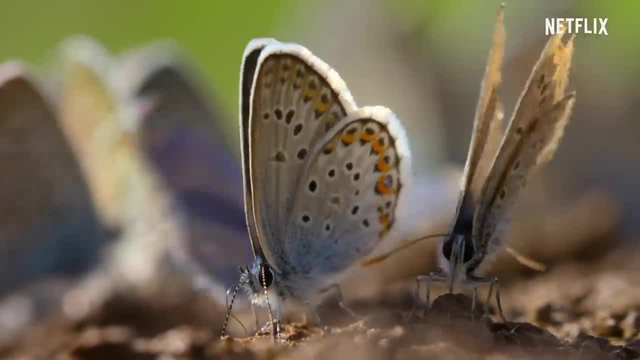 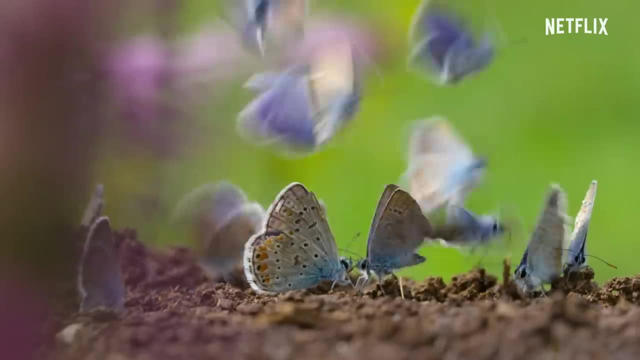 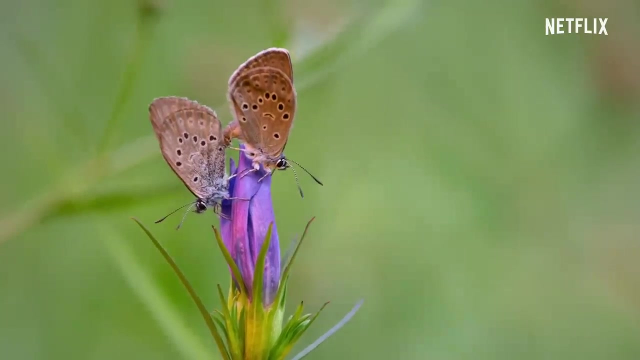 Butterflies are abundant. They can be found in the forest. Some can even be found in the wild. One species has an almost unbelievably complex life cycle. How does it work? That is why I want to introduce you to another species. It has a common name. 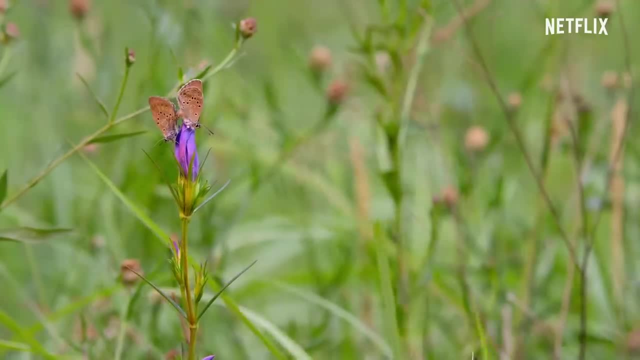 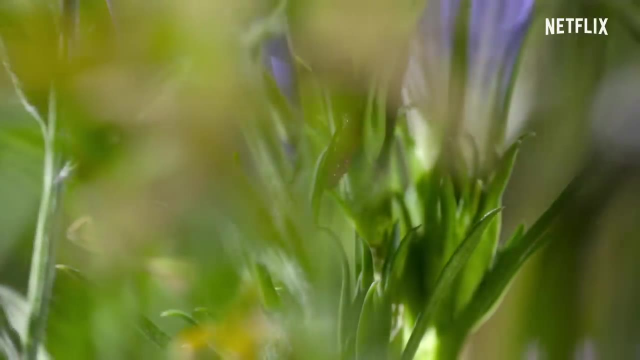 Like this other one, It's called the great white. The white is a compound of alcon blue. Each female must mate and lay eggs on just one species of plant, the marsh gentian. What's it like? The eggs soon hatch into caterpillars. 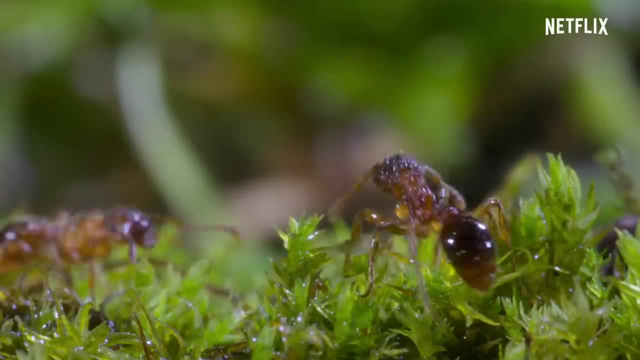 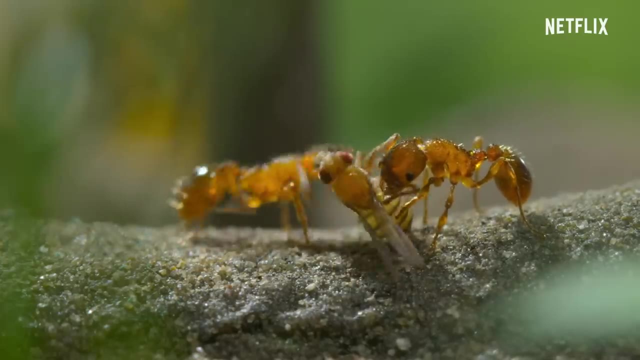 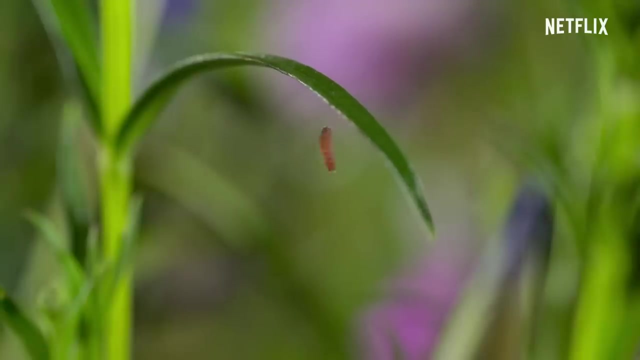 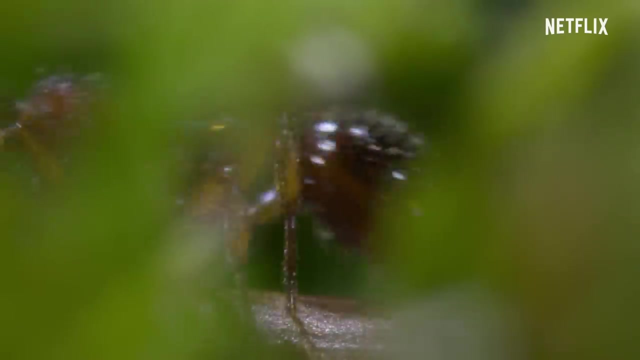 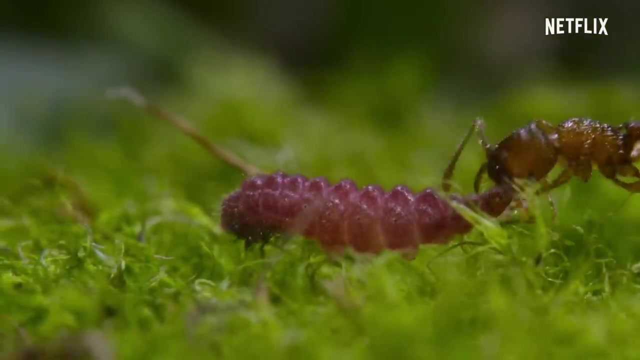 High up on the plants, they're safe from predators below. But then the caterpillars do something seemingly suicidal. They abseil down on threads of silk to the ground below and into danger. They have no defense against the marauding ants which carry them off. 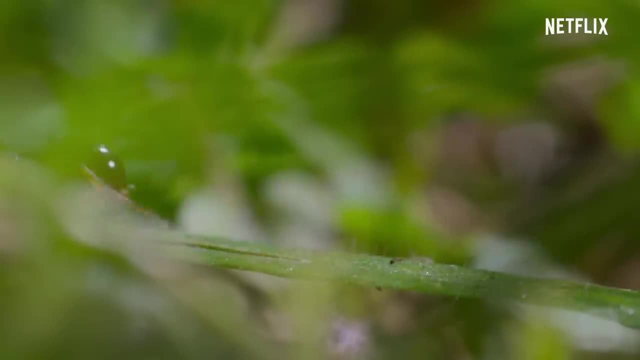 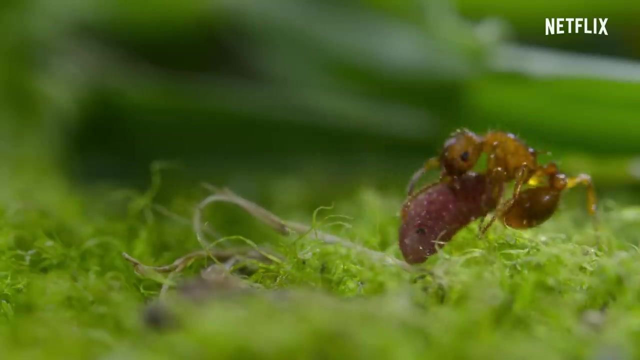 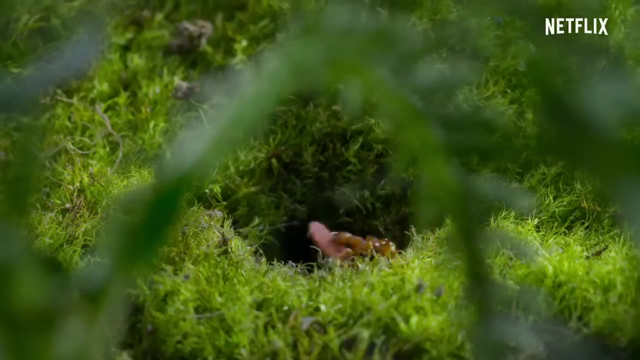 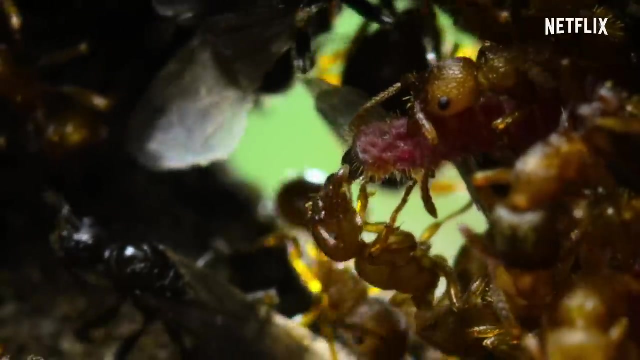 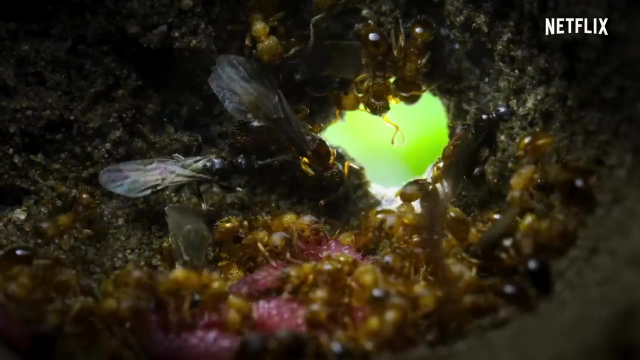 But this is the only way to keep them safe. This is exactly what the caterpillars need to happen. They're producing a scent like that emitted by an ant larva. The ants respond by taking them back to their nest. There they deposit them in the colony's brood chamber. 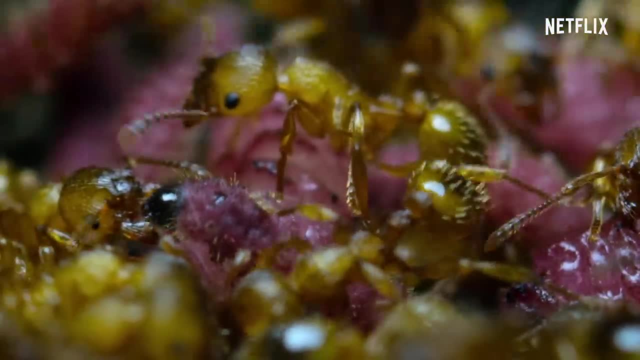 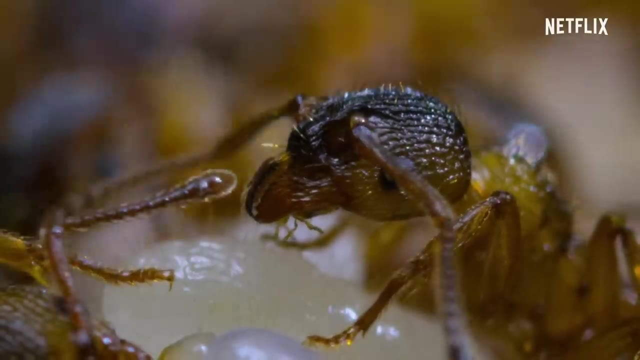 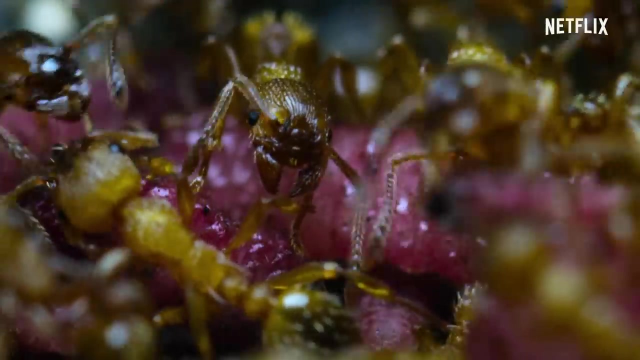 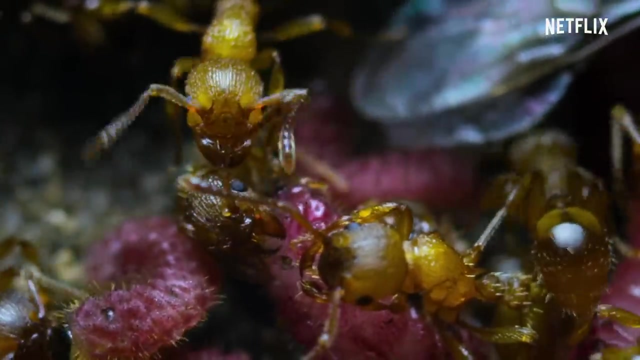 The purple-colored caterpillars lying among the ants' own white larvae give off just the right signals And the nurse ants rush to feed them. But there is more: The caterpillars now start to mimic the sounds made by the queen ant. 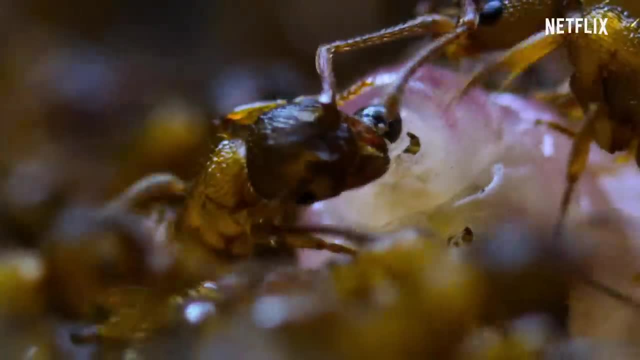 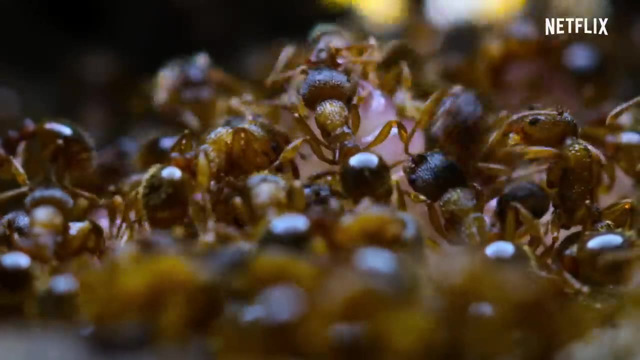 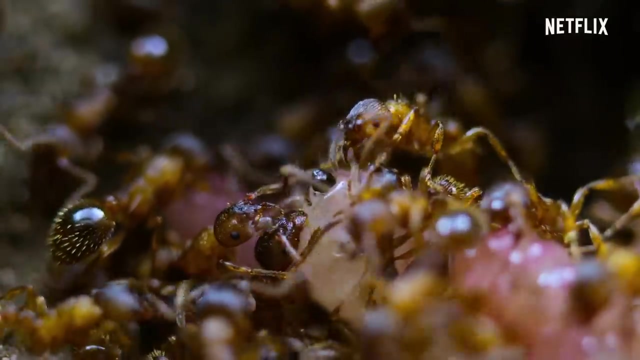 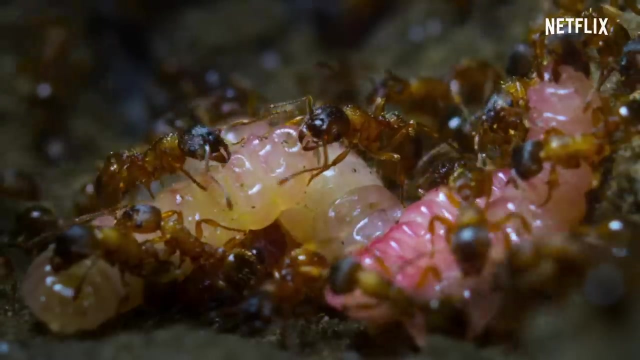 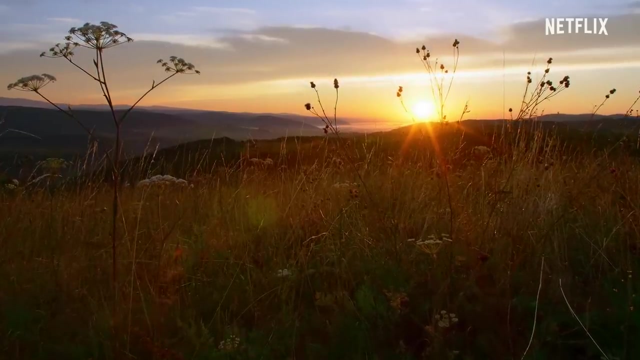 And as a result, the ants treat them like royalty. If food gets short, the ants will even feed the caterpillars instead of their own young. They give them such quantities of food that the caterpillars grow hugely, And there underground the caterpillars feed and grow for nearly two years. 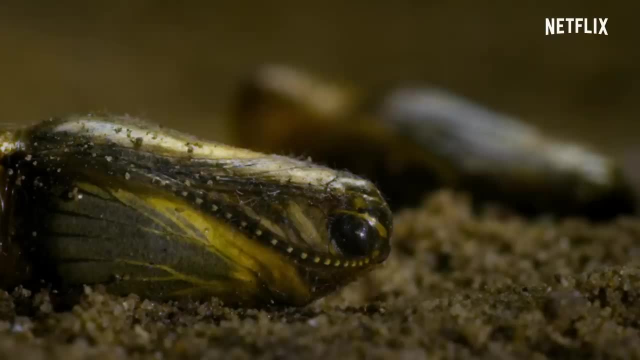 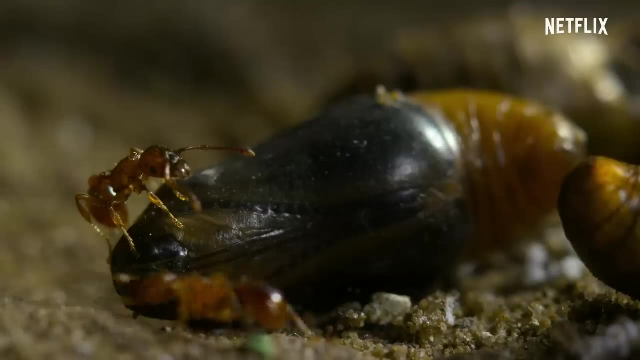 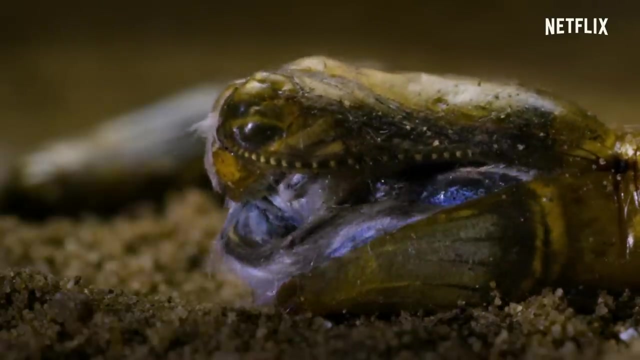 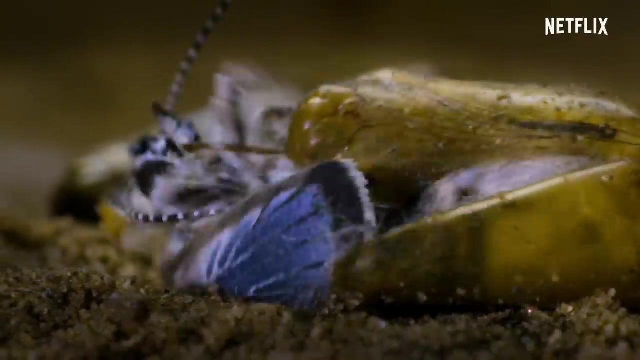 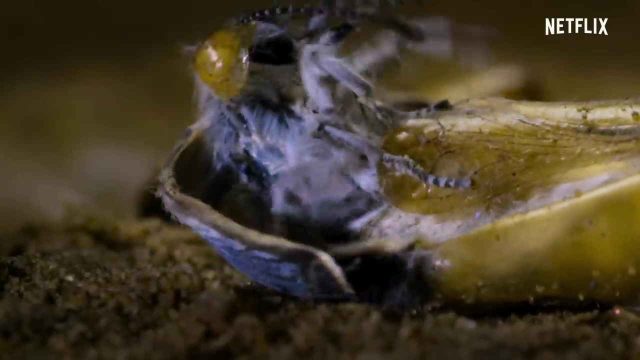 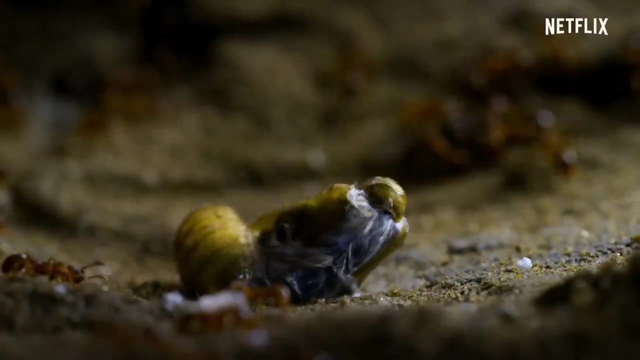 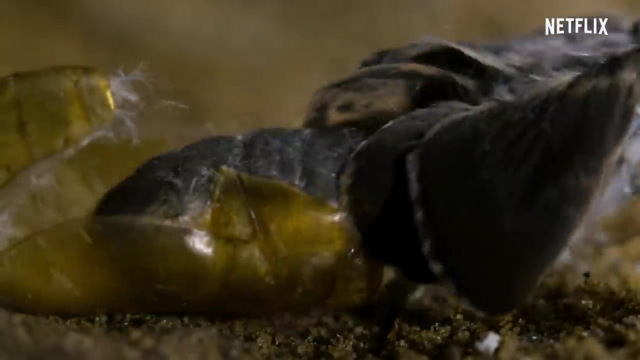 Until one day there is nothing for the ants to feed. The caterpillars have pupated, But a few weeks later out crawls an alcon-blue butterfly. Now they begin to leave the nest that has been their home for the last twenty-three months. 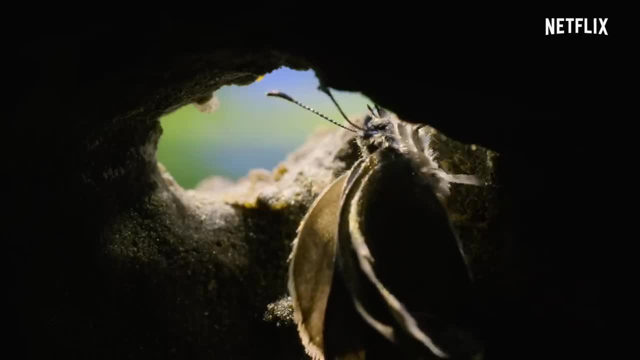 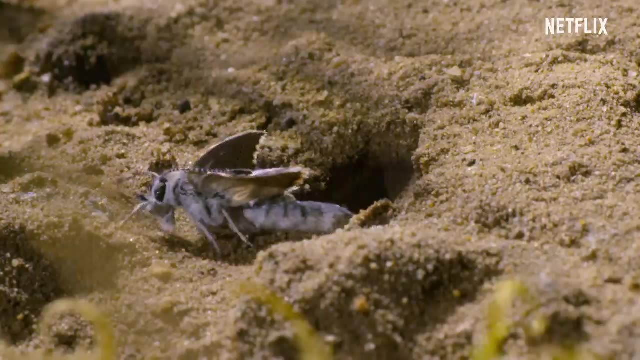 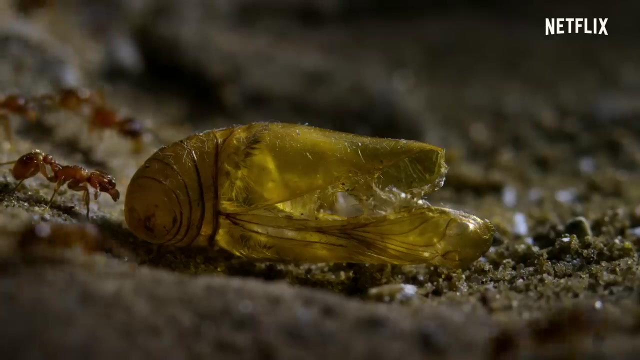 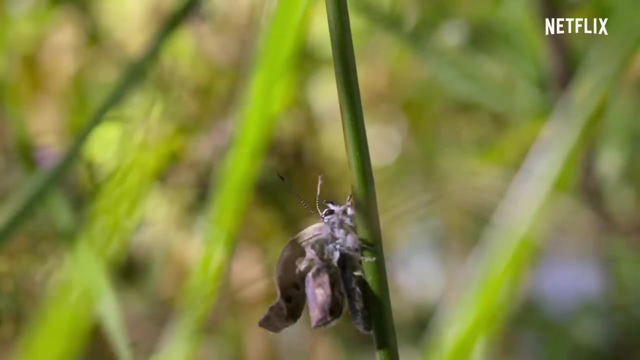 Now they begin to leave the nest that has been their home for the last twenty-three months. Now they begin to leave the nest that has been their home for the last twenty-three months. The young adult makes its way out of the nest and clambers up a grass stem. 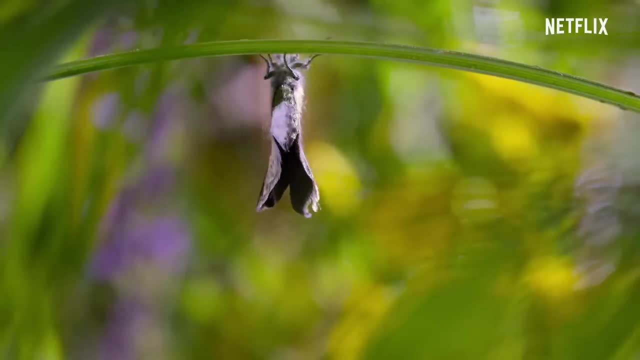 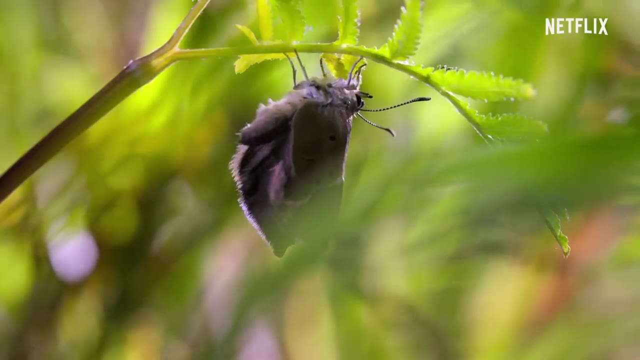 Its wings expand as it prepares to fly off and find a mate. Its wings expand as it prepares to fly off and find a mate. This complex life may be labour-saving for the butterfly, but it's risky. This complex life may be labour-saving for the butterfly, but it's risky. 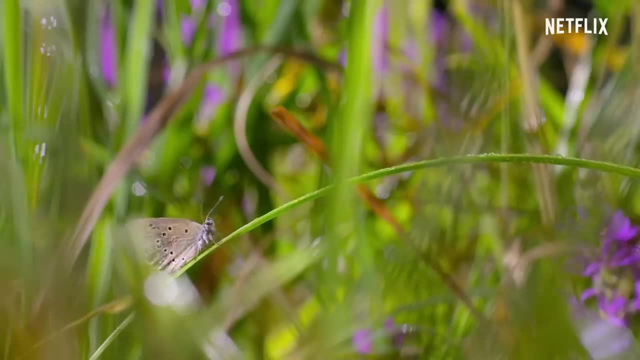 This complex life may be labour-saving for the butterfly, but it's risky. If anything happened to the ants or to the gentian, the alcon-blue would become extinct. If anything happened to the ants or to the gentian, the alcon-blue would become extinct. 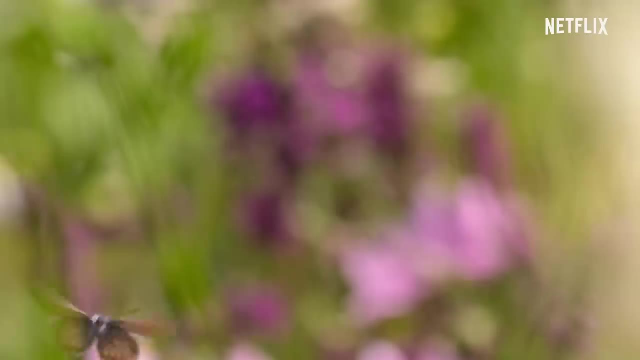 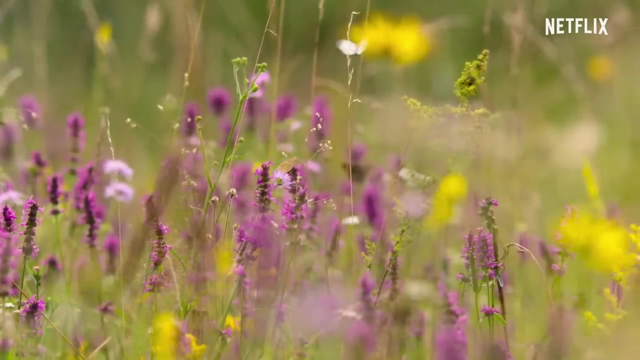 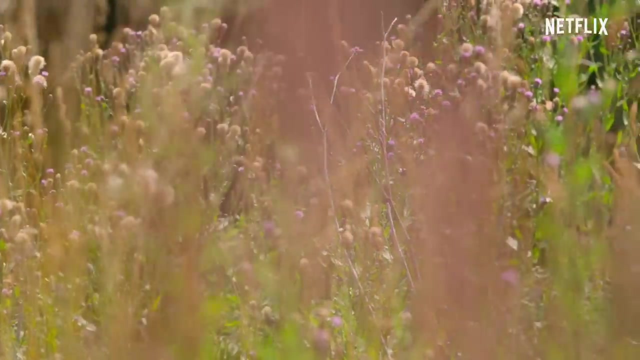 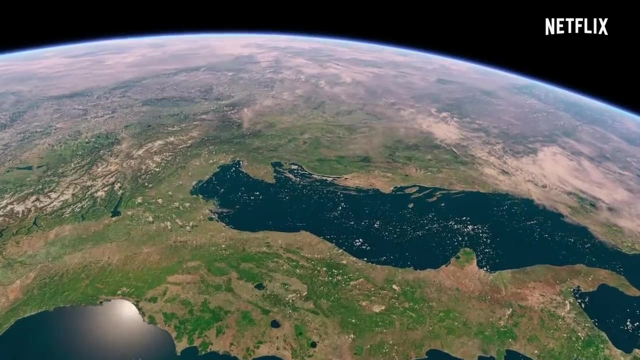 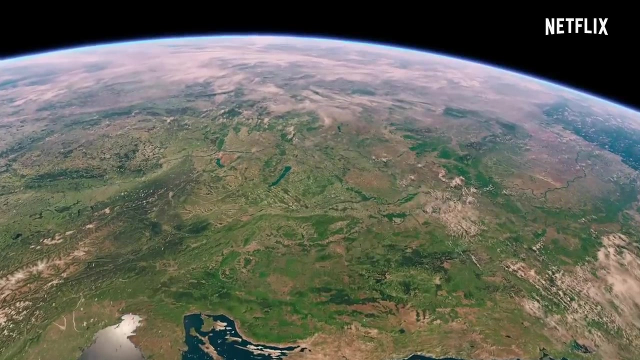 If anything happened to the ants or to the gentian, the alcon-blue would become extinct. Only tiny fragments of these ancient meadows are left in Europe, But beyond them, to the east, once stretched grasslands that extended for a fifth of the way around the world. 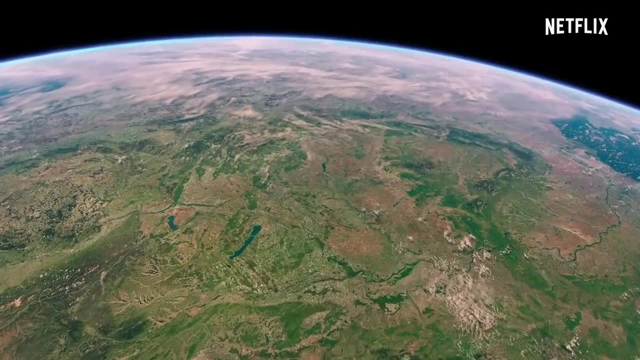 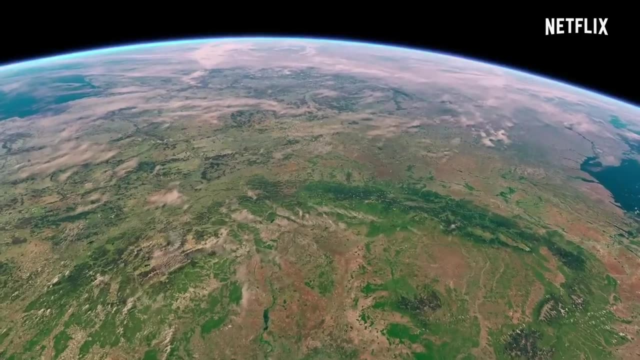 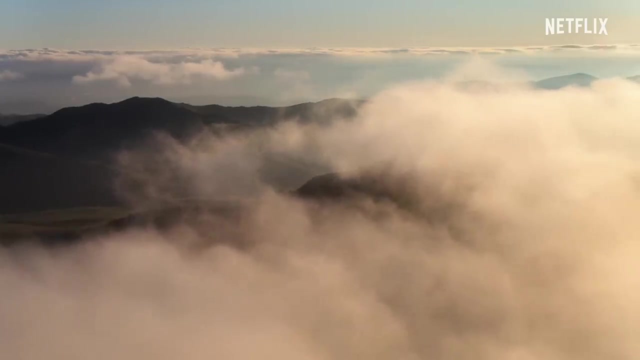 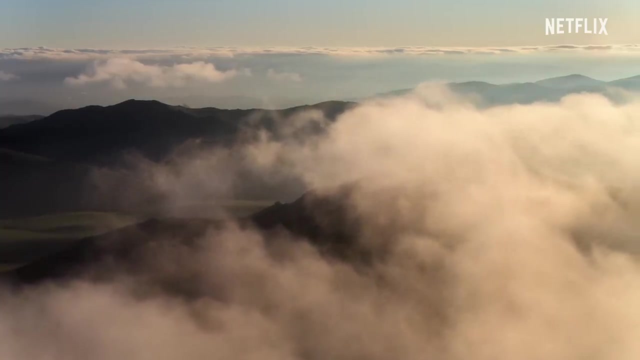 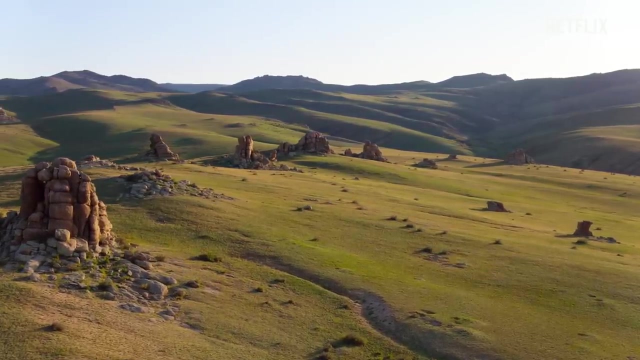 from Romania to China. Here there are places where, for mile after endless mile, there are no roads or fences. Here, where there are no trees, eagles and no birds. there are no trees, eagles and no birds. 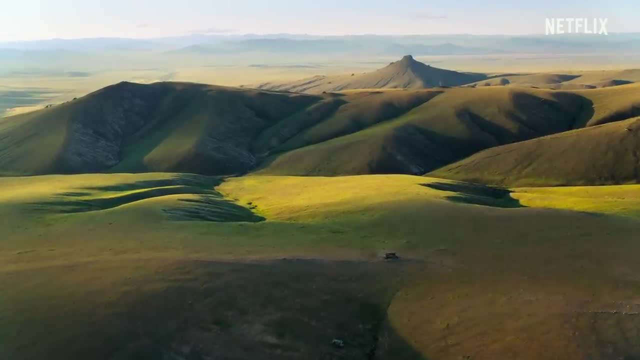 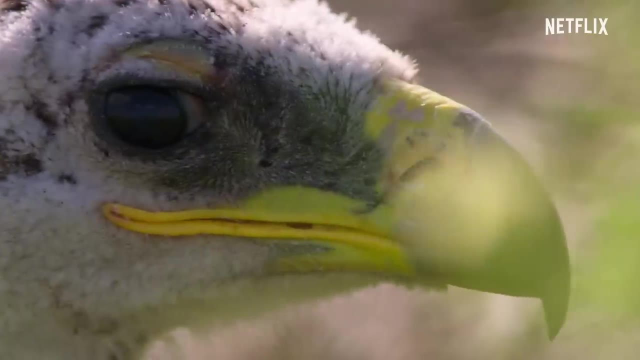 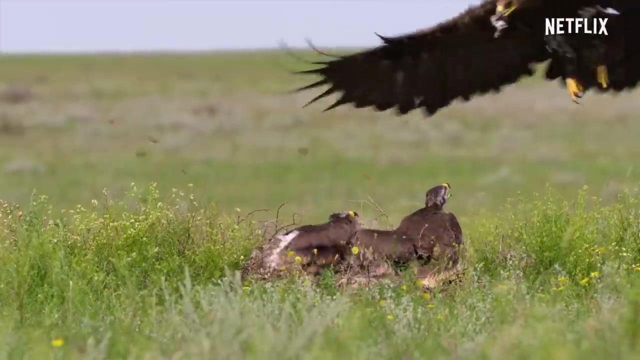 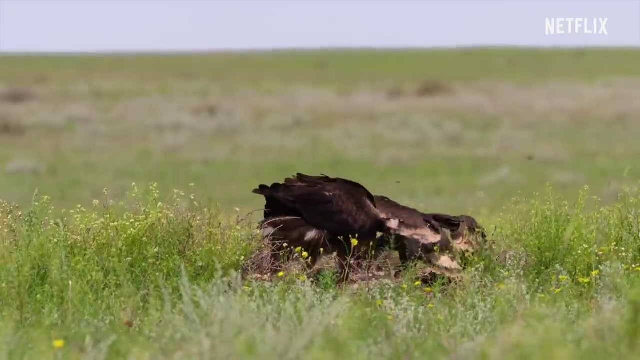 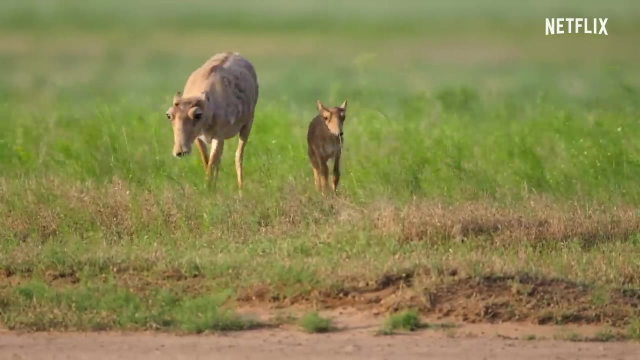 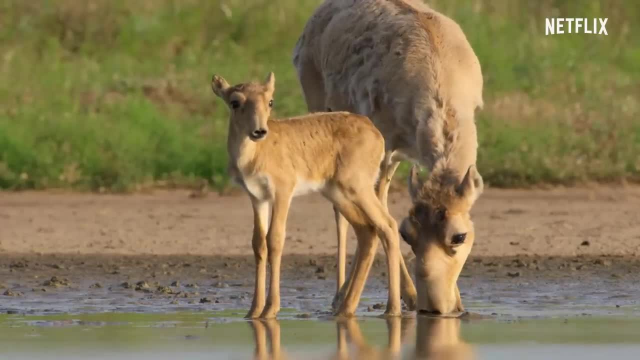 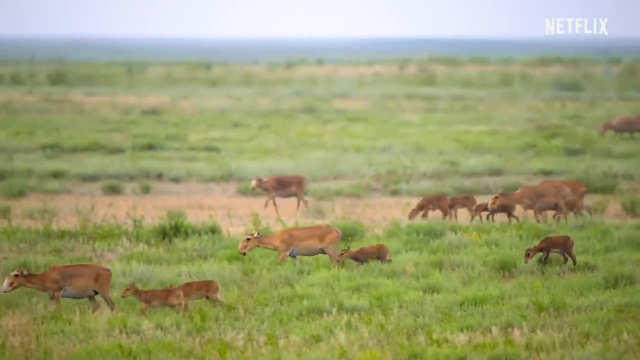 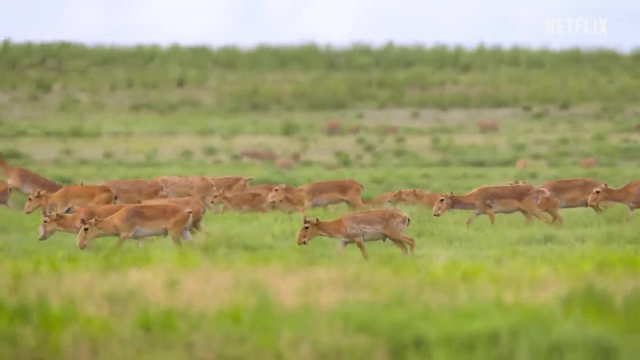 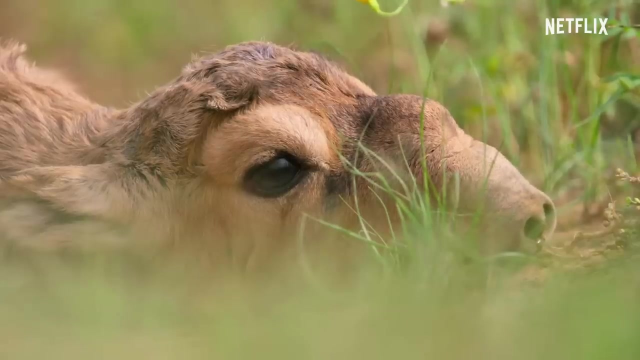 Their extraordinary noses are specially adapted to filter out the dust kicked up by the immense herds that once lived here. Now they're critically endangered. Poaching and the loss of habitat have had a devastating impact on them, But conservation efforts have recently started to make a difference. 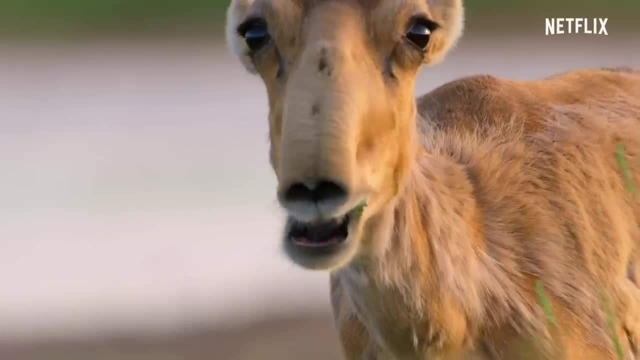 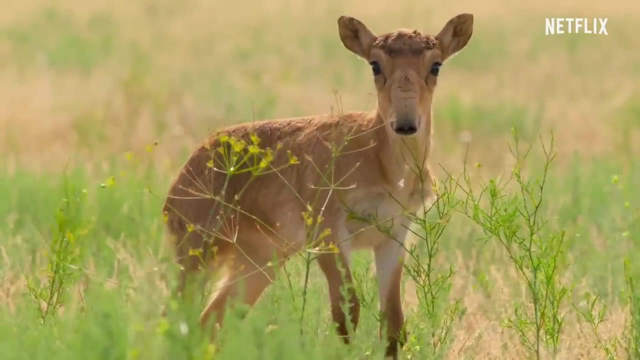 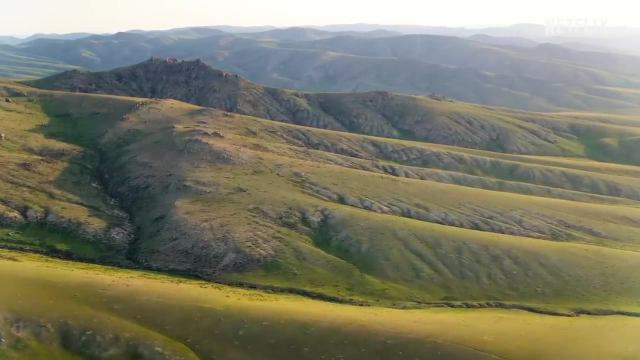 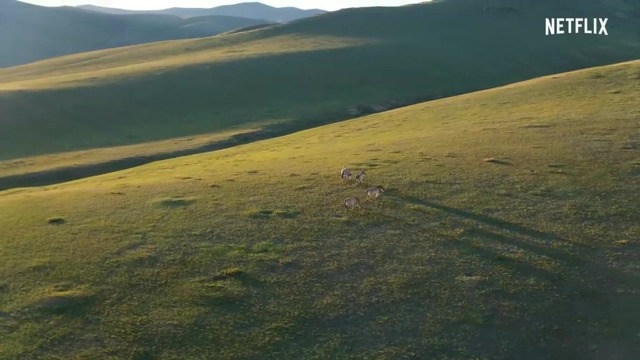 There is still hope for these extraordinary plains dwellers, And the proof of this can be found further east, in Mongolia, where the grasslands still remain largely intact. The grasslands are still in good condition, but they are still in poor condition. 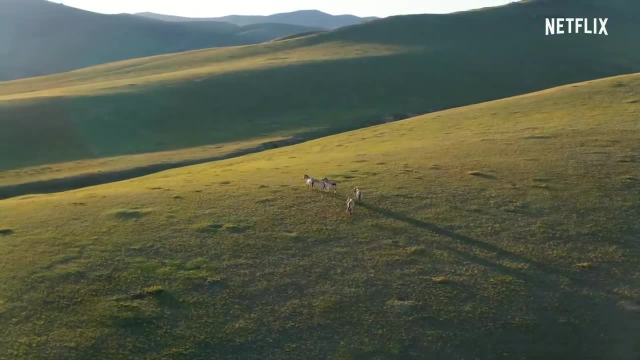 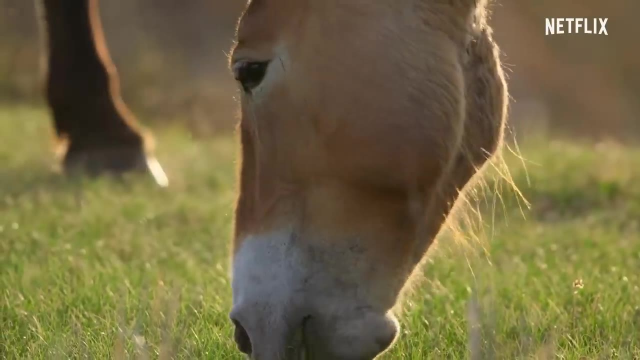 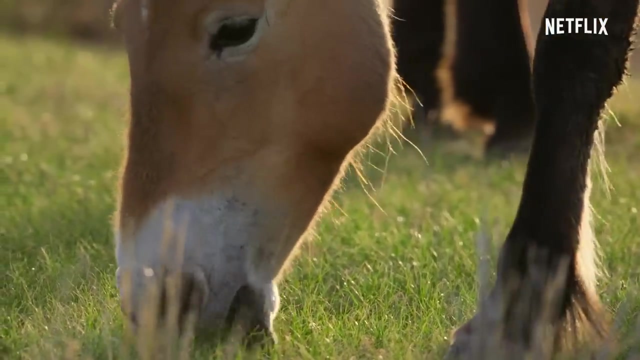 The grasslands are still in poor condition, but they are still in poor condition. They are Shuvalsky's horses. Fifty years ago they were extinct in the wild, But a few adults survived in captivity. Careful breeding from 12 of them increased their numbers. 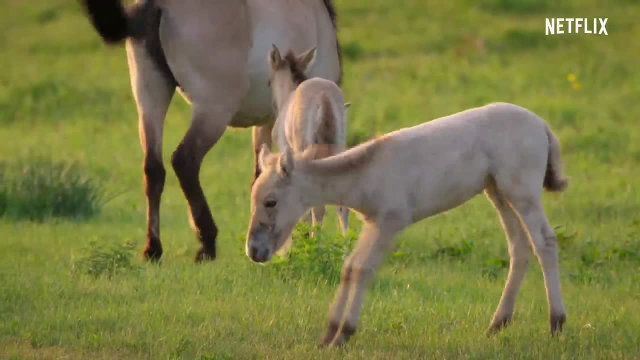 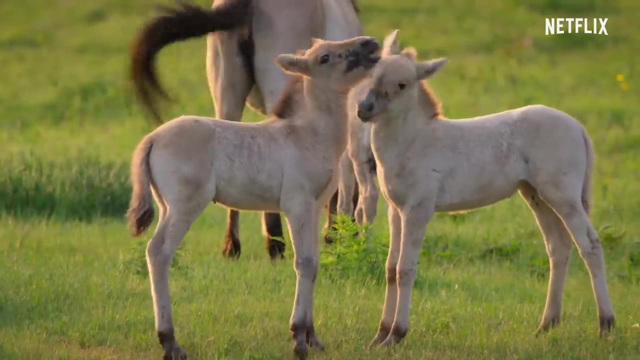 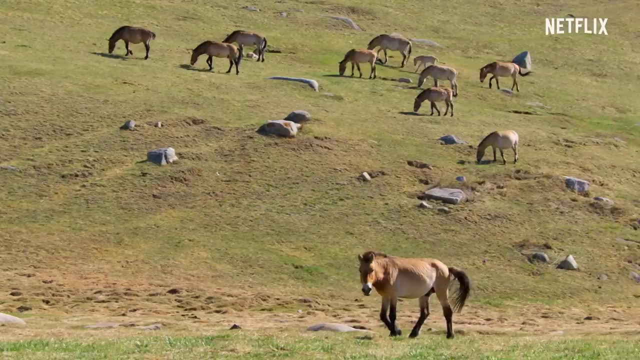 until there were sufficient to release on the plains. These are their descendants. They gave birth to a good family. They have many children. The young are already helping their mothers and children. The older are feeding their children. These people are not just coming to get food. 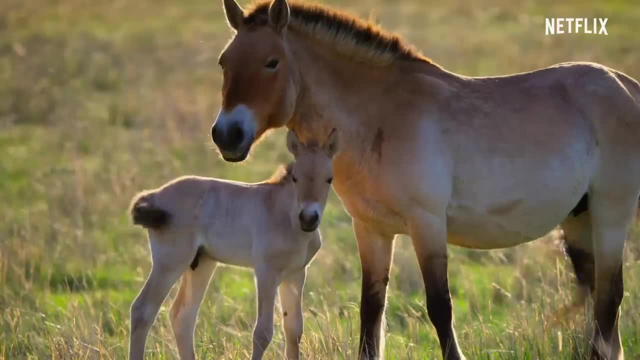 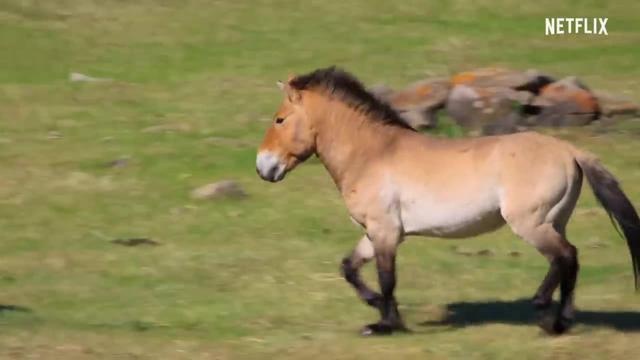 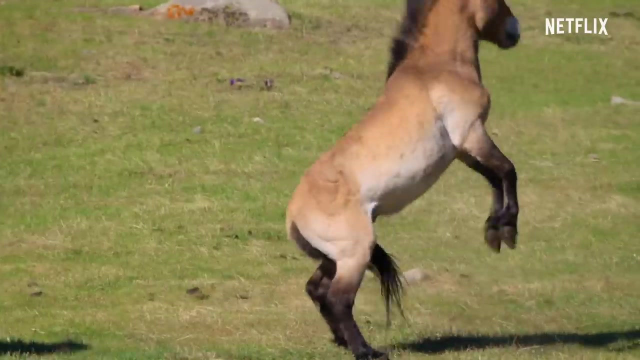 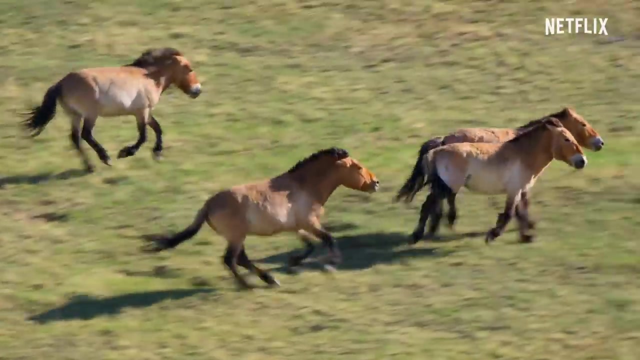 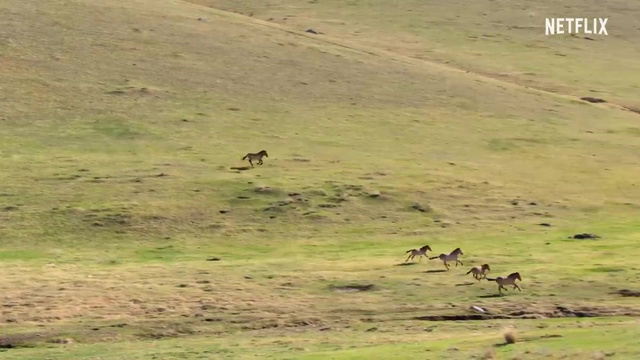 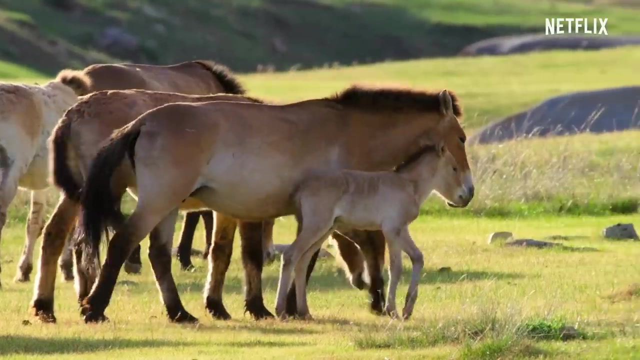 so they must also look after the poor. A stallion protects each harem. They must be vigilant and they race to defend their herd, Faced off bachelors trying to lure away a mare, With their numbers now topping 300,. 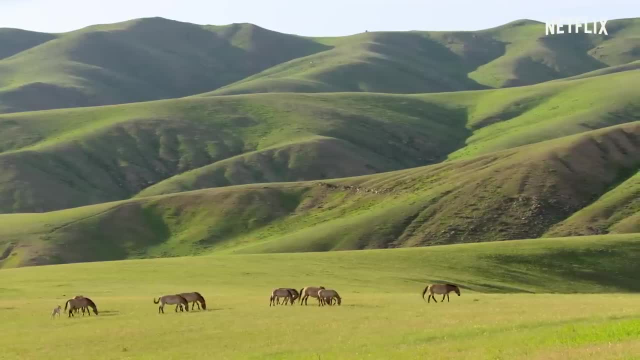 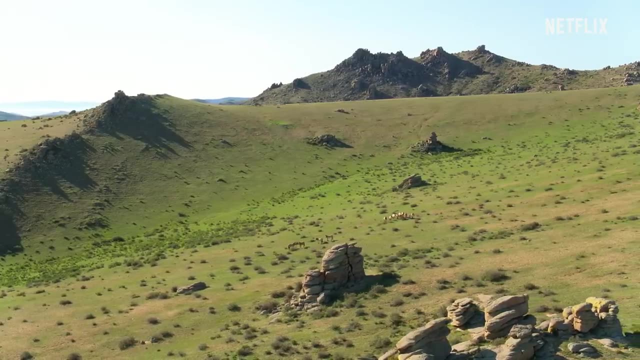 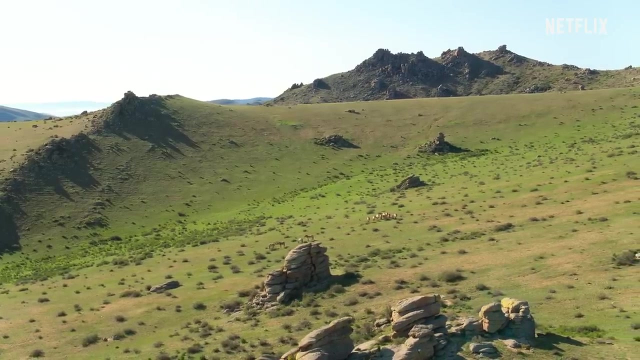 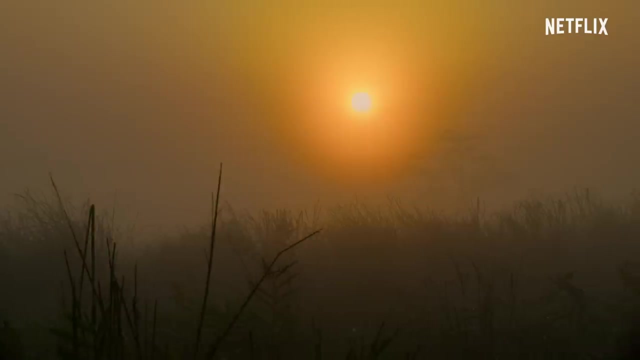 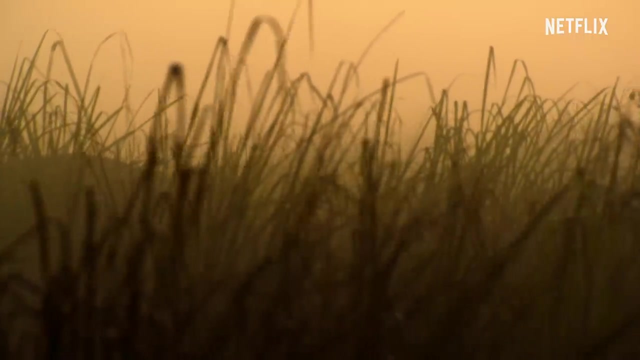 the future for these wild horses looks more secure. Their recovery was only possible because the vast Mongolian steppe still remains largely untouched. These grasses are some of the tallest to be found anywhere on our island, On our planet. They're so tall they can conceal elephants. 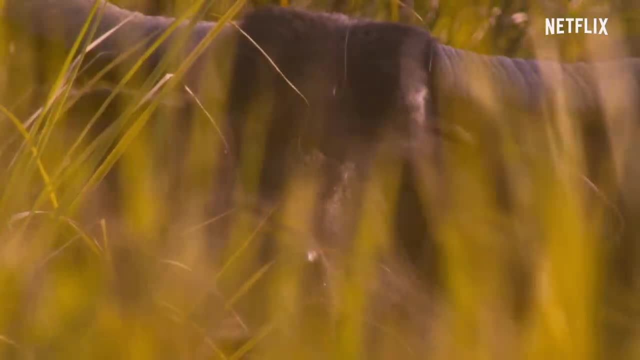 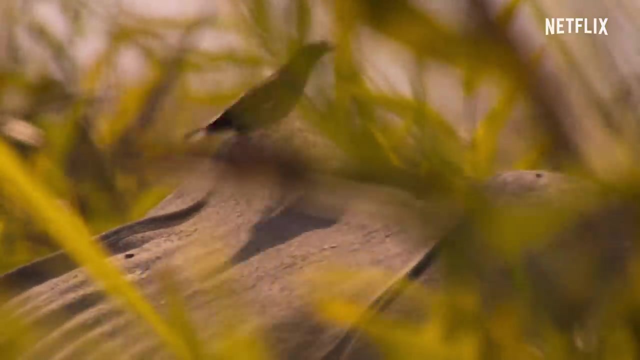 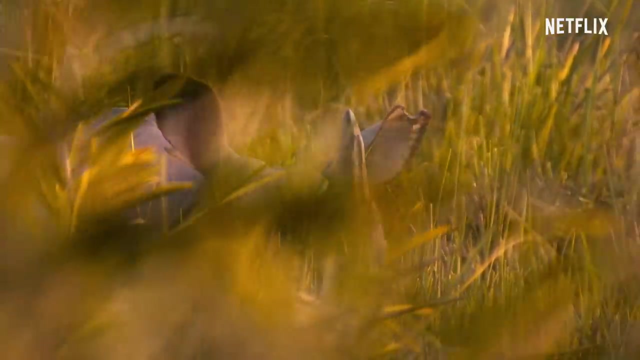 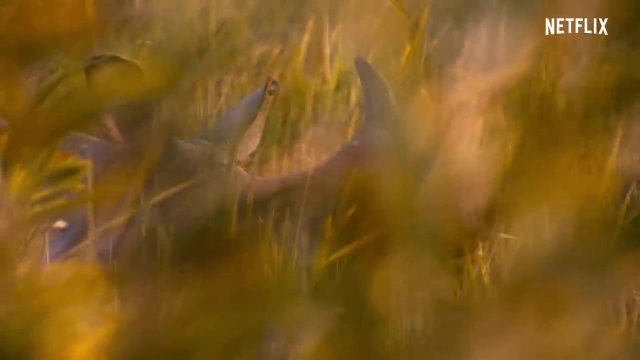 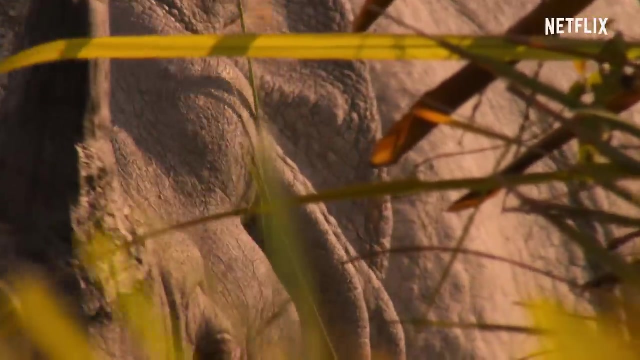 They make the giants that live among them seem small. They're also very well-trained. They're very well-trained. They're very well-trained. They're very well-trained. A last hiding place for the highly endangered greater one-horned rhino. 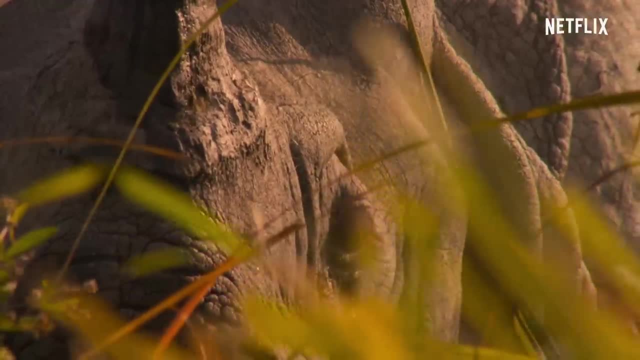 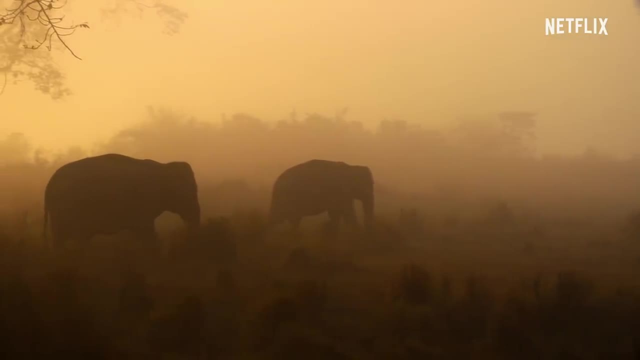 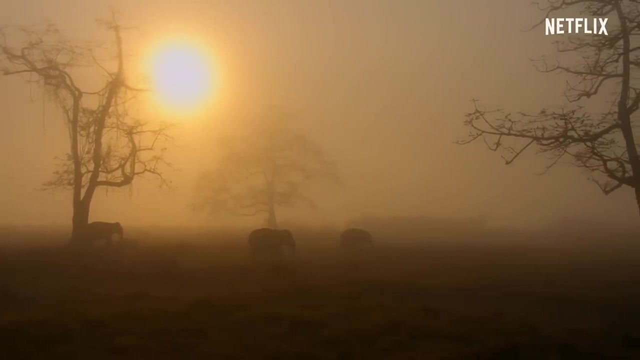 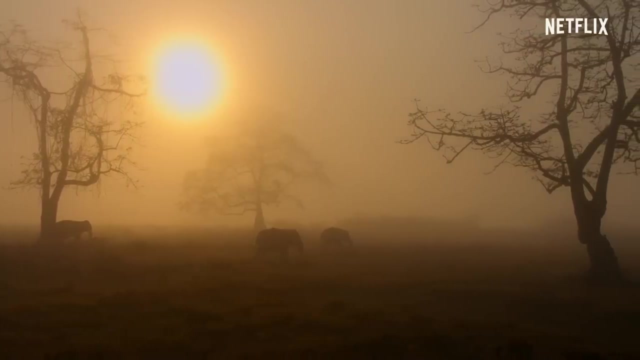 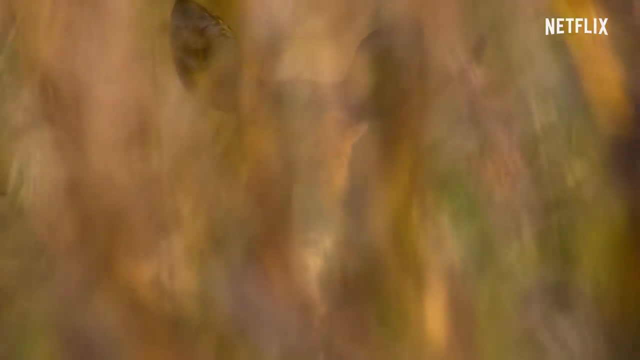 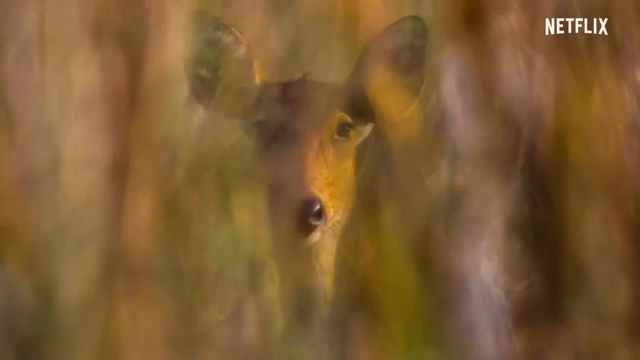 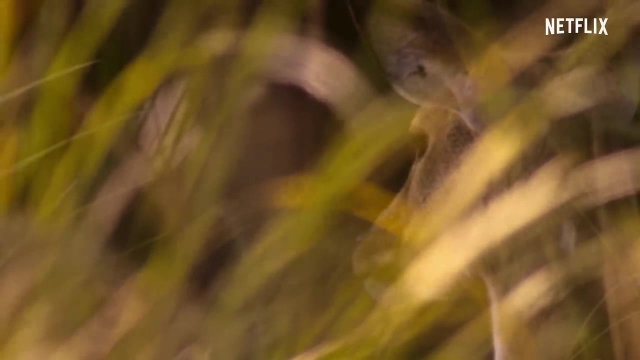 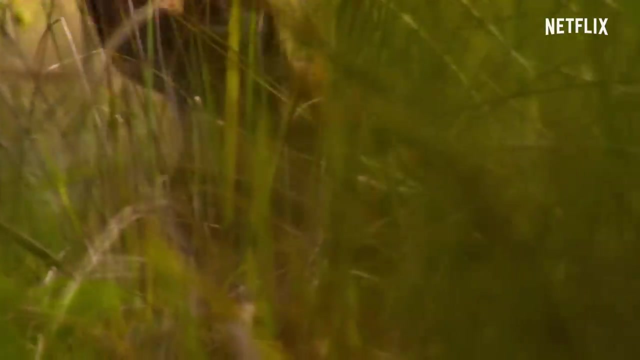 This is India, one of the most populous countries on Earth. Yet here there is a great determination to protect these crucial grasslands. What must it be like to live in this dense, claustrophobic world? Just moving about could mean walking into danger. 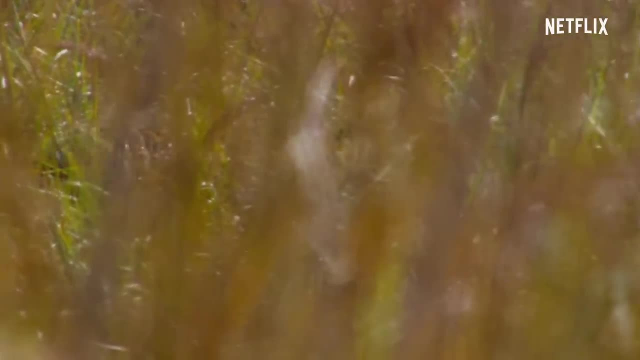 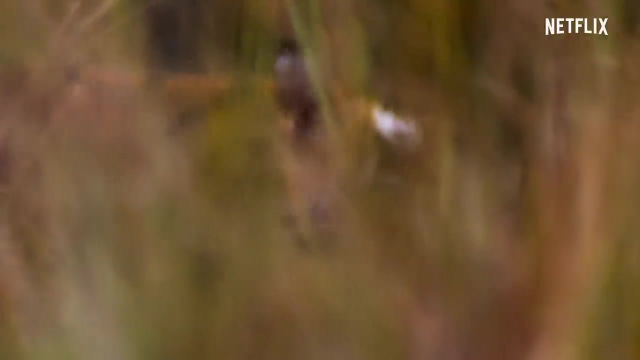 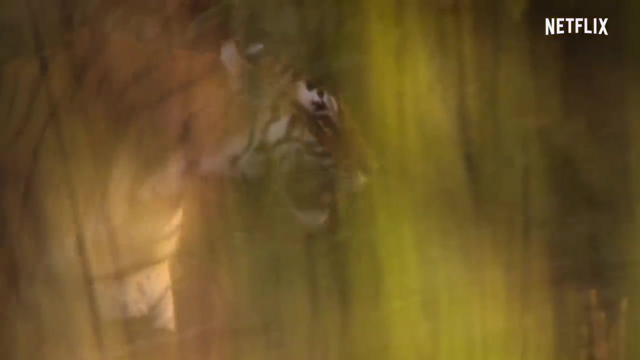 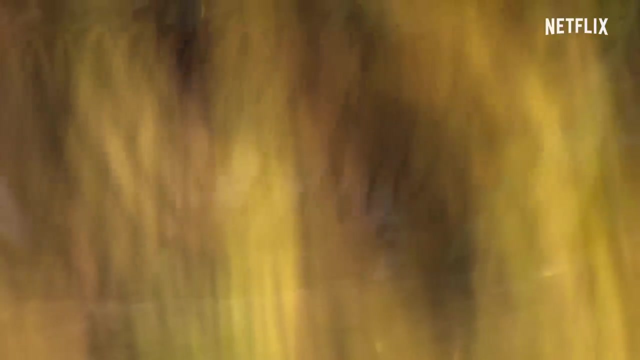 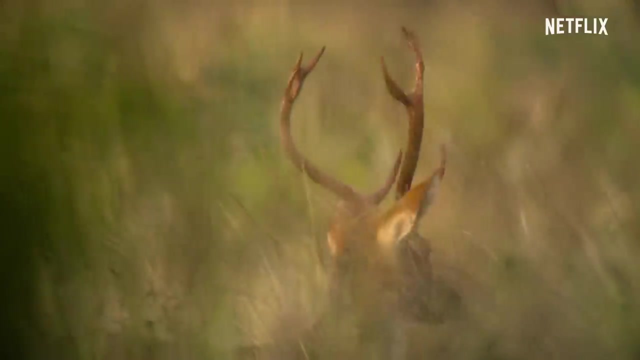 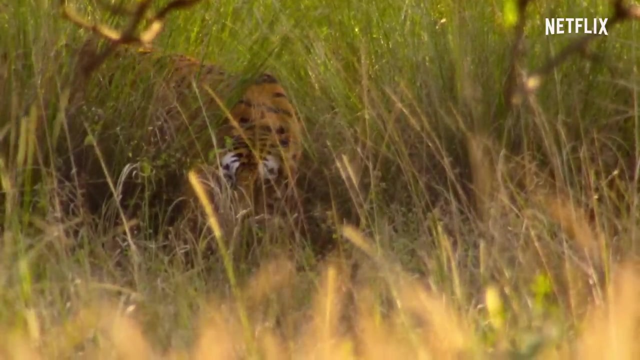 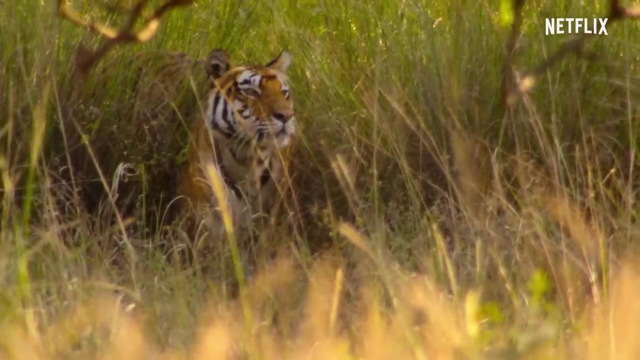 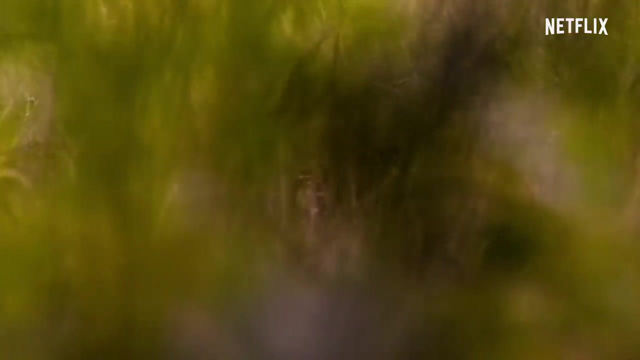 The grasses conceal tigers. Stripes and shadows Blend. Long grass may hide a tigress from her prey, But it also hides the prey from her And the tigress will enter the forest Within 20 metres of the forest. 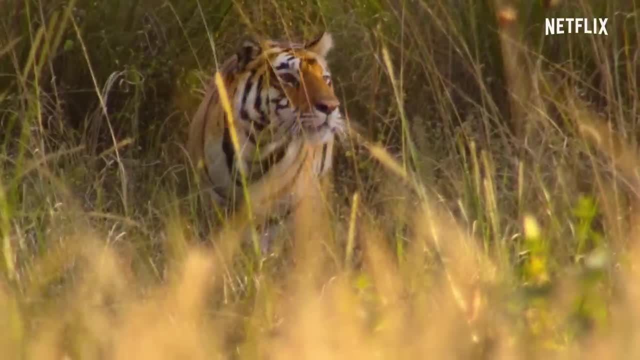 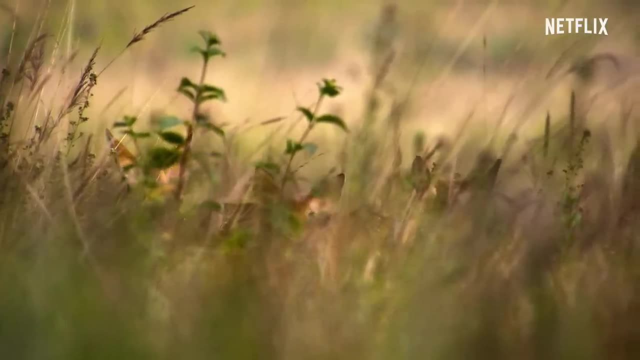 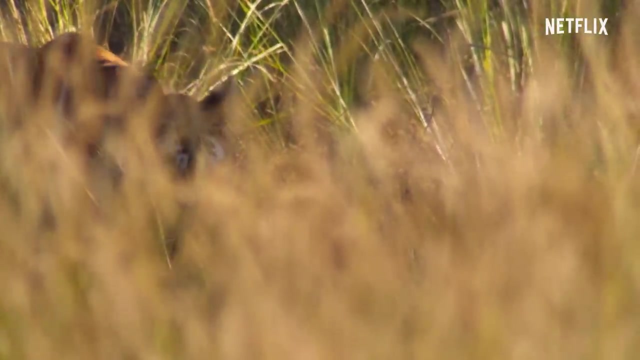 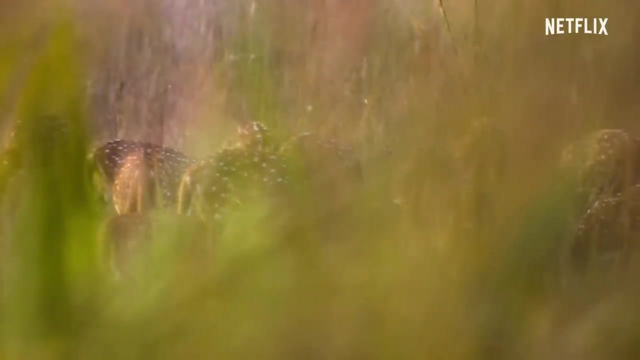 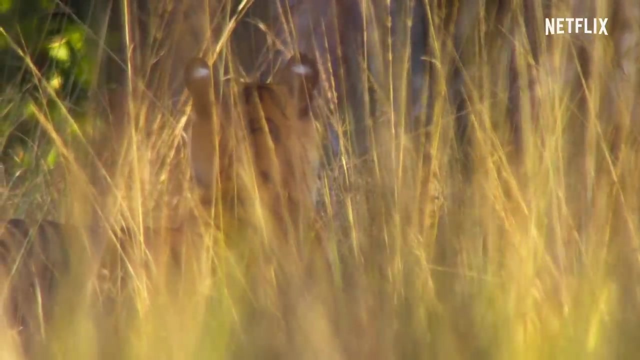 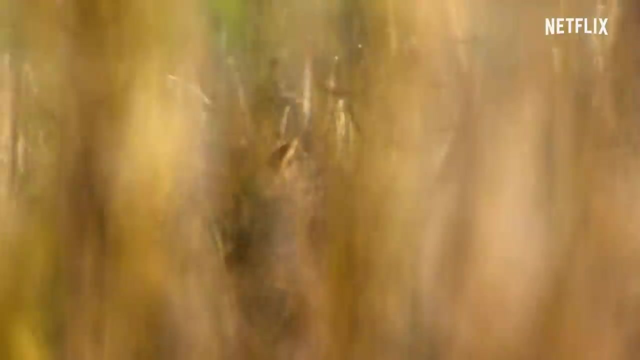 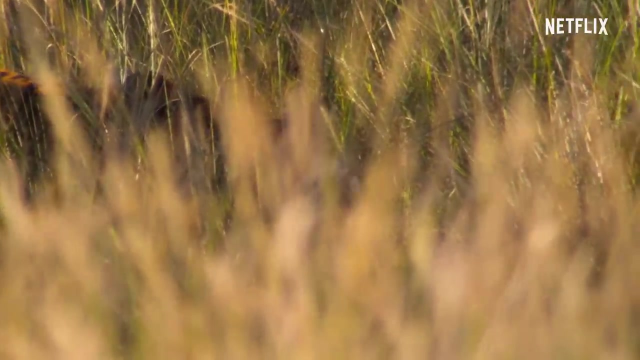 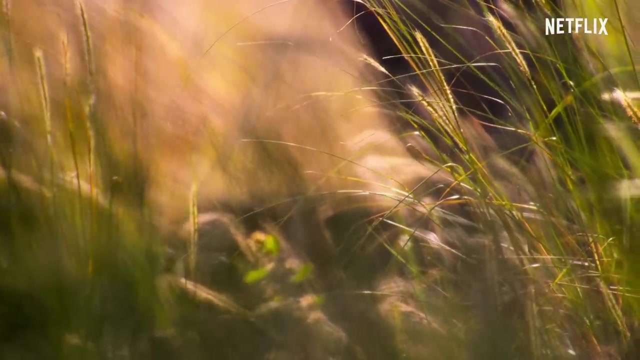 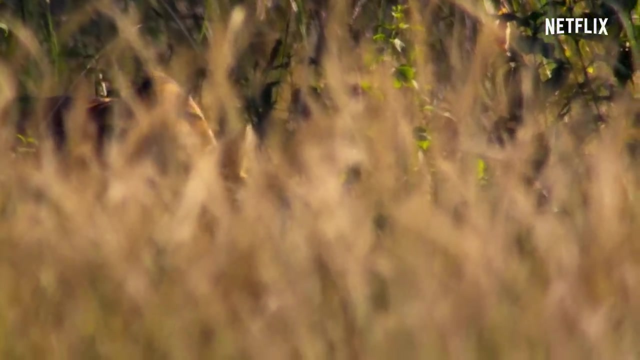 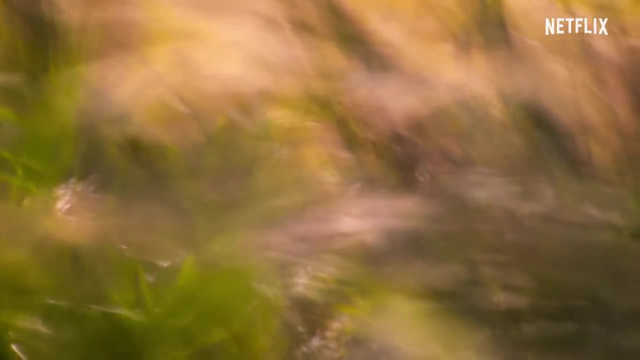 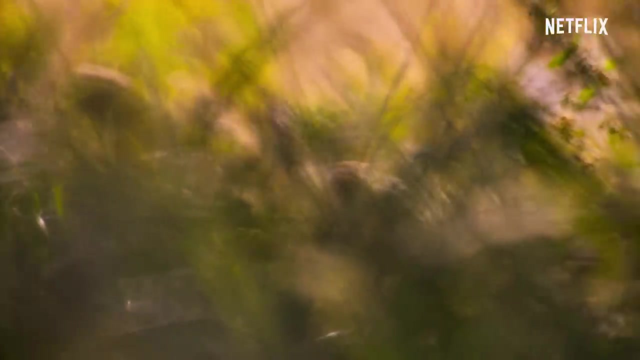 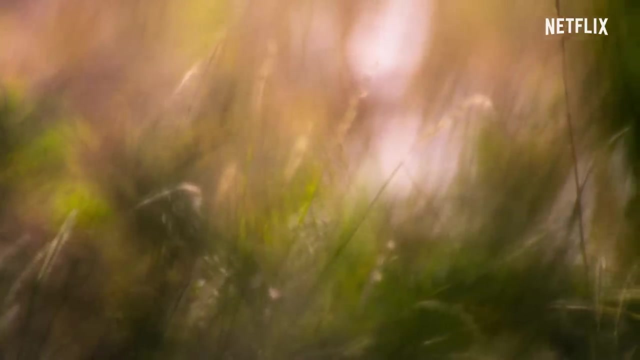 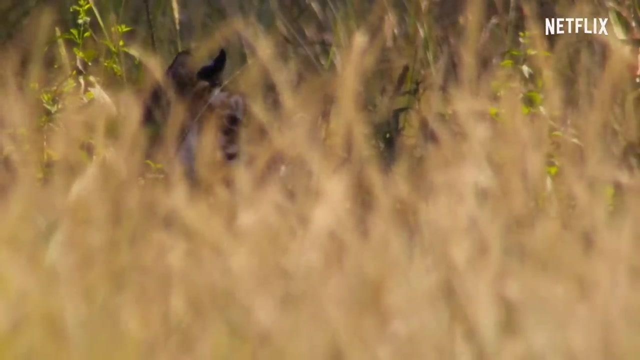 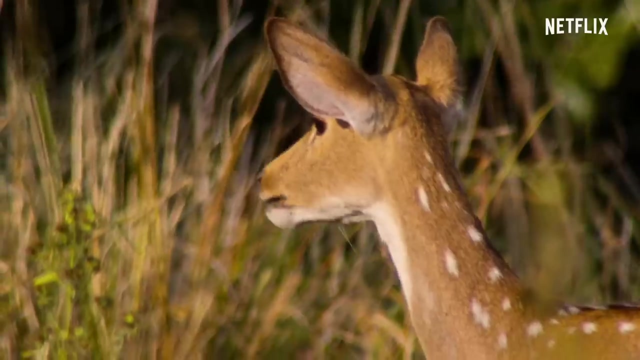 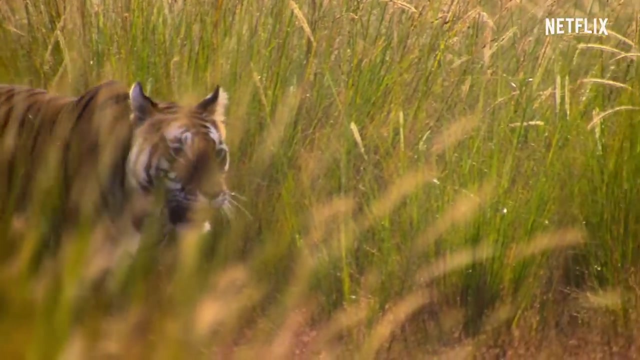 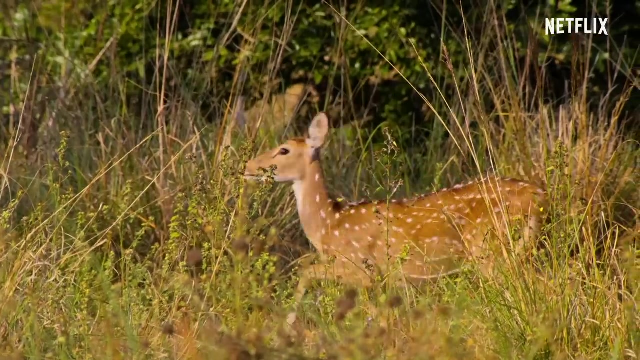 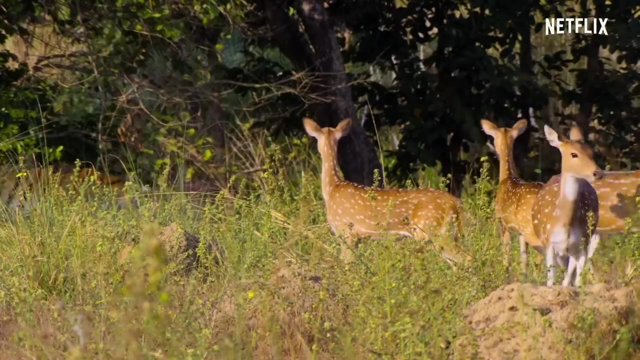 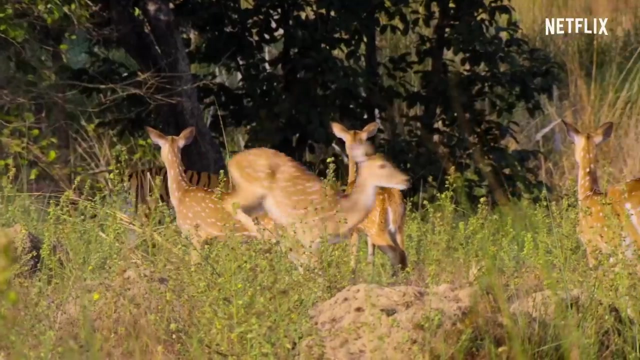 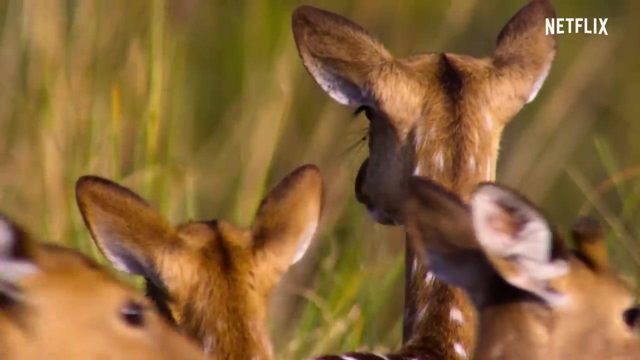 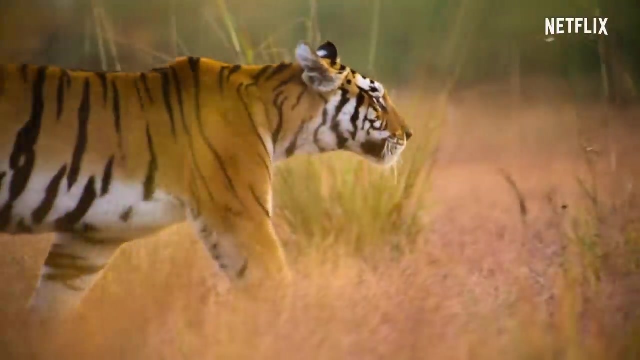 She must get within 20 metres of it And she must always know exactly where the prey are hidden. I love you. I love you, I love you. Every deer around now knows exactly where the tiger is. I love you. Others have heard. 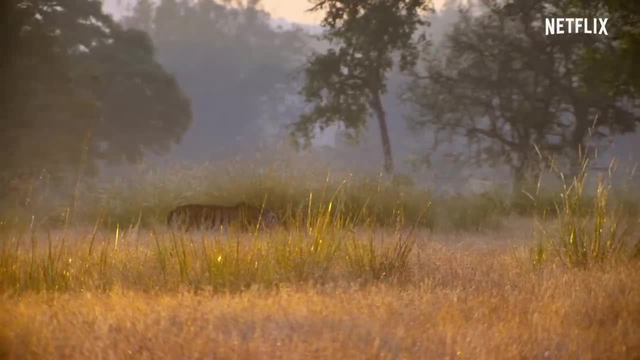 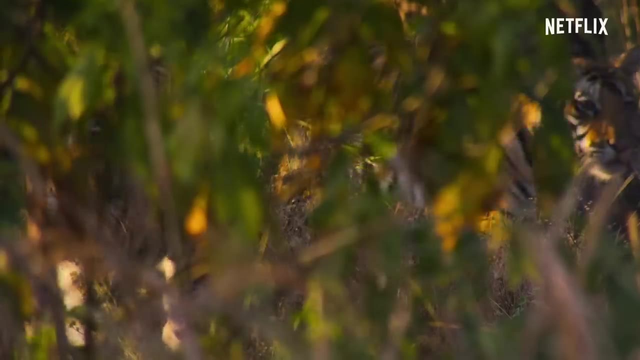 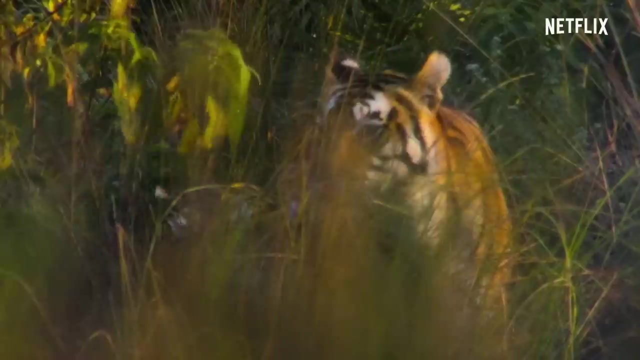 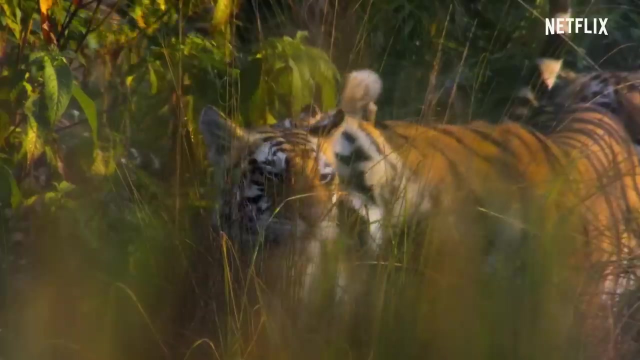 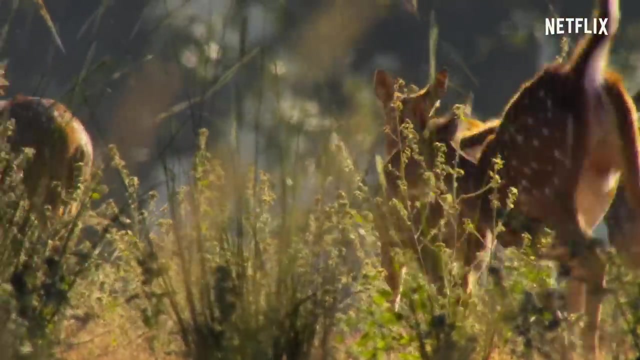 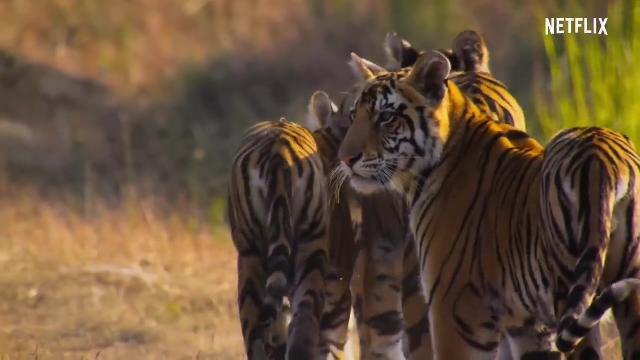 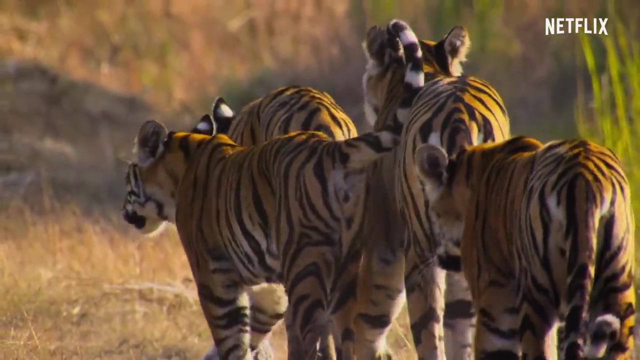 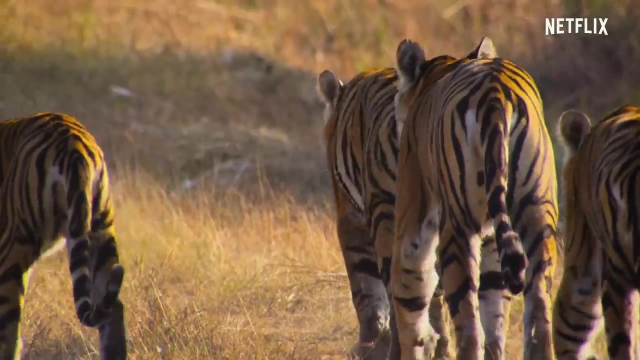 the signal that announced her failure: Her cubs. She had left them hidden in the grass. In the last hundred years, the number of wild tigers has declined by over 95%, But here in India, despite the enormous pressure from poaching and a growing 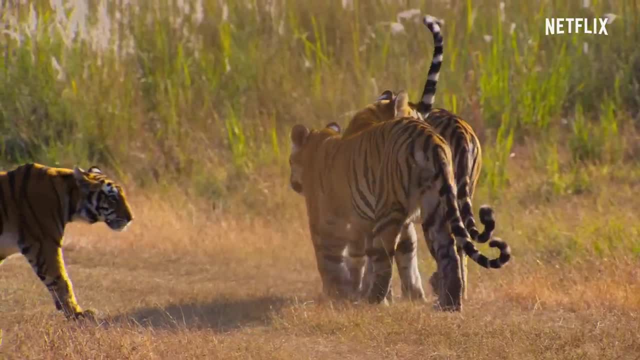 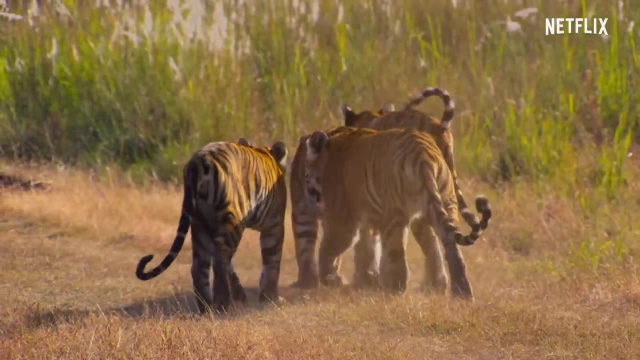 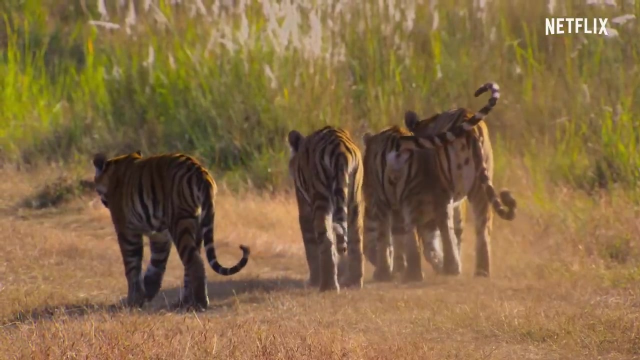 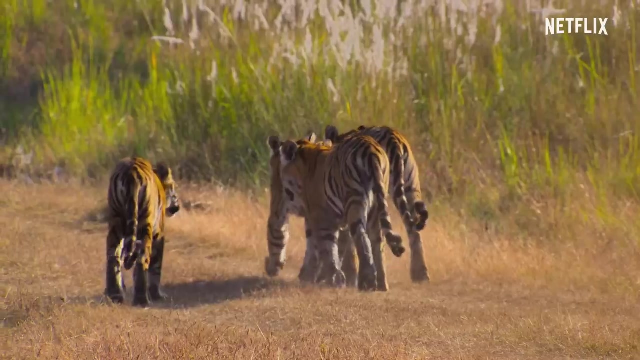 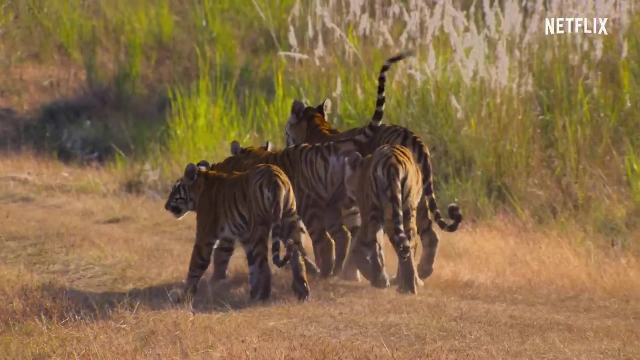 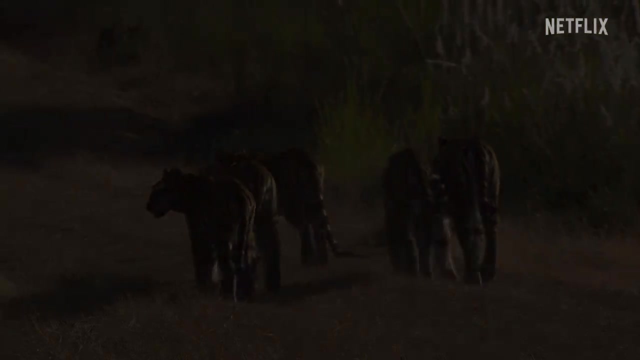 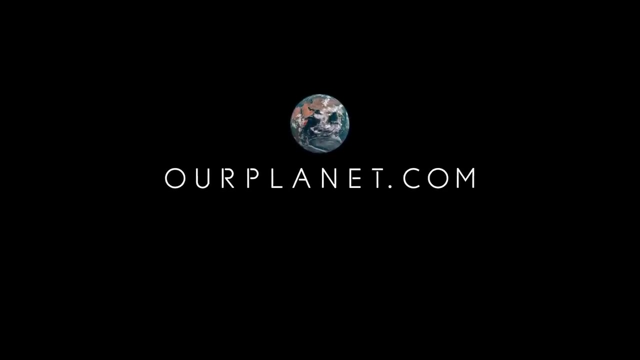 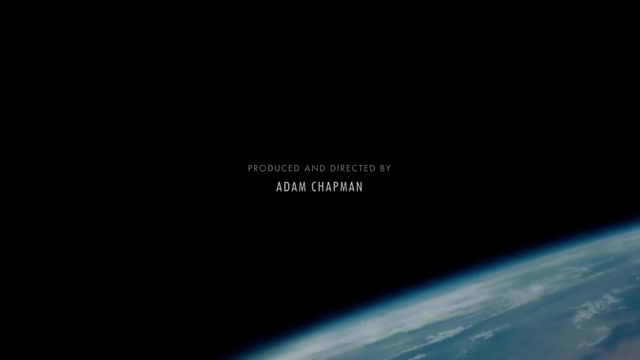 human population. tiger numbers are actually increasing. Protect the precious space that grasslands and deserts provide, and the animals will bounce back Our home. Please visit ourplanetcom to discover what we need to do now to protect wild grasslands. I can hear the whole world. 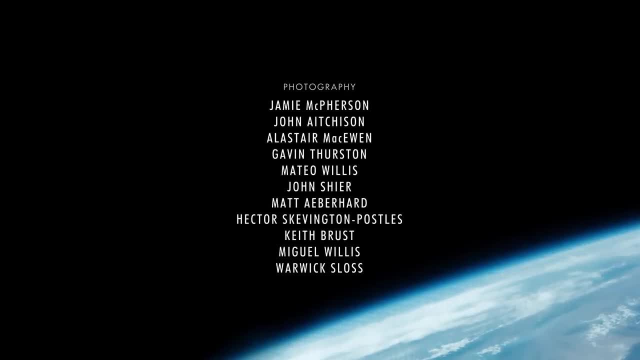 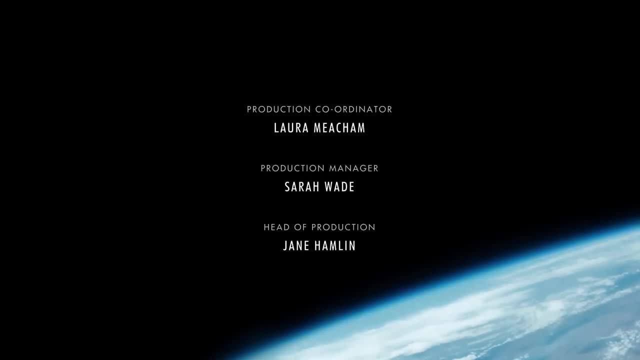 singing together, together. I can hear the whole world singing together, together, together. I can hear the whole world singing together, together, together. I can hear the whole world say it's now or never, Cause it's not too late if we change our ways. 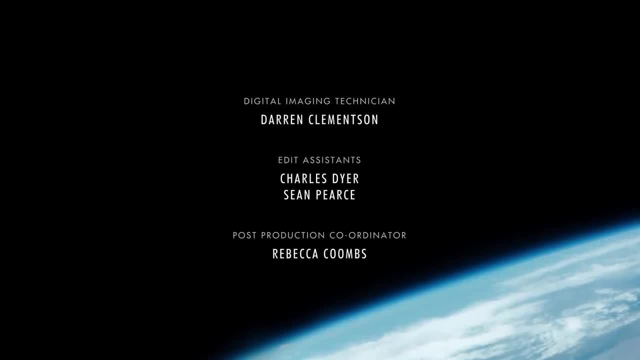 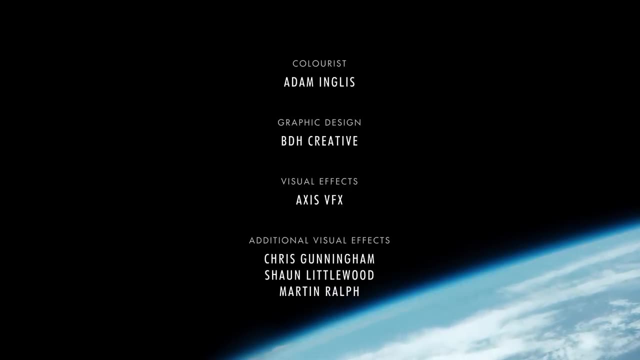 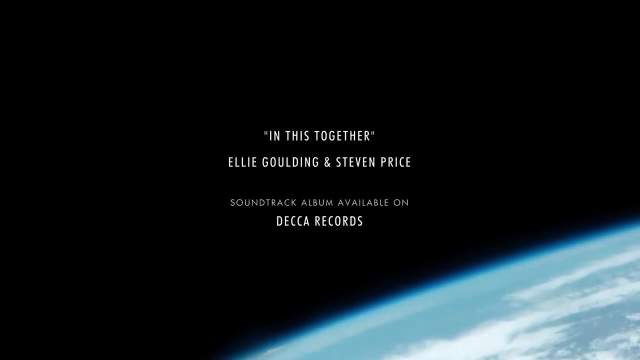 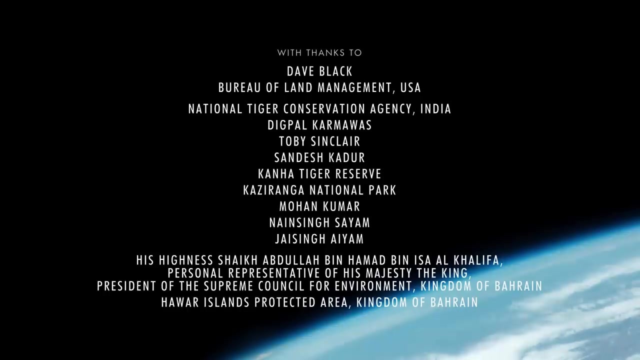 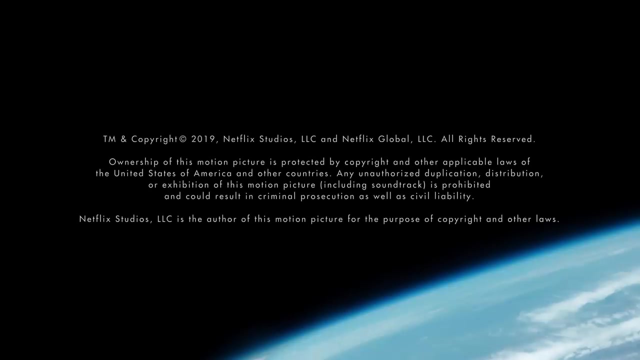 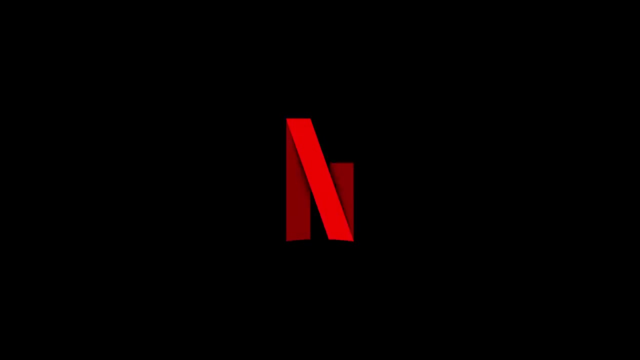